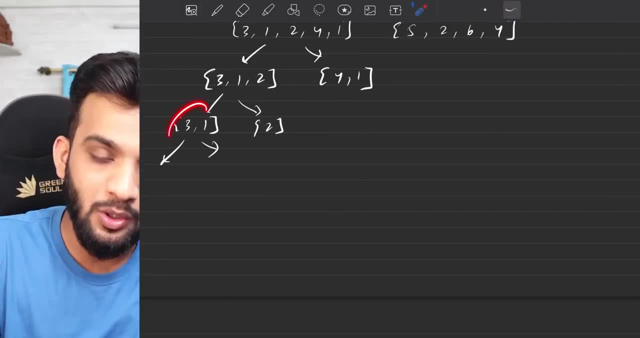 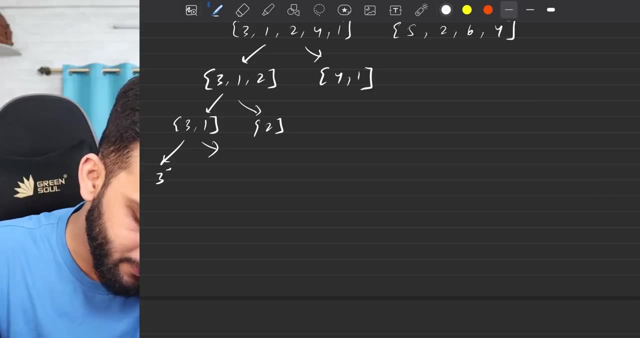 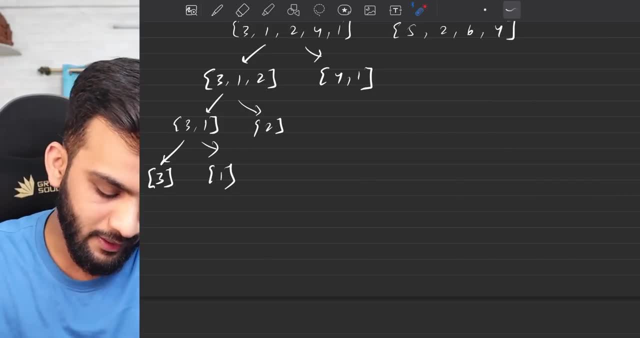 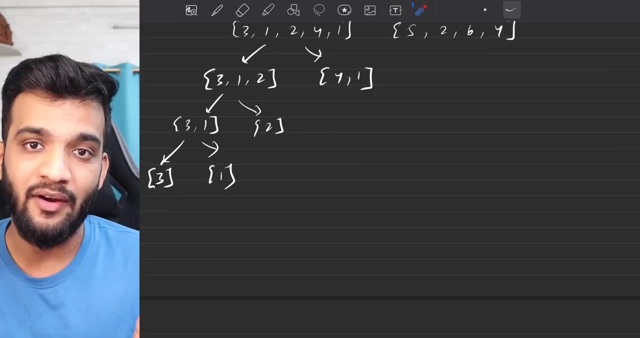 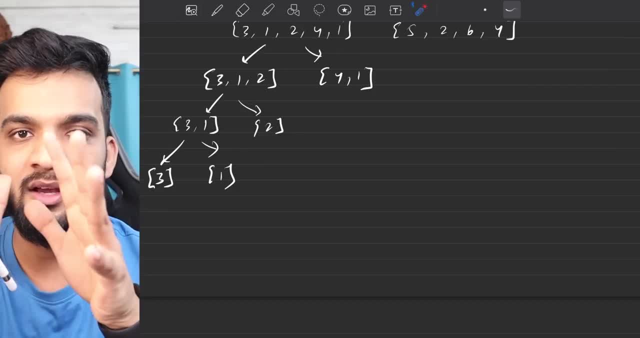 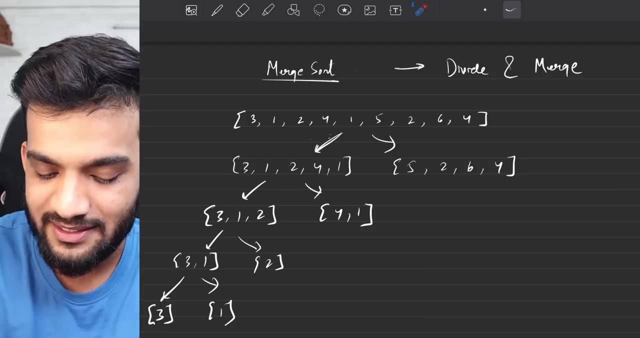 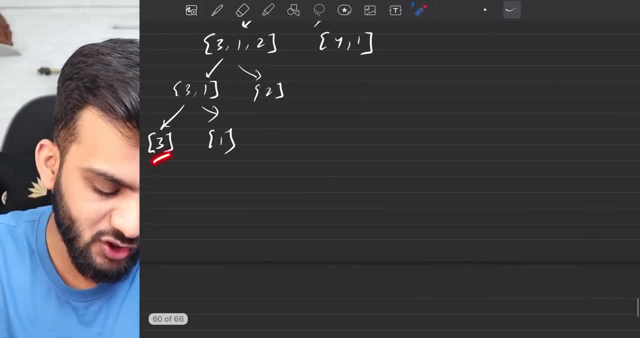 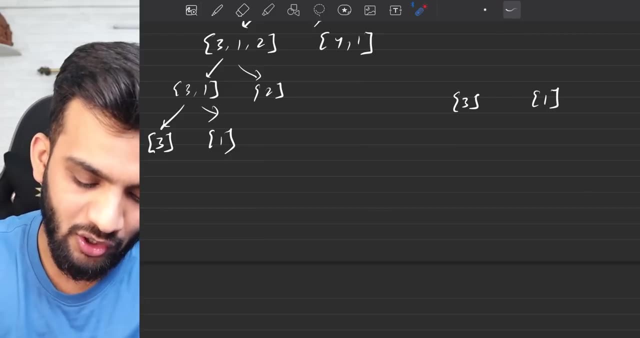 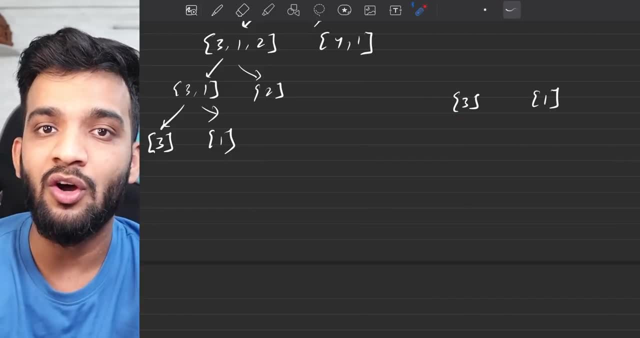 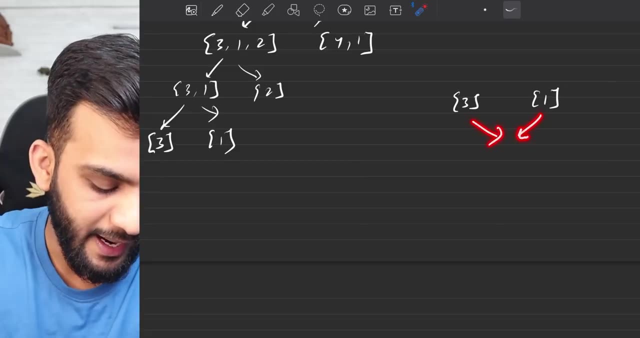 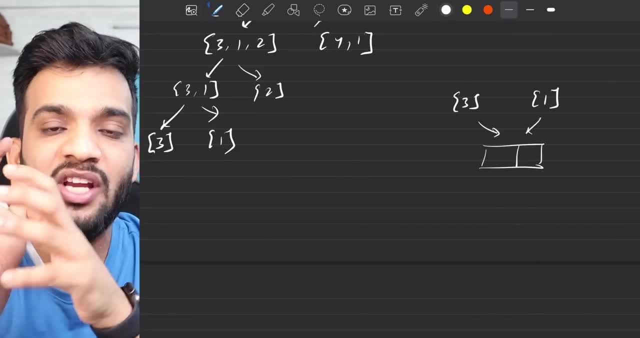 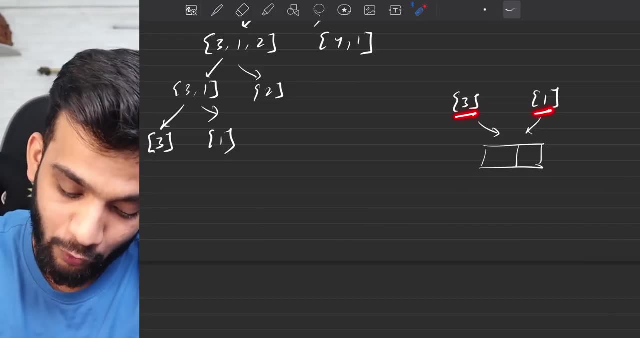 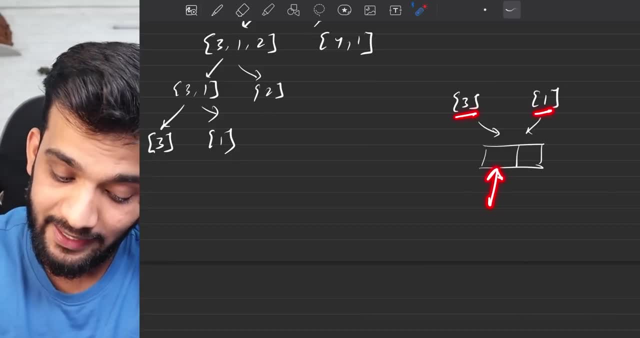 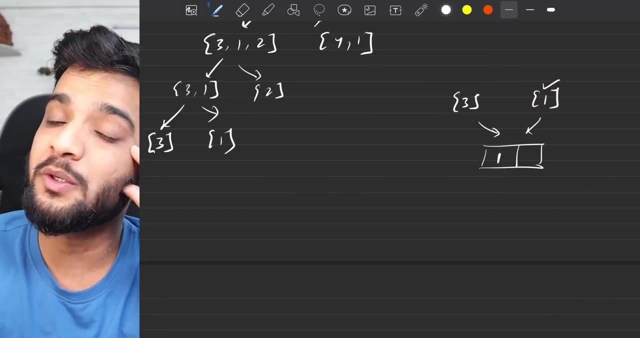 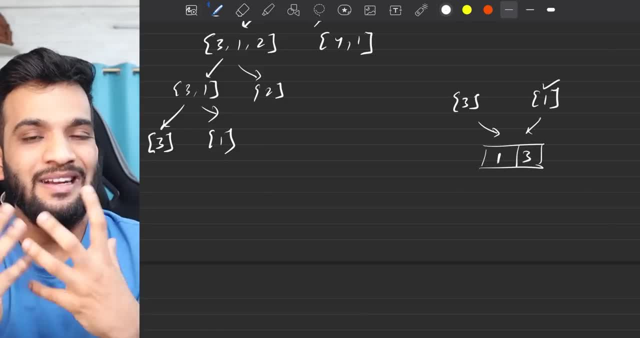 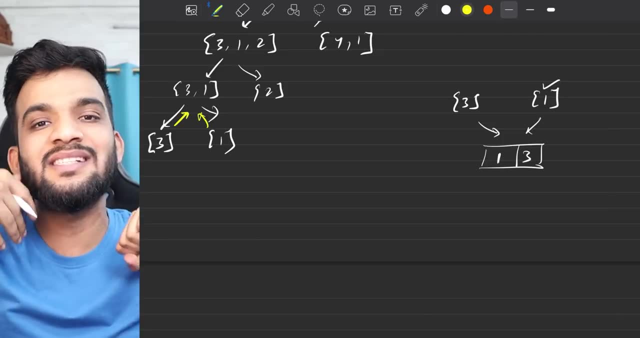 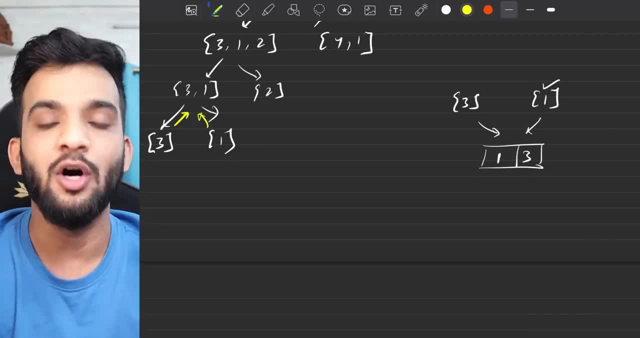 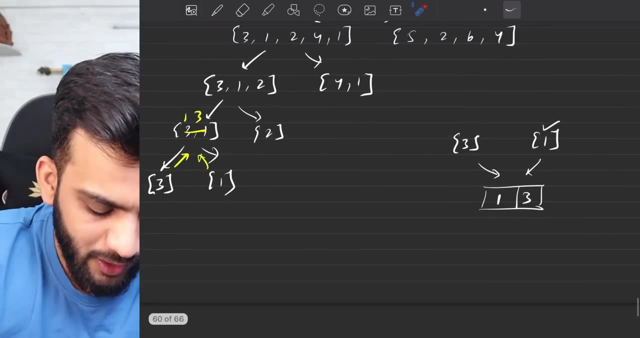 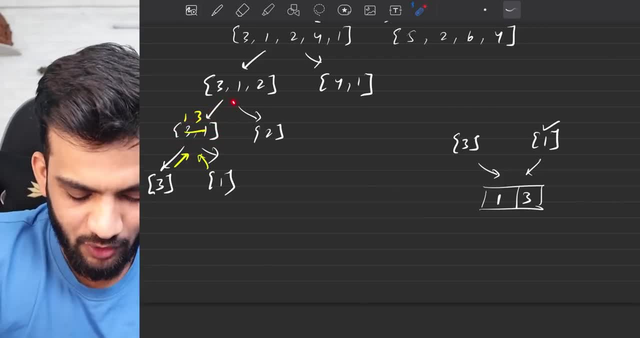 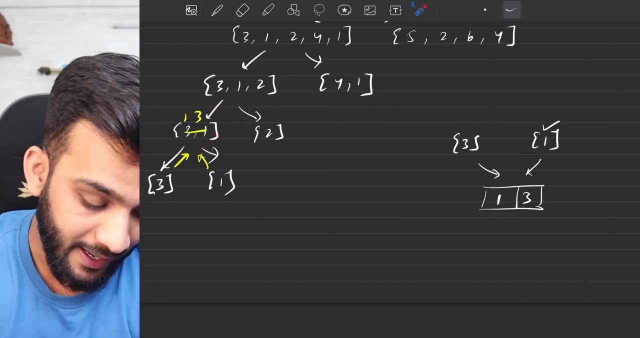 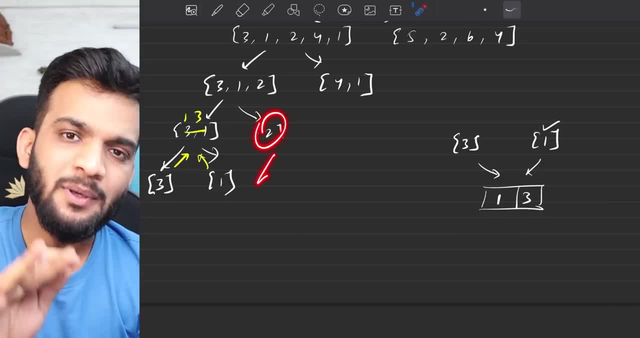 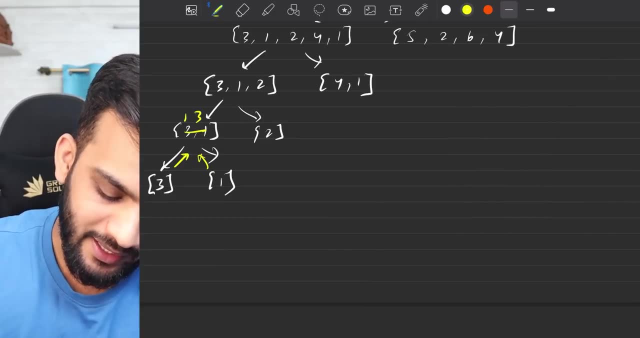 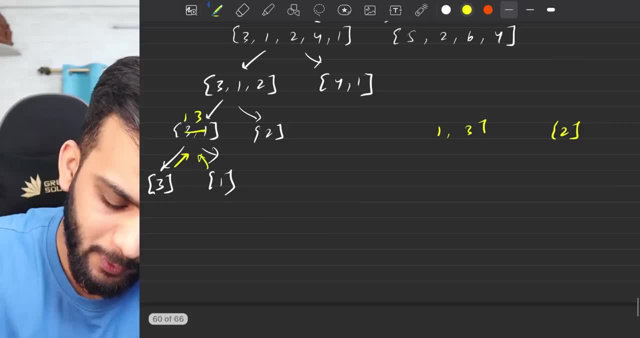 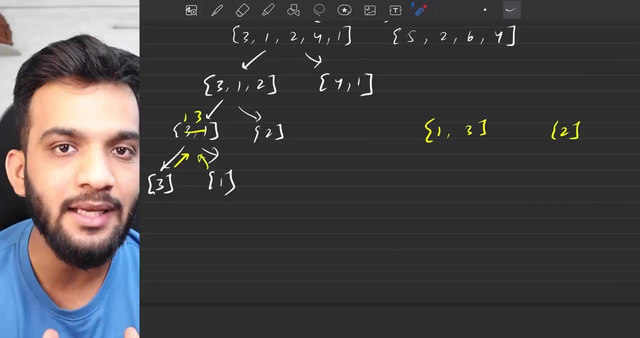 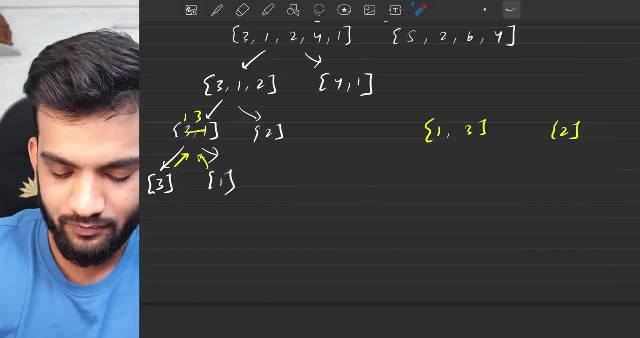 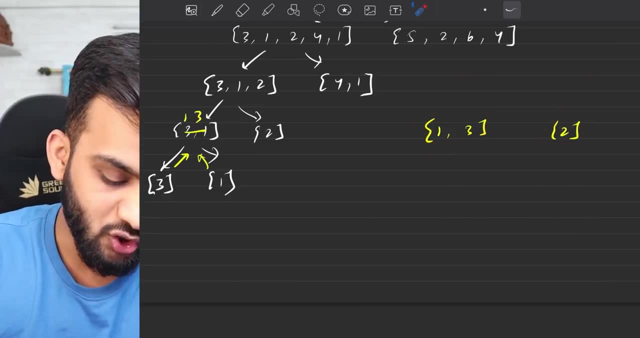 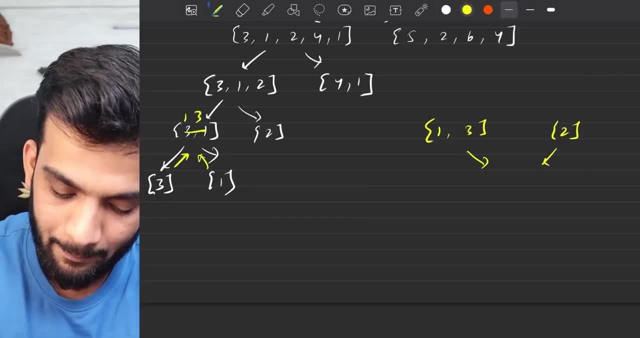 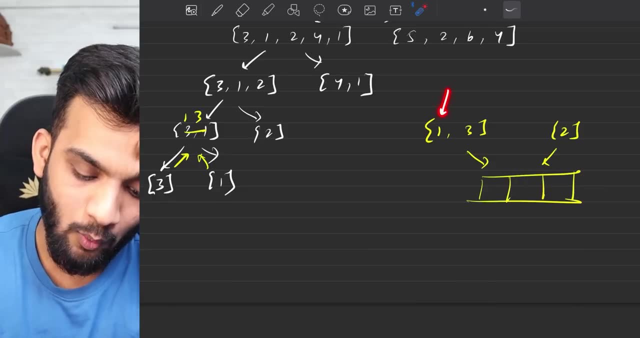 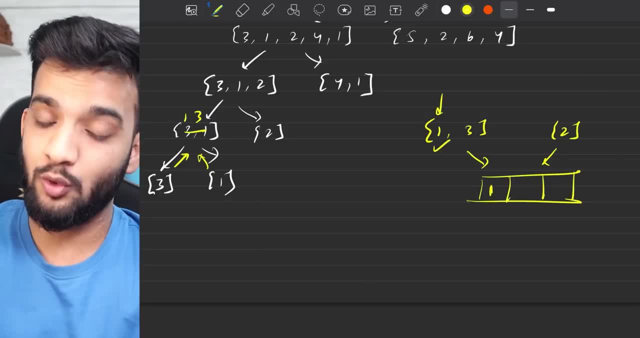 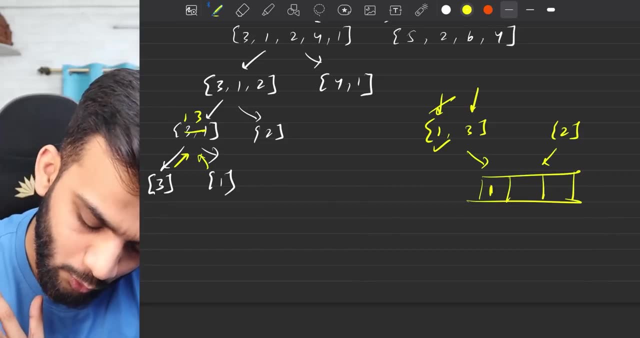 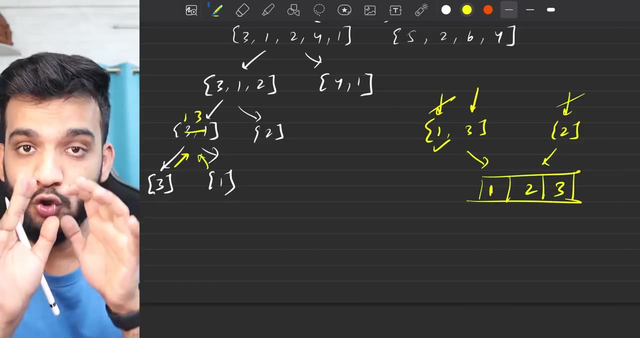 one. so you took one and you did not take two. so the moment you've taken one, the next you will say: do i take three? do i take two, like i'll take two? so you took two. next, you're just left with one, so you will take three again. i'll explain this algorithm in depth, do not worry. so we basically 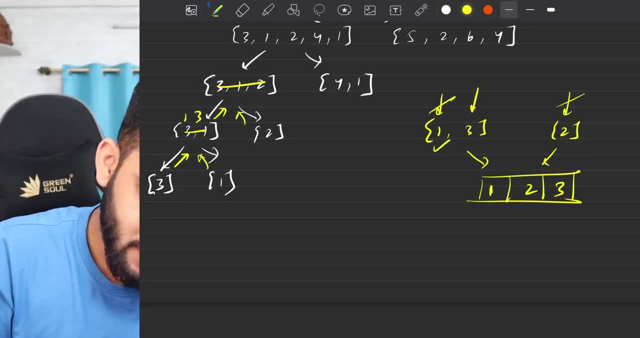 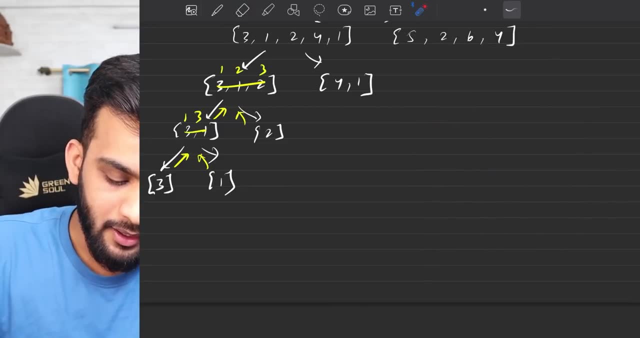 merge them again, merge them so we get one, two, three. the merging has completed. so can i say, initially, when i went to the left we had one, two, three, and when we went to the right we had four, one. so the left portion has divided and merged itself into a single. 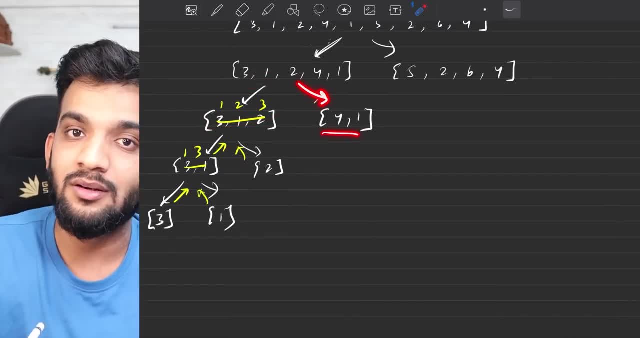 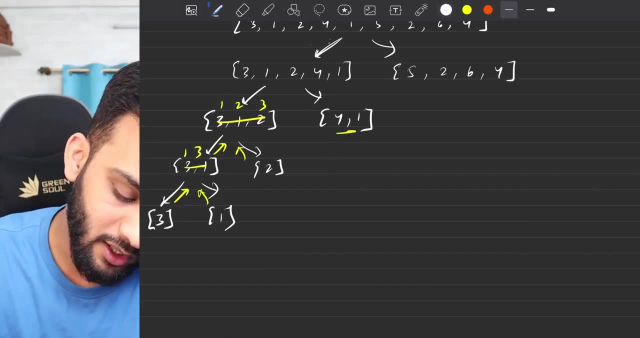 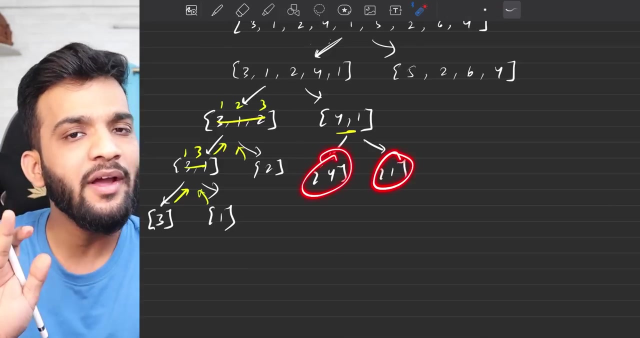 sorted array. it has it's time to go to the right. let's go to the right. so the moment you look at the right it has four one. so we again try to divide it. so if you try to divide it it will be four and one. can i say we can stop over here, because they are single elements and they cannot. 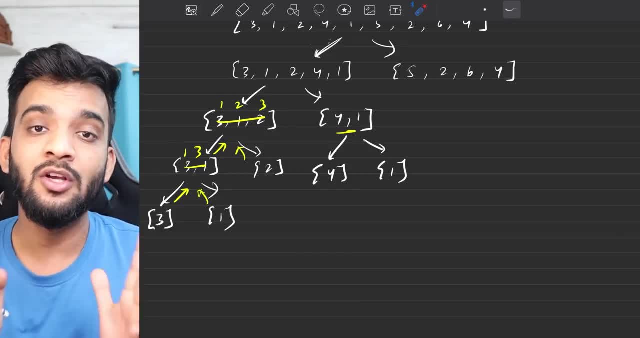 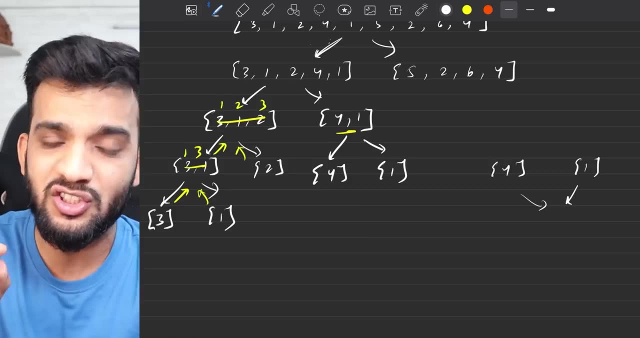 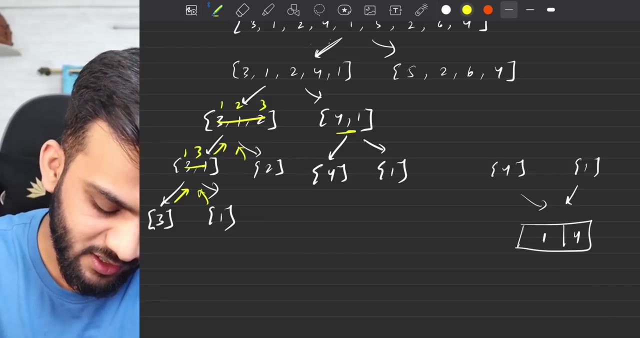 be further divided. yes, we cannot further divide them. so what we do is we stop. now, if it is four, if it is one, and if you have to merge them into a single sorted array, first one will come, then four will come. so what will happen is they will try to merge them and you will get one comma four. so can i say 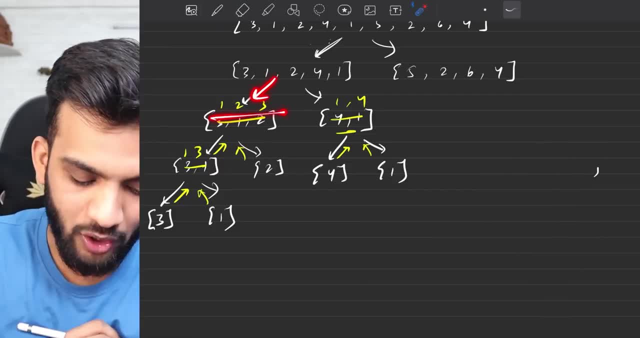 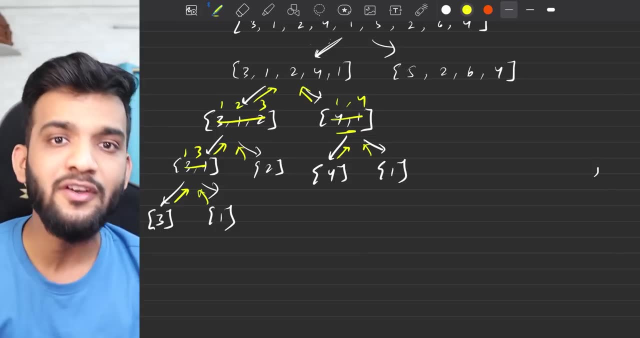 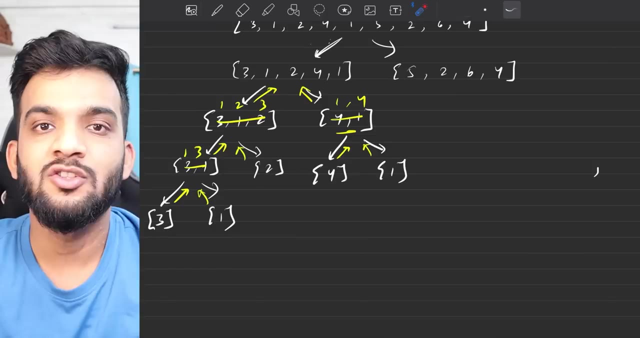 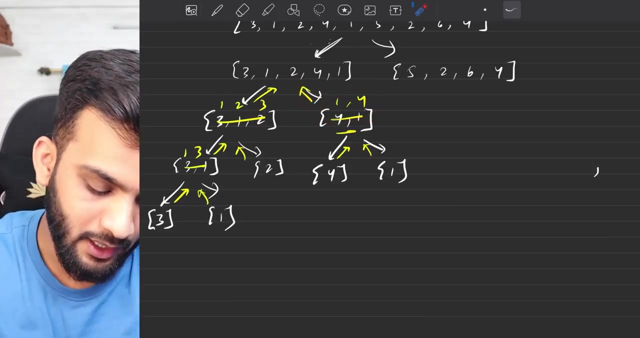 can i say that this one went, got it sorted, this one went and got it sorted. so basically now they both will come back because the left half is sorted and the right half is sorted. if both of them are completely sorted, what will happen? so can i say it went left and it got itself sorted. it went right, it got itself sorted. it's. 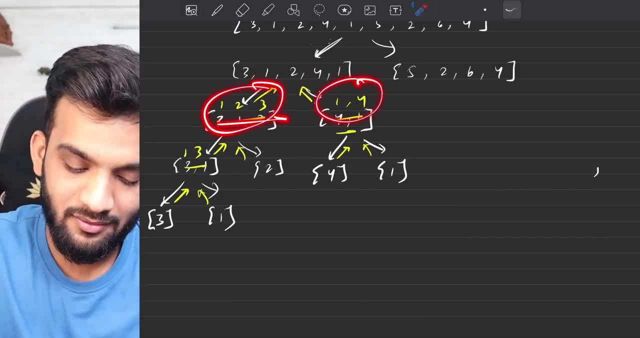 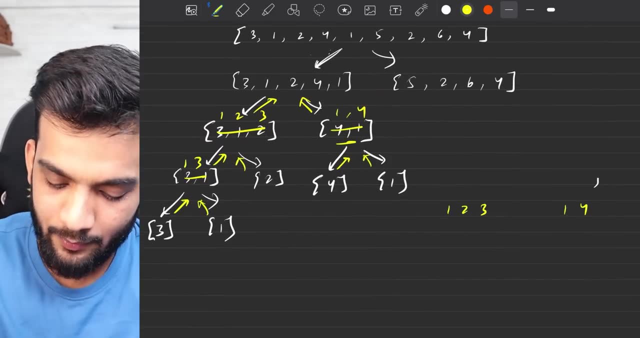 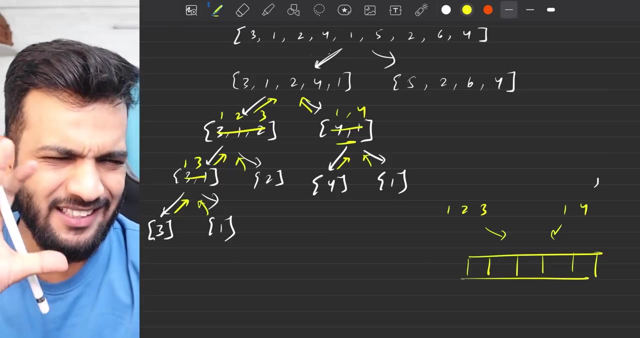 time to come back. so they will get merged. very simple, let's write it again: one, two, three and one four, and they will try to merge themselves. into how many elements? definitely, yes, five elements. so let's kind of now try to get into the algorithm. and you know, this is the smallest. 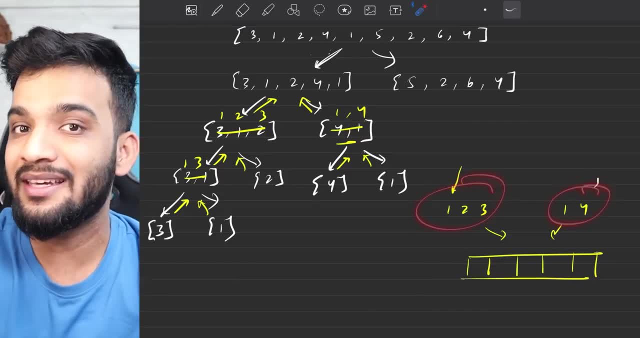 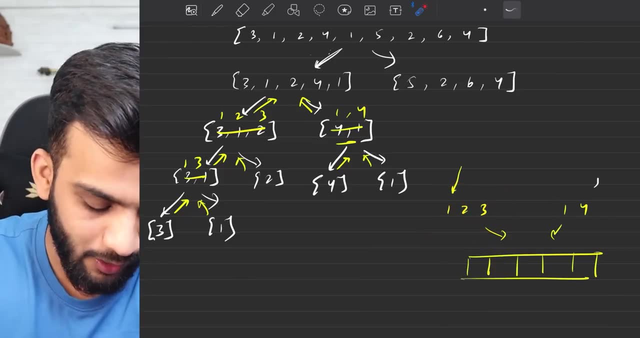 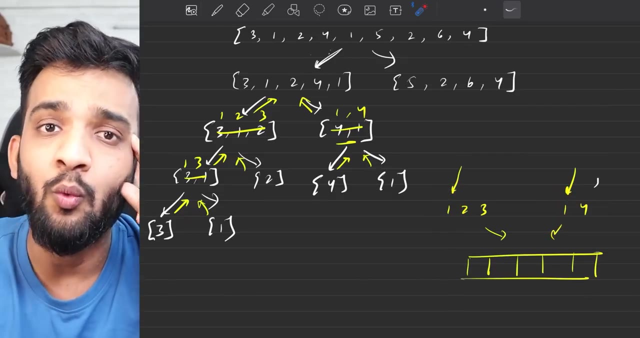 element on the left half. if i say there are two hypothetical arrays, can i say on the left the smallest element is definitely on the beginning because both the arrays are sorted. so we will take one. we will take one. we have one over here. we have one over here. i have to ask you which one. 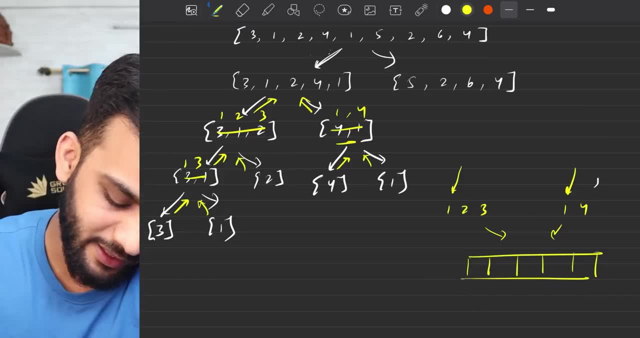 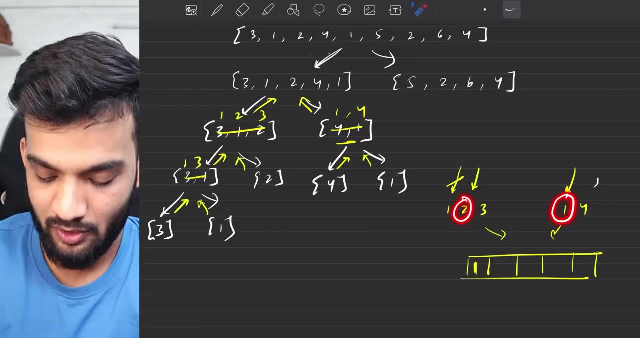 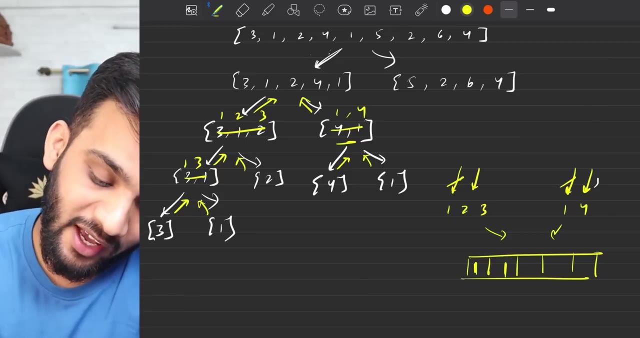 will occupy this. it can be any of the ones. i take any of the ones and maybe i'll just move it now. if i have to ask you out of two, out of one, which will occupy this, you know the answer: it's one. so you now move the pointer. next, if i ask you out of two, 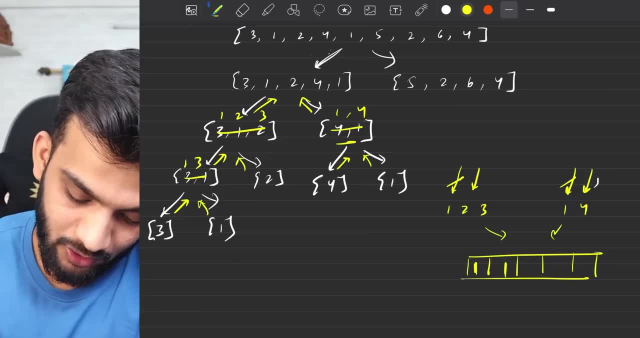 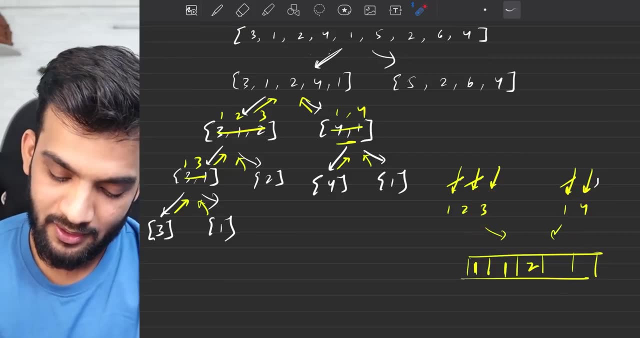 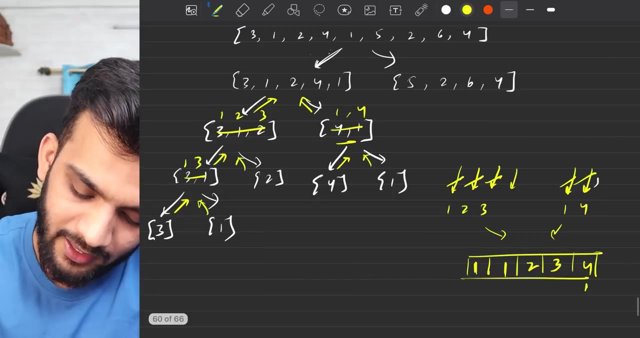 out of four, which one will occupy this? you will be saying two, so i'll move the pointer. next, if i ask you, out of three out of four, which one does occupy this particular guy, it'll be like three and this will move out. next, if i ask which one will occupy this, you'll be like four and this moves out. so 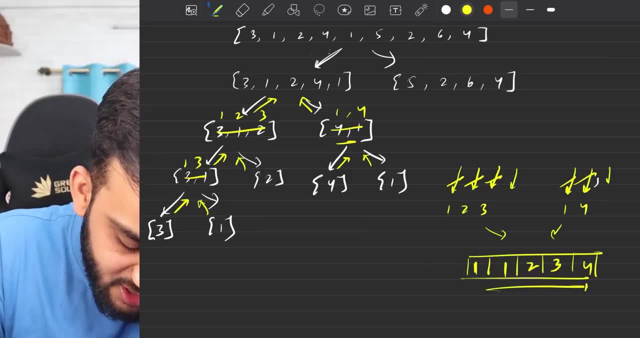 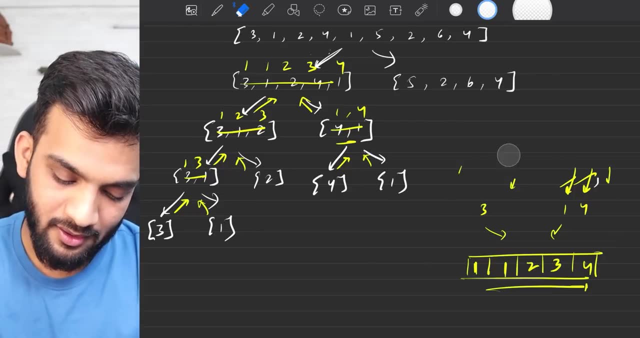 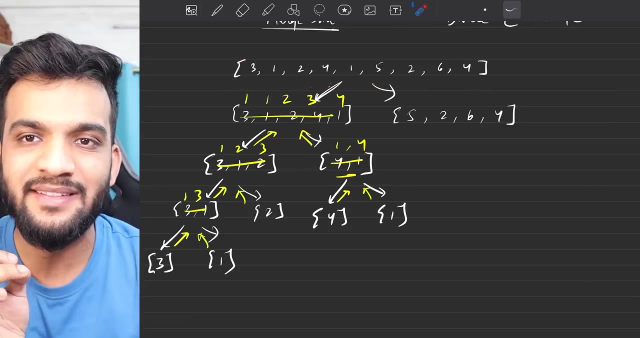 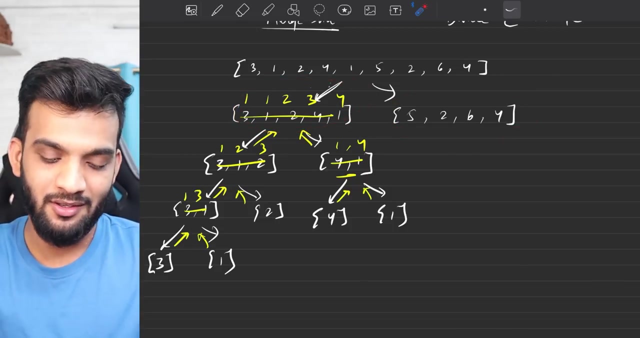 apparently you got this entire thing sorted, so i can. i see this will become one, one, two, three, four done, so this half is sorted. so we started with nine numbers. we split them into five on this side, four on this side. five guys are have been sorted by the algorithm: divide, divide, divide and merge. 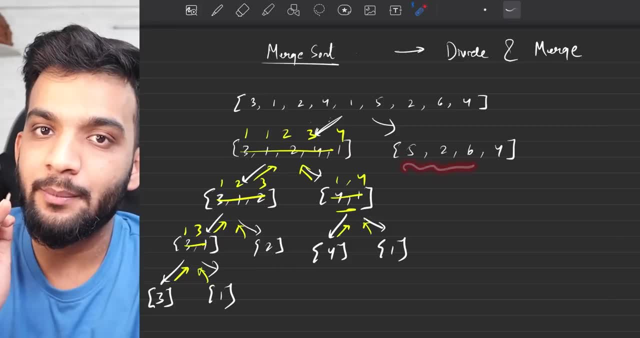 merge, merge. they got themselves sorted. now it's about these four elements. can i perform these? merge, merge, merge. they got themselves sorted. now it's about these four elements. can i perform these? can i perform these all? you can go to top. only then we can outsource, so you get solution like: 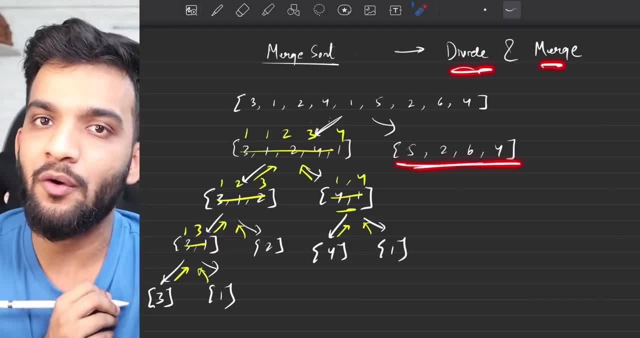 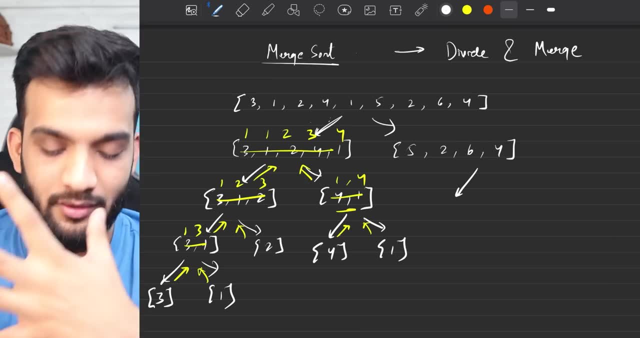 halTimes and K attempt silly, so sit with which link? look for the below inquiries at next. that's something, the same algorithm of divide and merge on these four i can. so what i'll do is i'll again start, because now it's the right half's turn to get sorted, so i'll not again divide the four elements. 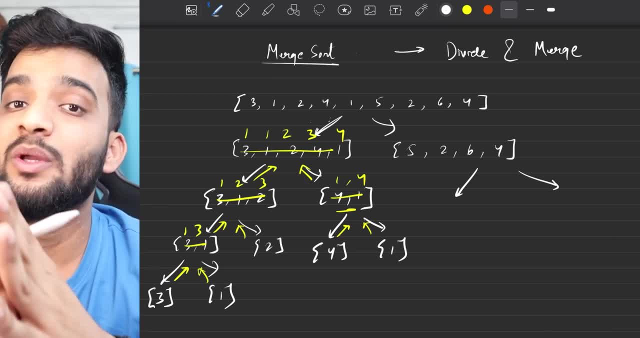 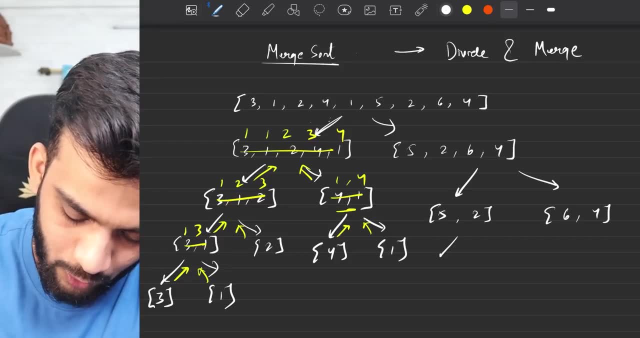 and if there are even elements, how do they get divided into equal number of elements? so it will become 5 comma 2 and 6 comma 4. 5 comma 2 will become 5, 2. so again can i say they will be sorted. 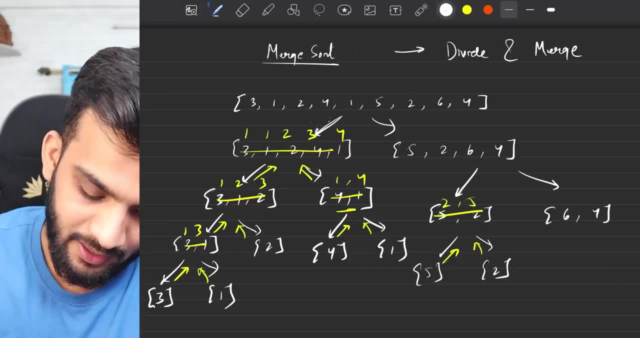 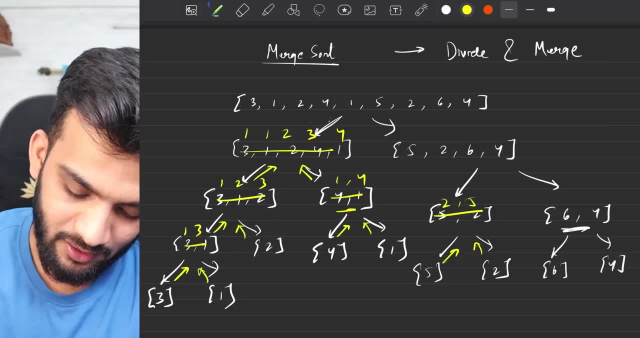 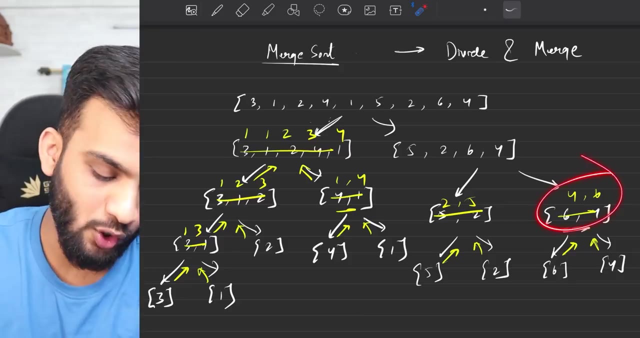 back into 2, 5, and now this one will take place, so it'll be like 6, 4. again it will come back. i'll say 4, 6. perfect, now can i say this portion is sorted, this portion is sorted, so now they will. 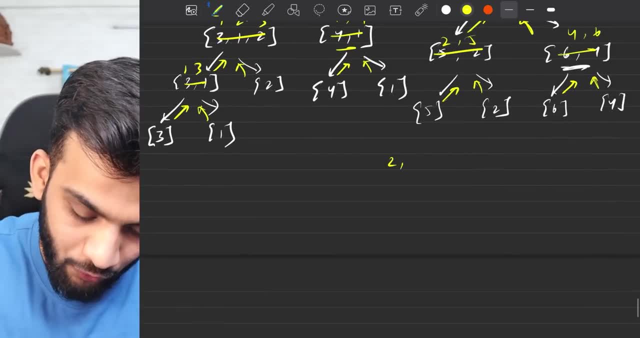 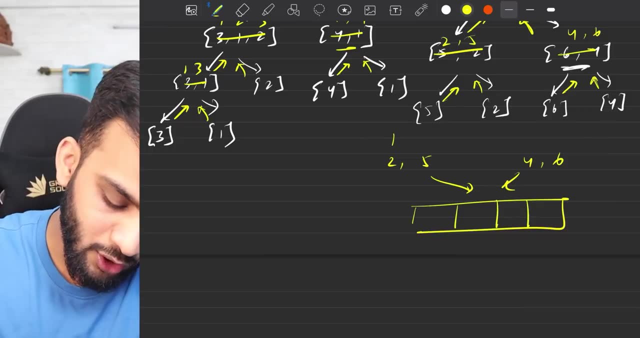 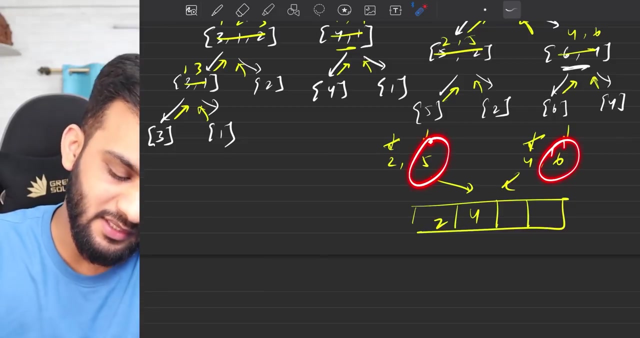 come back, and how will they come back? let's write it out: 2, 5, 4, 6, so both of them will get merged into how many elements? 4 elements 2, 4, 4. which one goes at the first? 2, 4 or 5, 4 or 5, 4. sorry, uh, now 6 or 5, yes, 5, next 6. it's like 2, 4, 5, 6. 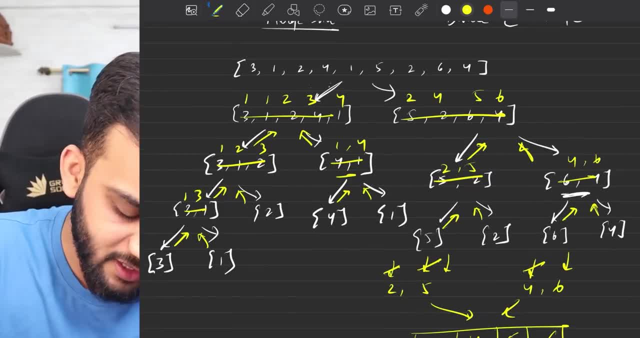 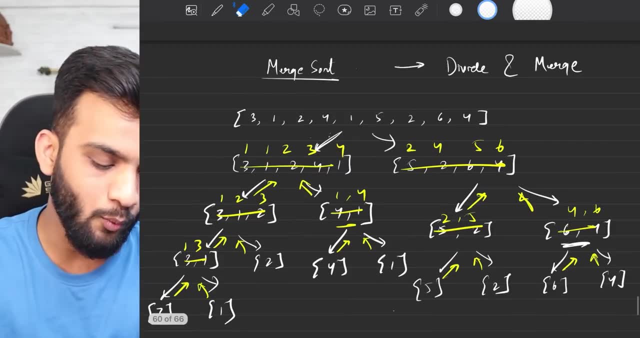 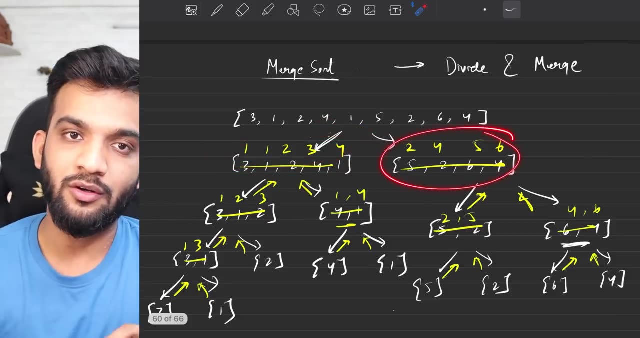 very simple. so this becomes 2, 4, 5, 6. we can go ahead and erase this as well. got a bit clumsier, but i'm i'm assuming you're getting the explanation now where are we? can i say: we went to the left, we got everything sorted. we went to the right, we got everything. 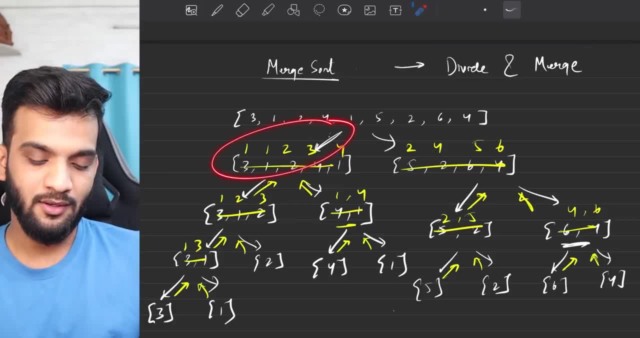 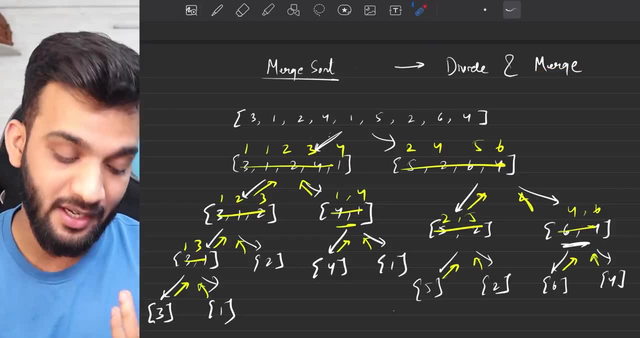 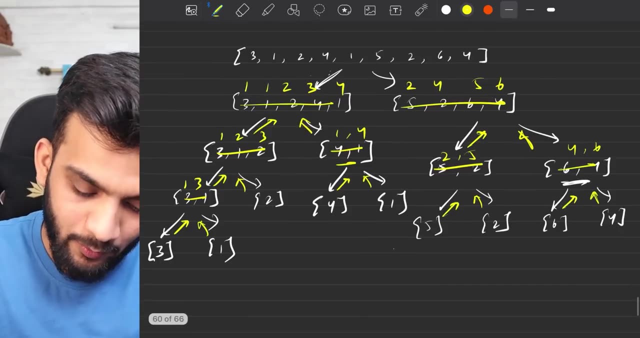 sorted. the left: the left five elements are sorted, the right four elements are sorted. what is that we need to do? we need to merge them. we need to perform the last step, that is, merge. so these 1 1, 2, 3, 4, 1 1, 2, 3, 4, and on the right, we have 2, 4, 5, 6. we have 2, 4, 5, 6. they will get merged. 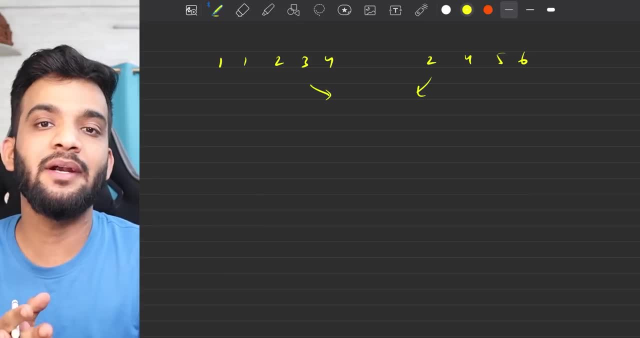 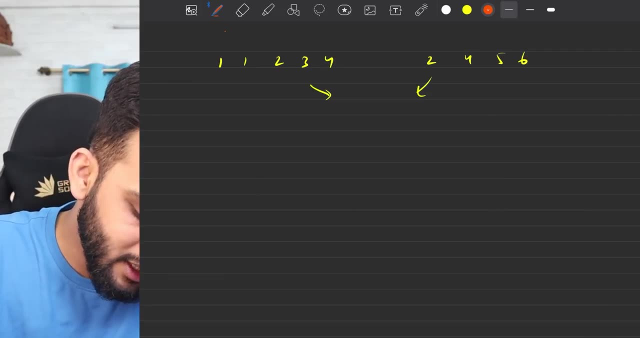 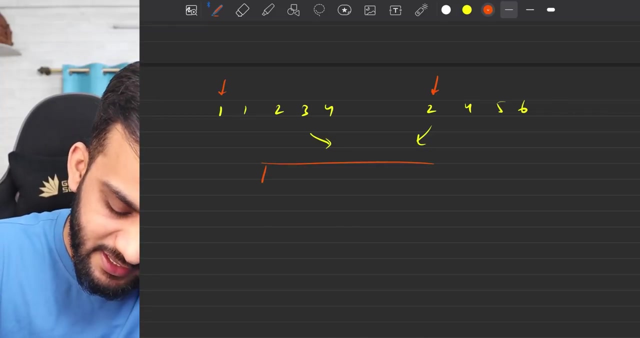 into 9 elements, and that will be my ultimate sorted array. how do we merge? let's now understand the algorithm in depth. so what we do is we keep couple of pointers- one here, one here, okay- and then we create an array of size. let's say nine: one, two, three, four, five, six. we created an array of size. 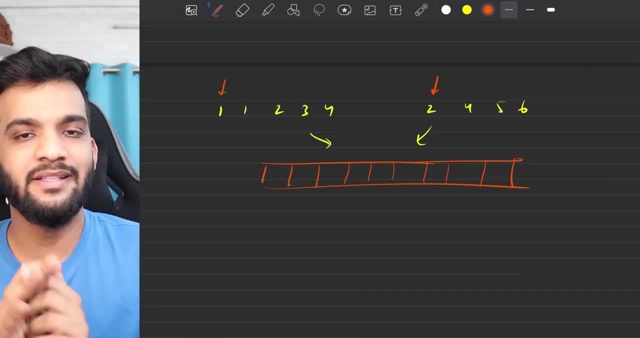 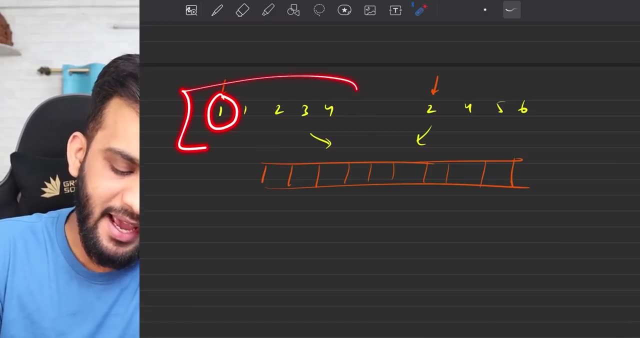 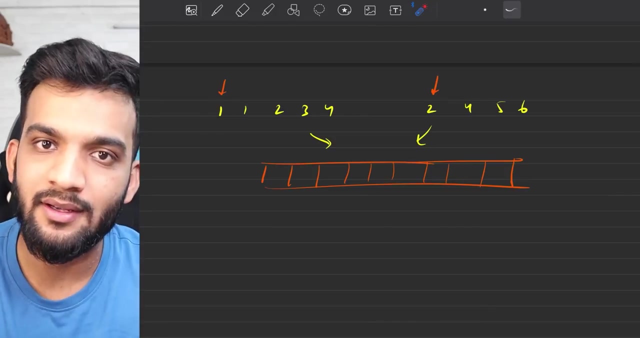 nine, or you can create an empty array and keep on piling it up. that's your choice. we will take care of that during the implementation. so we know this entire left array is sorted. we know the entire right array is sorted, so we have to combine them to get a sorted array. so out of one and out of two. 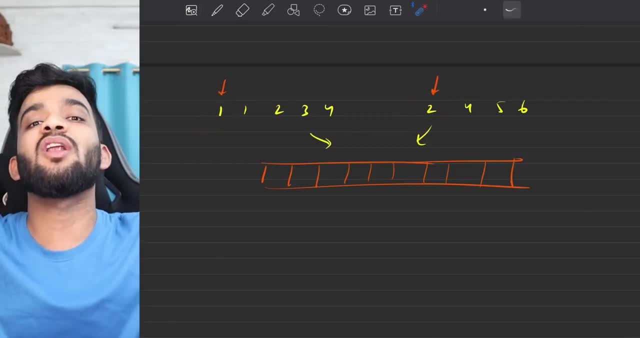 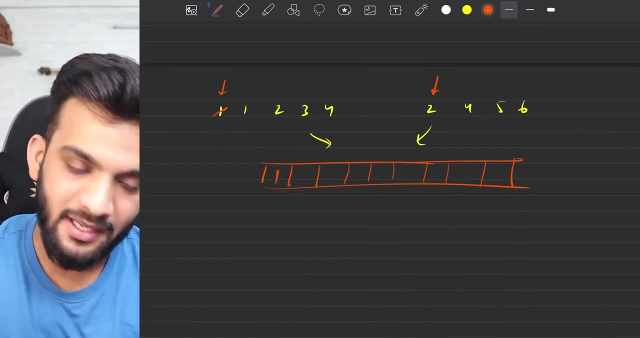 because both of them are smallest. i know i've taken the two smallest guys from left, from right. which one will take this place? you say one, so you take one and you place it, and the moment you've taken someone you'll just move the pointer. let's start. 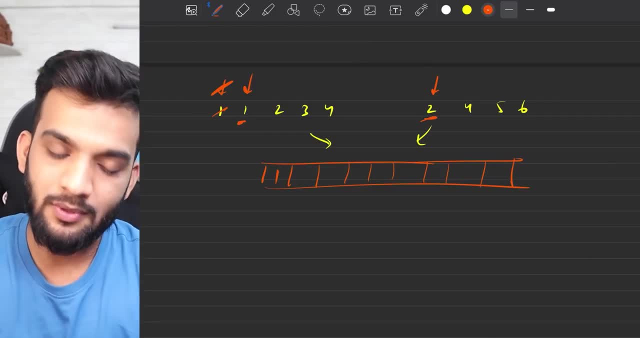 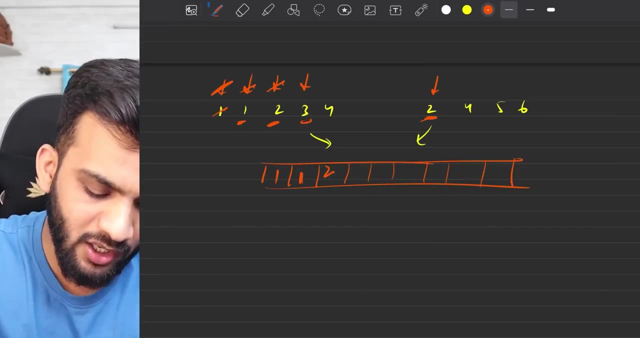 start. start moving the pointer. got it. you take one or you take two. again, you take one and you move the pointer. you take two or you take two. you can take two and you can move the pointer. you'll take three or you'll take two. you'll take two and you'll move the pointer. now, will you take four? will you take? 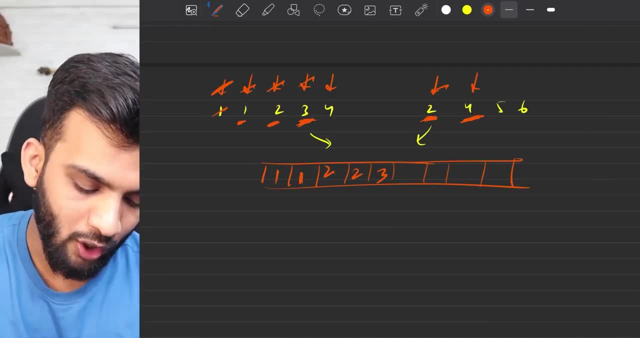 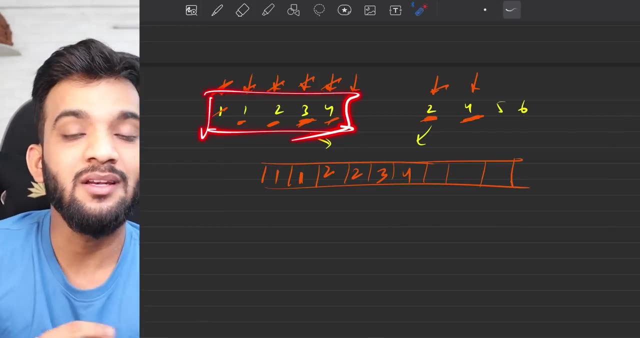 three. you'll take three and you'll move the pointer. now, will you take four or will you take four? you can take four and you can move the pointer, so we can say the left array has been exhausted. please hear me properly. i can say the left array has been exhausted. please hear me properly. i can say the. 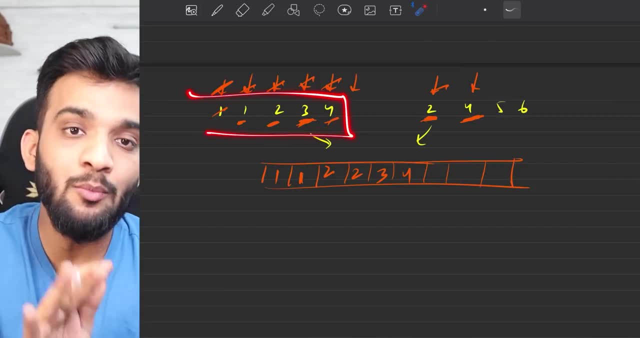 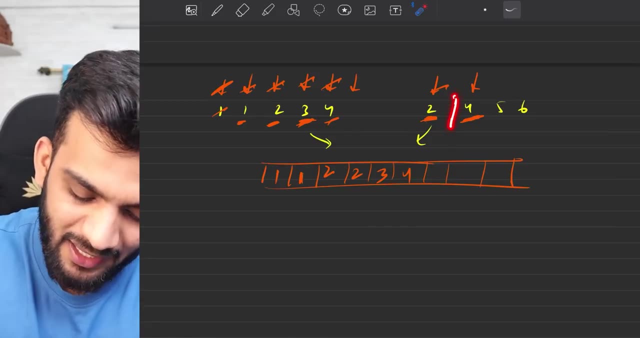 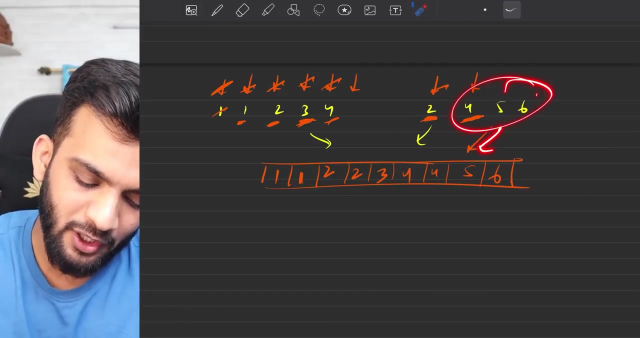 the left array is completed, it doesn't have any more elements that can go over here, so what i will do is, without doing any further comparisons, i'll pick up everyone from the right and i'll just put it over here. i'll pick up everyone from the right and i'll put it over here, because there. 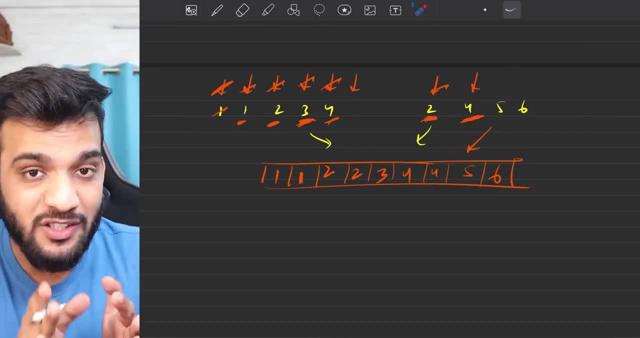 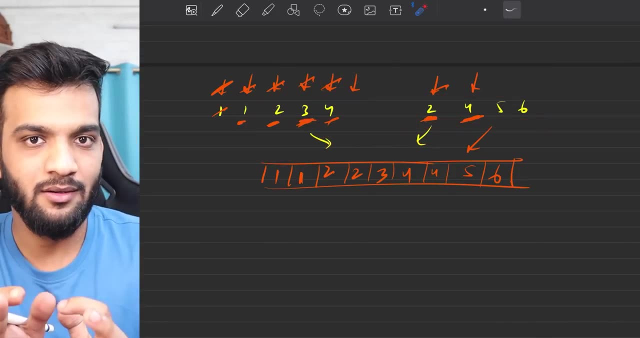 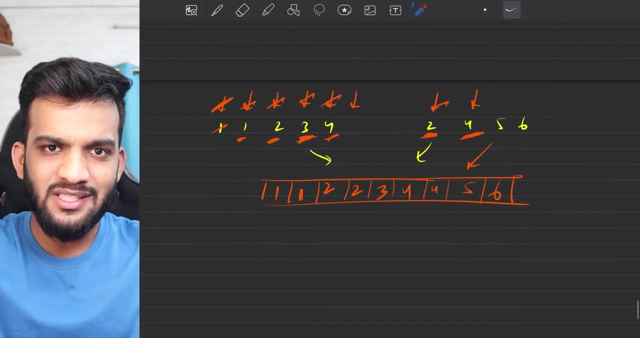 is no one left on the left got it. if something similar happened- that the right element got completed- then you would have taken this and you'd have put it in. doesn't matter. so it's very simple. if i have to define the merge algorithm, it's very simple. you take two pointers. 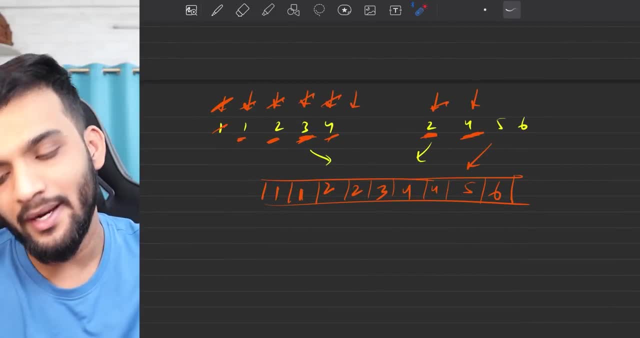 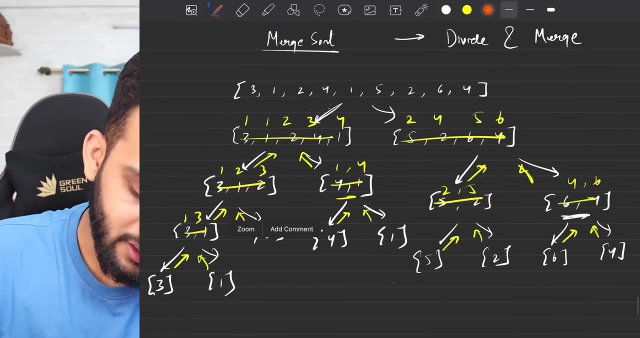 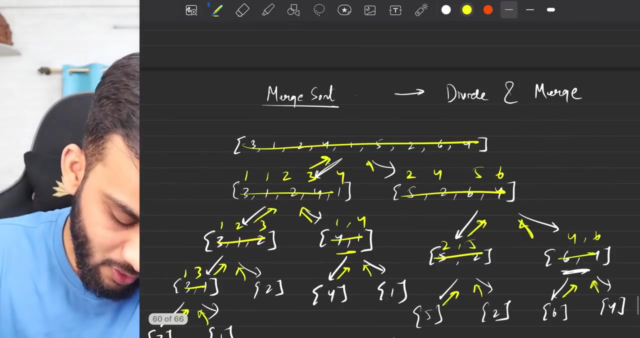 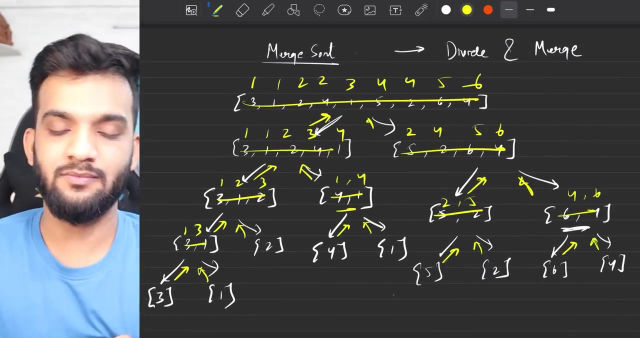 compare: put, put, put. one gets completed, the other one gets put. we will implement this, do not worry. so we have done the sorting. so the last step, what will happen? they come back, they come back and this will be: one, one, two, two, three, four. one one, two, two, three, four, four, five, six, four, four, five, six. 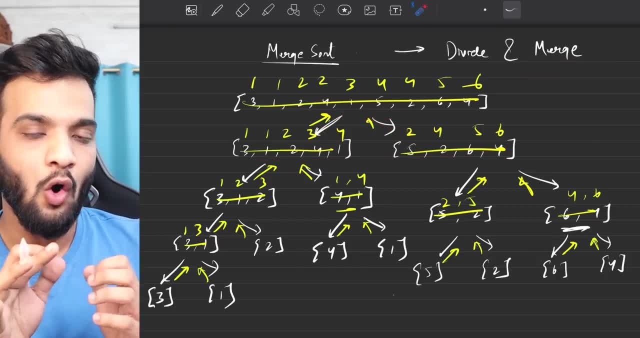 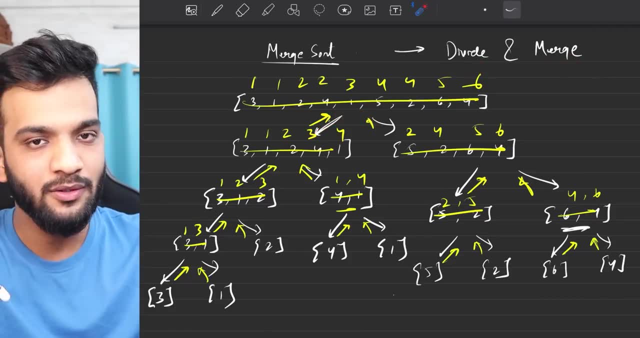 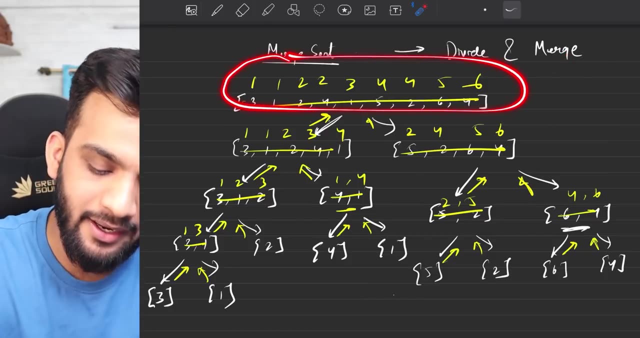 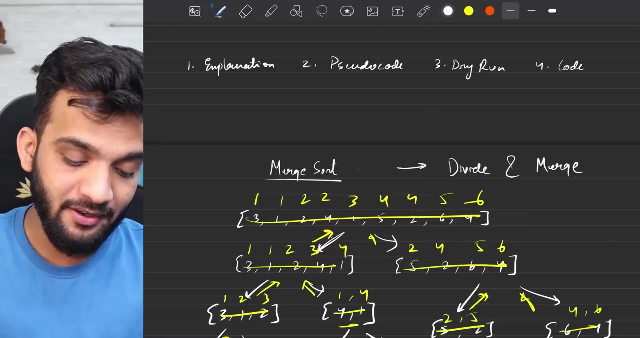 so can i say after i have completed all the steps of divide and merge. if you carefully notice, the last step was merge in the entire algorithm. so once i perform both of them completely on all the parts of the array, the array that i get will always be sorted. this was the algorithm. i hope you have understood the explanation. okay, so i hope you have. 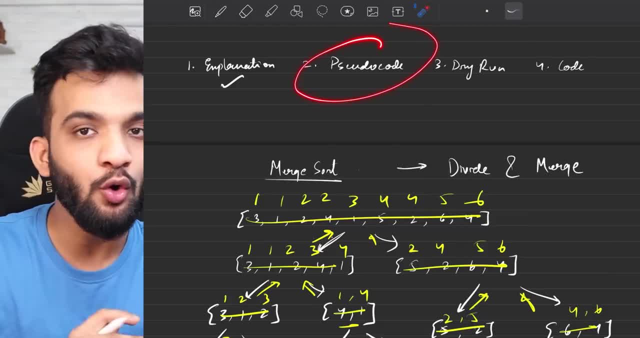 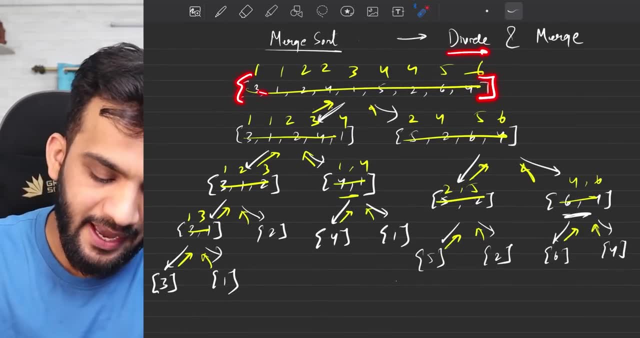 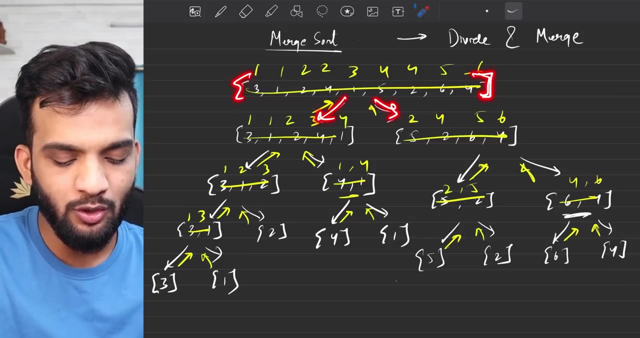 understood, uh, the explanation. it's time to understand the pseudocode. the first thing that we have to observe is: what are we doing? we are dividing. we are dividing the array into two halves, but, logically speaking, if you're going to break the, break the array down into two new arrays. 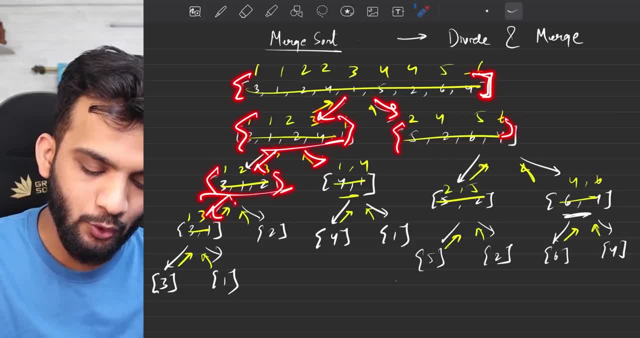 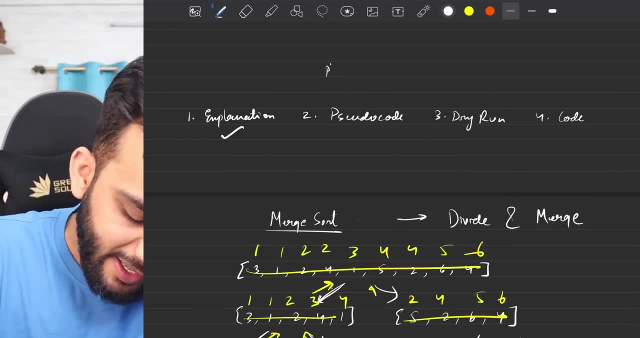 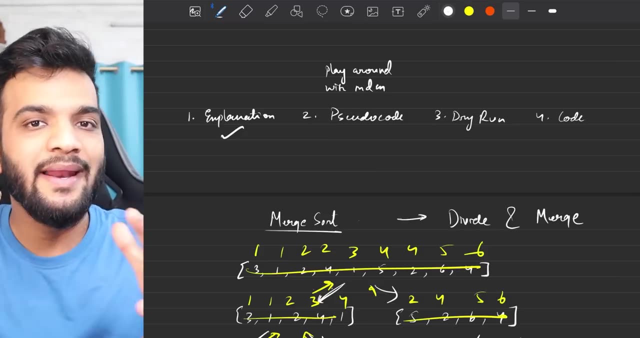 and then again this array into two new arrays. again this array into two new arrays. well, it makes no. this is where, in the pseudocode, we will try to play around with index. instead of breaking them down into two new arrays, we will try to play around with indexes. okay, so, in order to write, 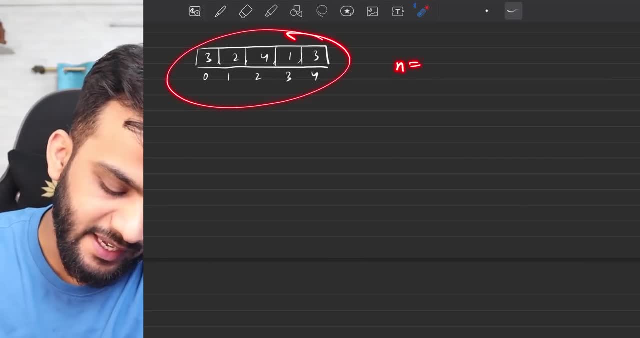 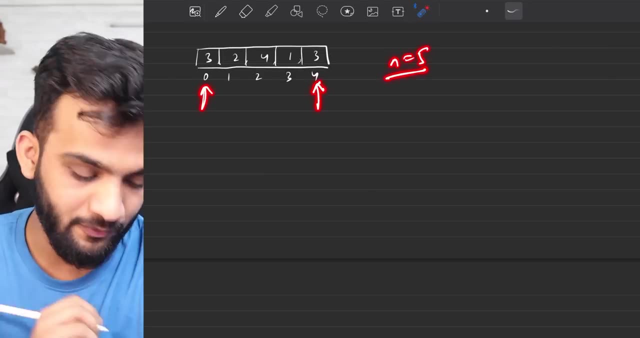 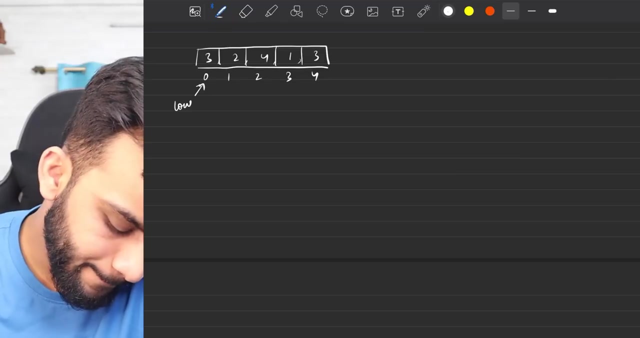 the pseudocode. what i've done is i've taken a very small array of size, five. now you know the array indexing starts from zero and it will go to four if the size is five. so what i will say is: c. this index will be referred as my low. this index will be referred as high. so what does low and high? 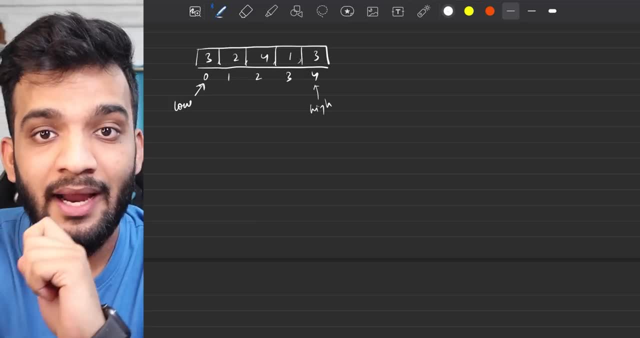 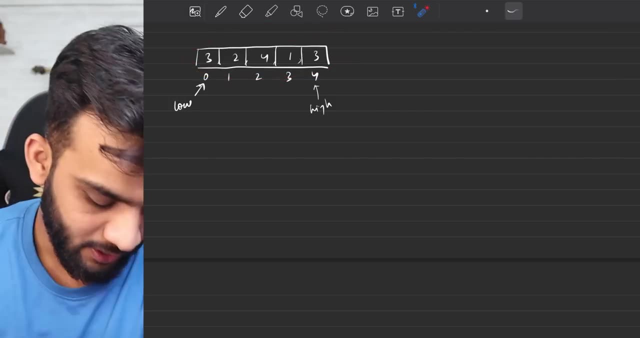 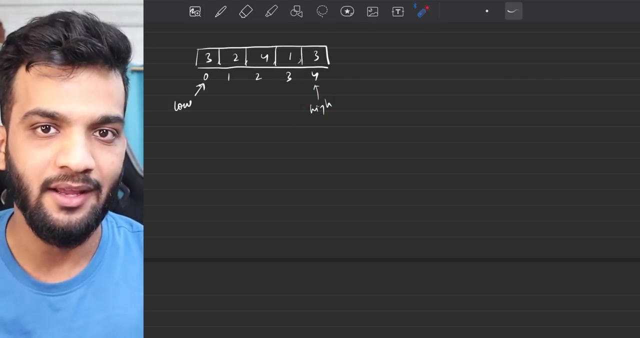 means is the starting point of an hypothetical array and high is the ending point of an hypothetical array. so initially we have an entire array that has to be sorted. so low is the starting point of that entire array and high is the ending point of that hypothetical array. got it okay, so let's try writing the pseudocode for this smart shot algorithm. 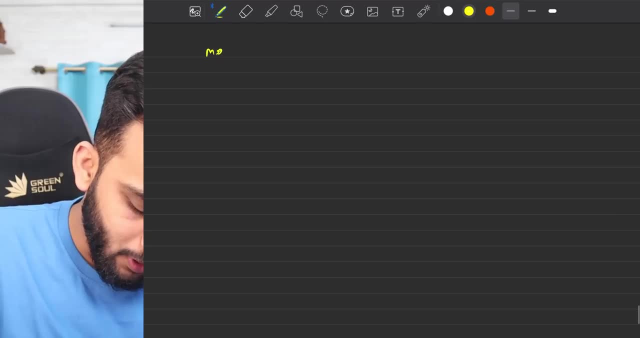 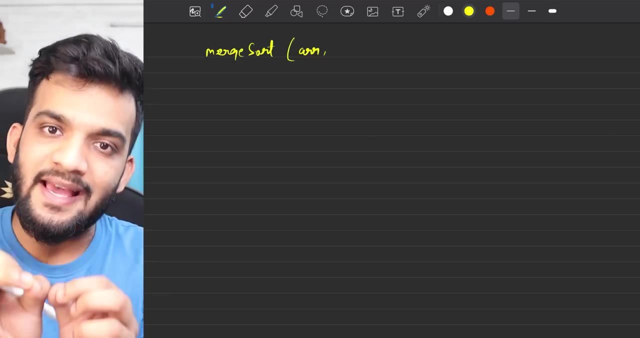 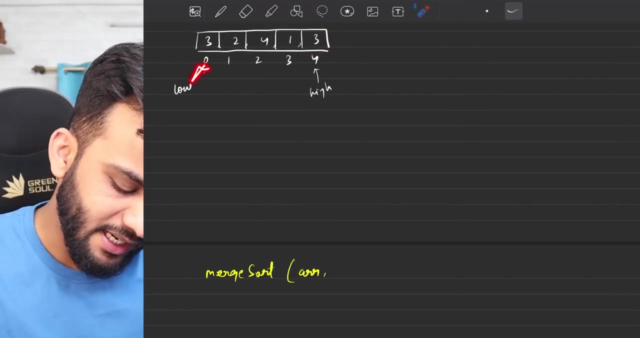 so i'll go ahead and write the function name as merge sort and initially i'll pass the array and i will say in this array: initially please consider the entire array that you have to sort. so the hypothetical starting point of this array is low and this is high, which means take the 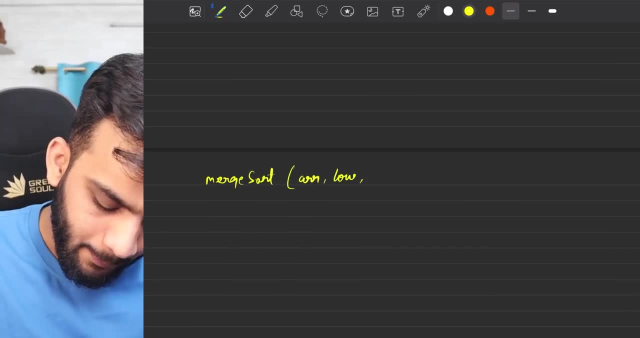 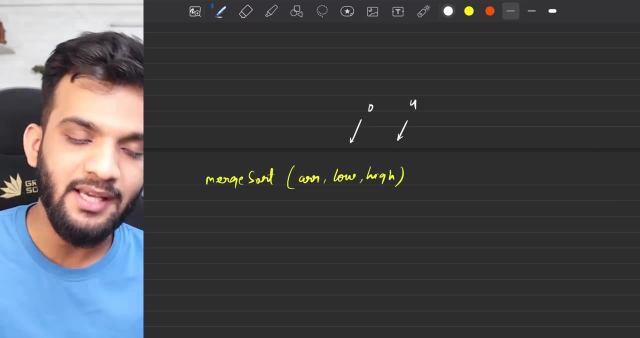 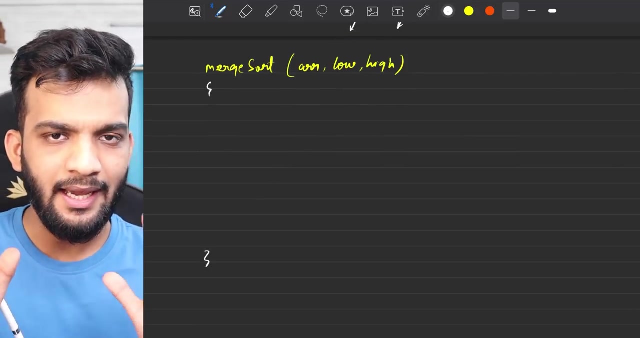 entire array. so i'll pass him low and i'll pass him high and initially, when this is called, low is going to be passed as zero, high will be passed as four. very simple, let's go on and as of now, i'll not write any condition. i'll keep conditions apart. so how do i write this algorithm? let's try to. 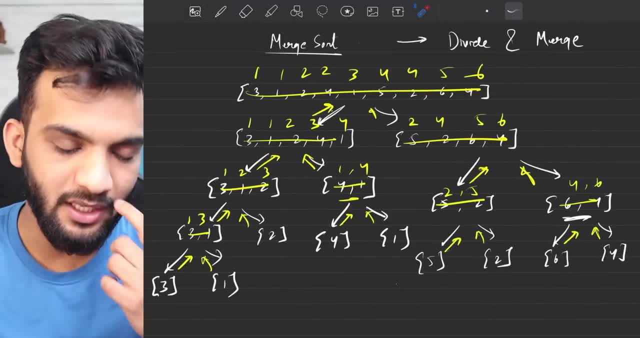 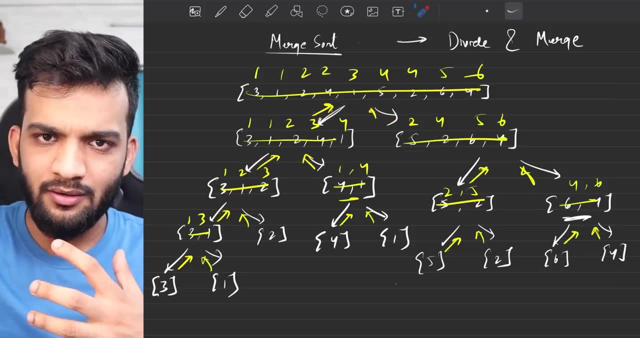 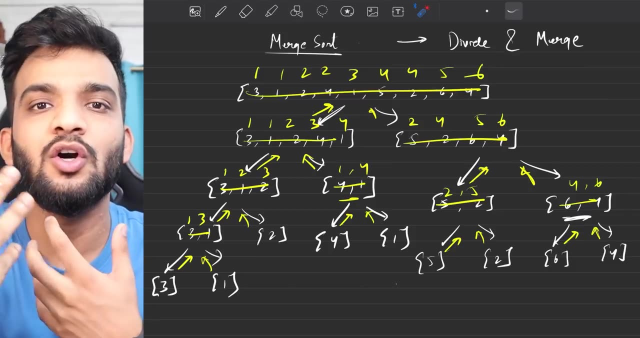 observe something: what are we doing repeatedly? are we doing something repeatedly? yeah, divide, divide, divide, divide, kind of doing divide, divide, divide, divide and at the last step we're trying to come back. come back. does it give you an idea that you have to apply something like a recursion? 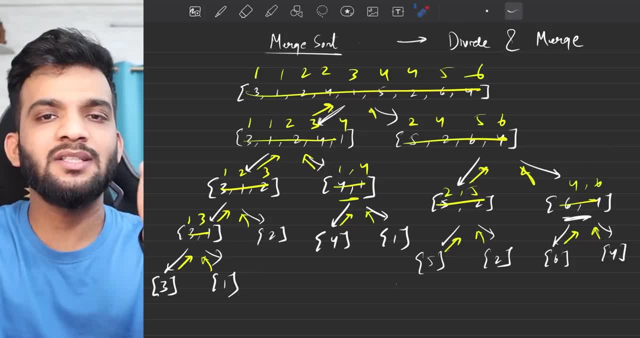 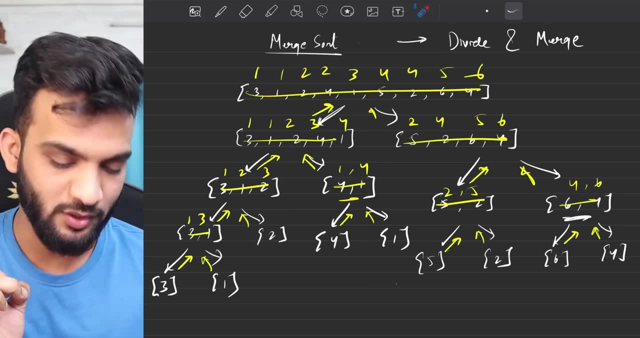 like you have to go divide, divide, divide and then you have to come back. that's kind of like recursion, backtracking. if you have seen the lectures, you can try to relate it with recursion and backtracking. that's what we will be using, so what i will say is: okay. now, what is the thing that? 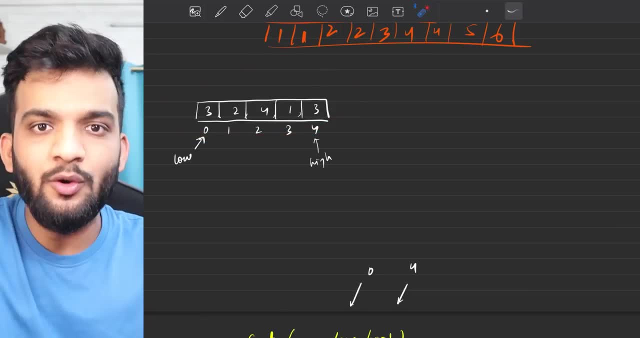 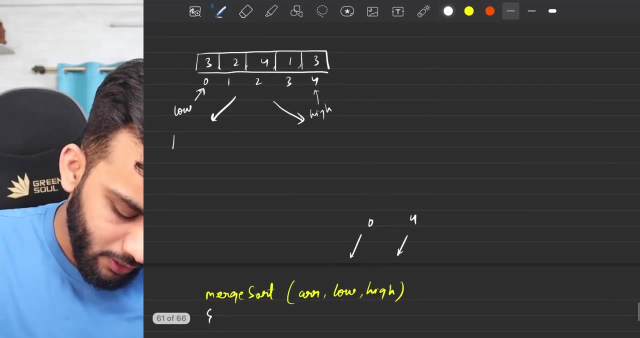 i'll do. i'll try to take this array and try to break it down into two parts. that is what i'm doing. i'll try to take this array and i'll try to break it down into two parts, where the first one to be three to four- that's how i was doing- the greater, like the three numbers at. 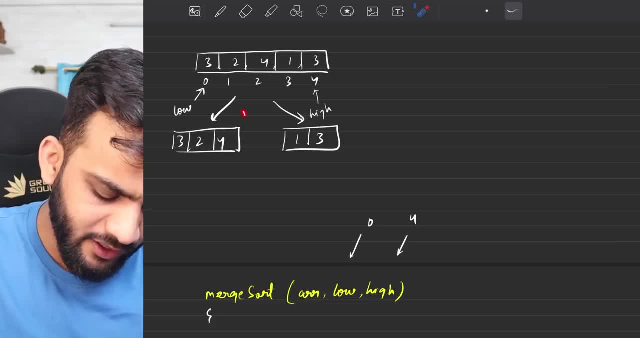 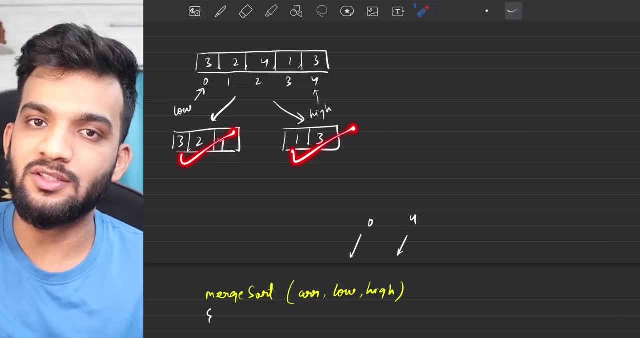 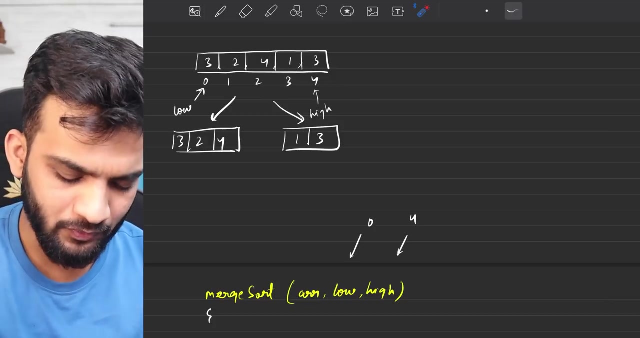 the first and then the two numbers at the back. so i'll say, i'll divide it into two parts, the left and the right. that's what i'm doing. and then i'll ask: can you please sort this, can you please sort this? once both of them are sorted, i can actually again merge them. that's what the algorithm was. 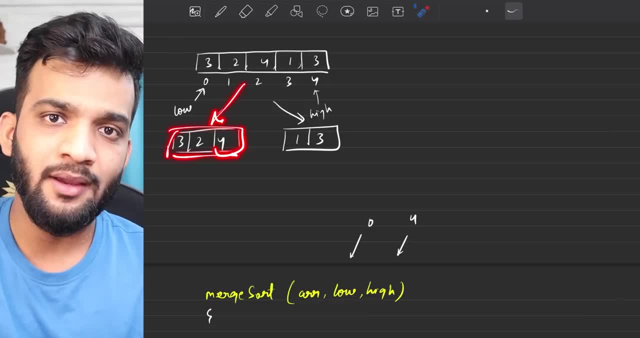 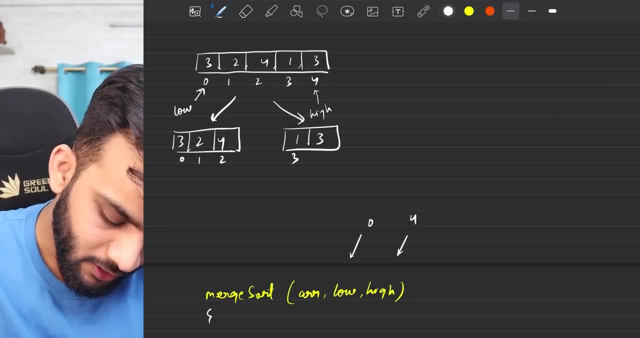 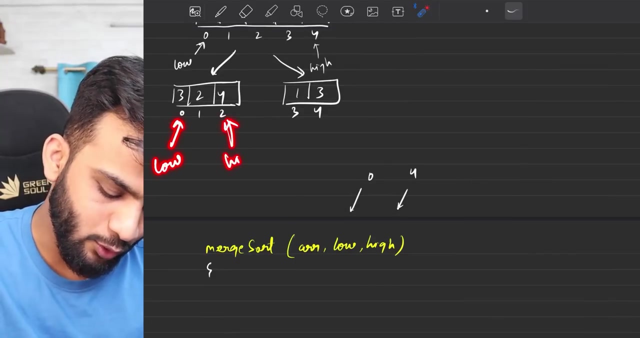 so i'll be like, okay, do i need to make a new array? no, this is where low and high comes in. i say, hey, listen, this is array indexing. so can i say: this array is nothing but an array where the low is at zero, an array where the high is at two. can i see this? i can. so if i 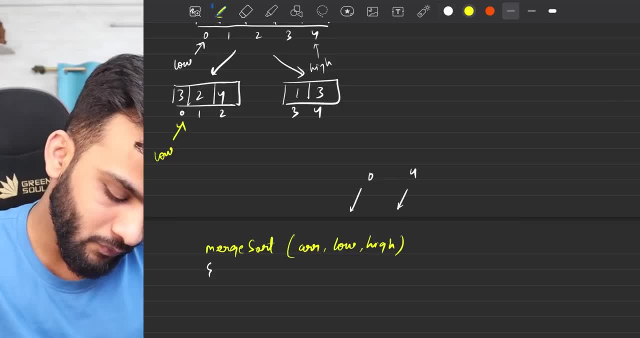 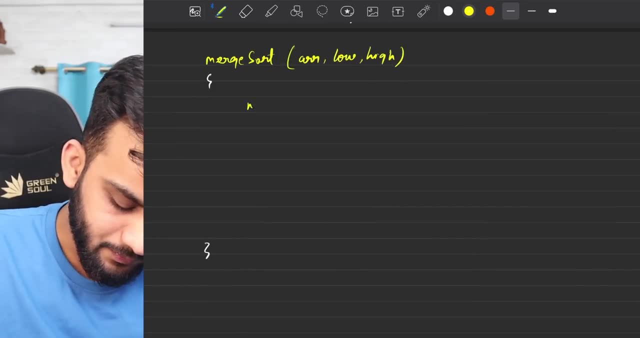 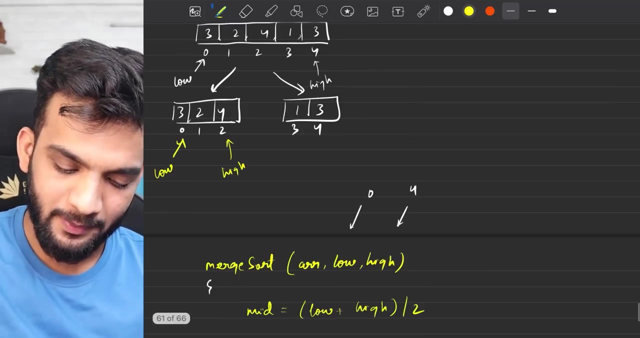 have to look properly. the low is at zero, the high is at two. that's what i'm doing. so i'll go and say that: hey, listen, maybe find a middle index. so middle is going to be low plus high by 2, very simple. so if you see over here what will be this, zero plus four by two will give you two. so 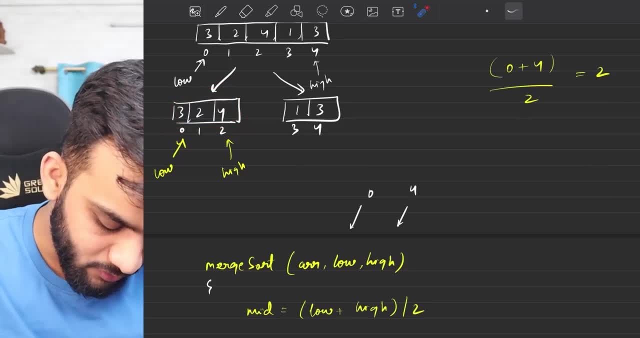 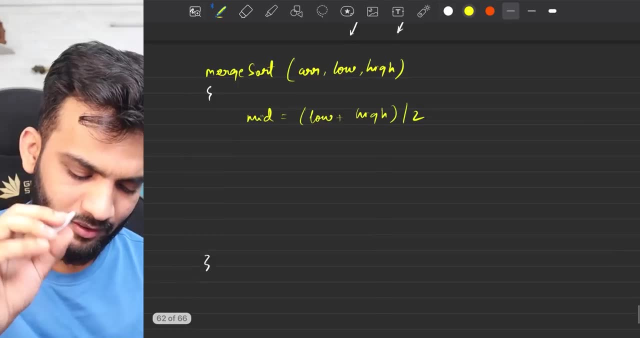 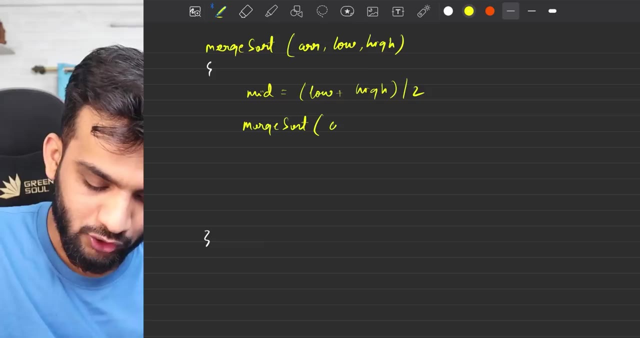 where is the first half of the array? it's from zero till two. and where's the second half? it's from three to four. so can i say: hey, please go ahead and try to sort this array, sort this array which starts from zero, which is apparently low. 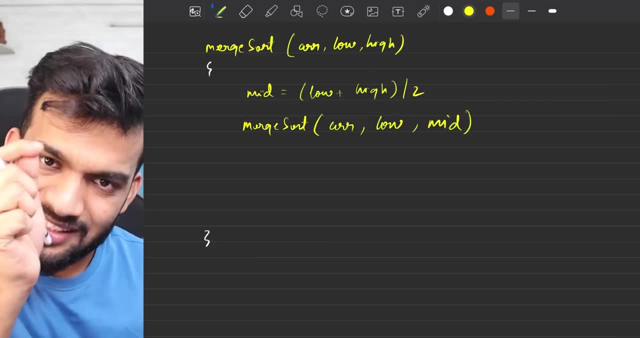 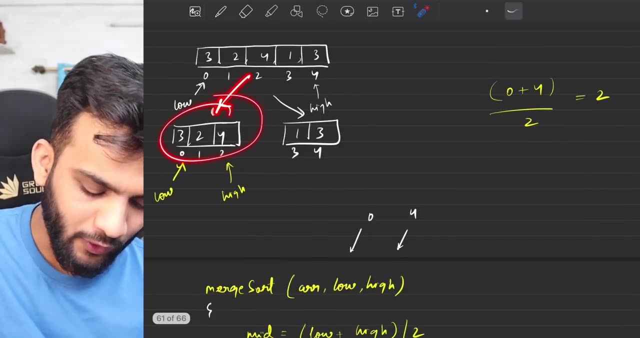 goes on till two, which is apparently middle, because in the first time the middle is two. and can i say: okay, this means i'm i'm asking him to do for this one right, but i have to also ask him to do for this one, because if he sorts this, 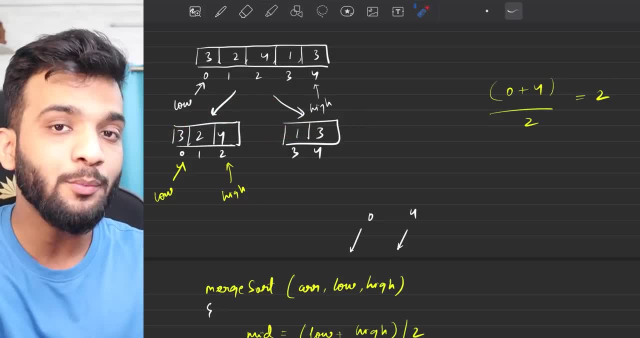 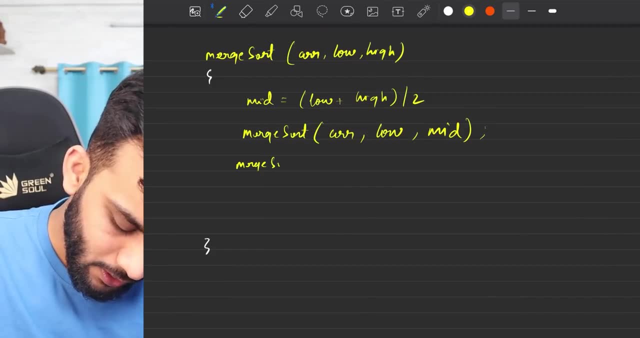 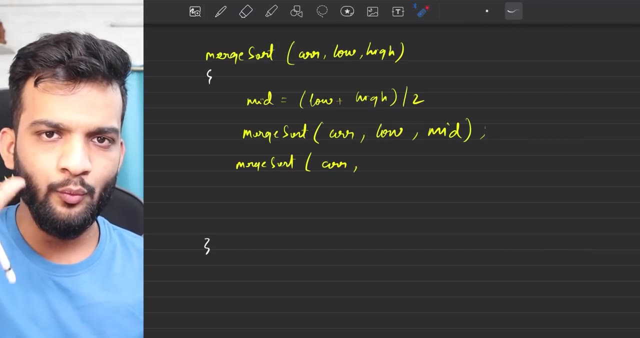 if he doesn't sort this, how will i merge them? because both of them have to be sorted in order to be merged. so what i will do is i will again say merge shot and i'll say array. can i get the right half of the array software? okay, in this array, which portion are you telling? 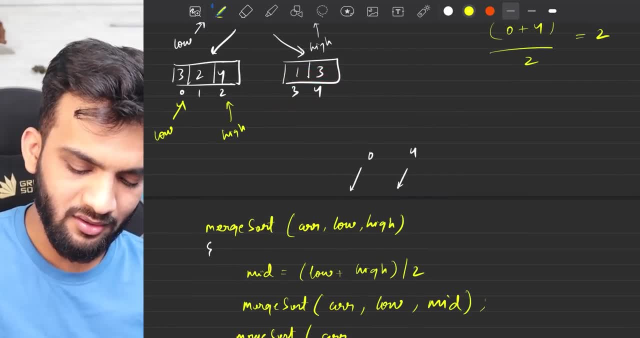 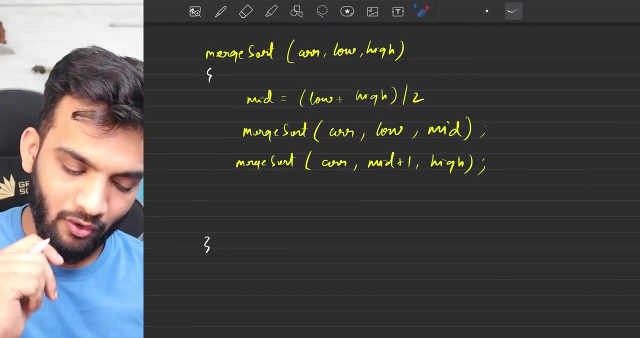 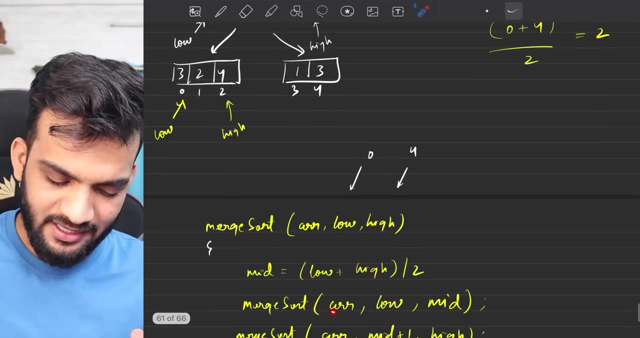 me to sort. i'm saying from three to four, what is three, that's nothing but mid plus one, because mid was two until high. so what i've done is, instead of making two new arrays, i told the indexes, i told in this array, take from low to mid, which is take from zero to two, which is this in this array. 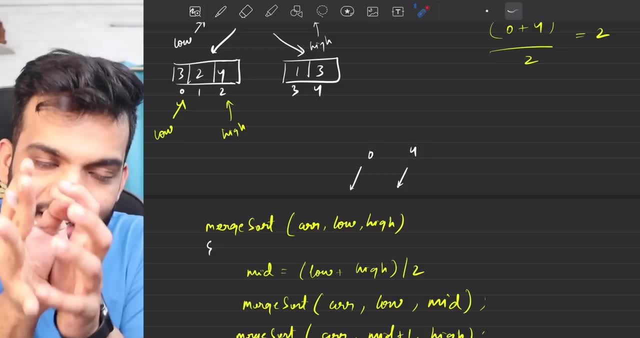 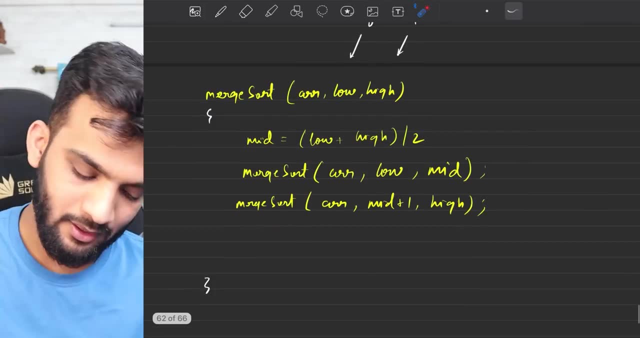 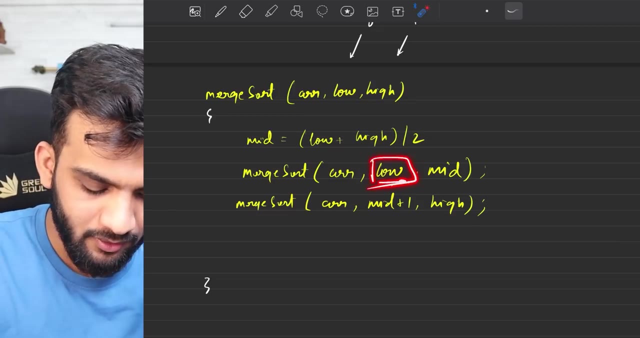 take from three to four, which is this. instead of dividing them into two arrays, i passed on the indexes and set them to one. set them to sort themselves. now, assuming that these functions are getting sorted by themselves. once the portion from low to mid, once the portion from low to mid. 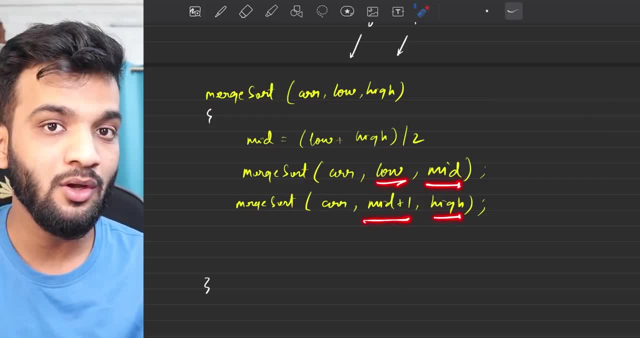 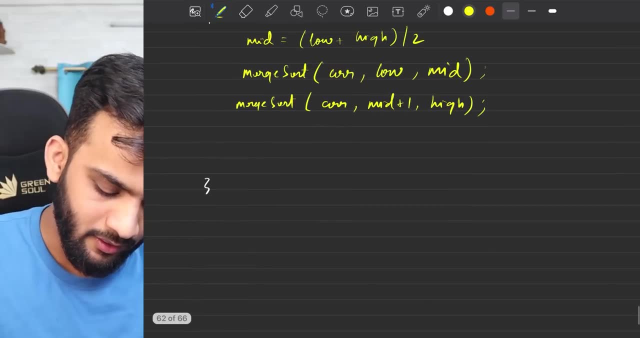 is sorted. once the portion from mid one to high is sorted, what is the next step? if you remember, the next step is merge, so probably i can say, if you remember, the next step is merge, so probably i can say that a, please go ahead and merge the array, the first half of the array is very simple. 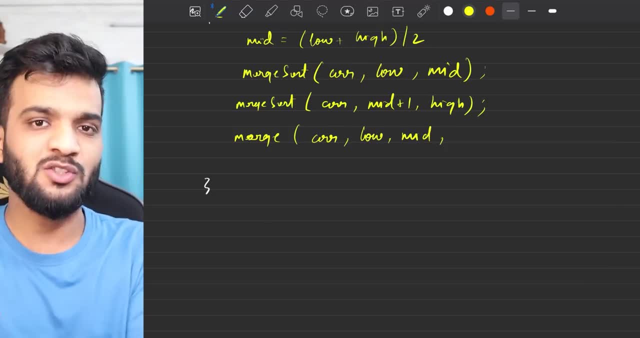 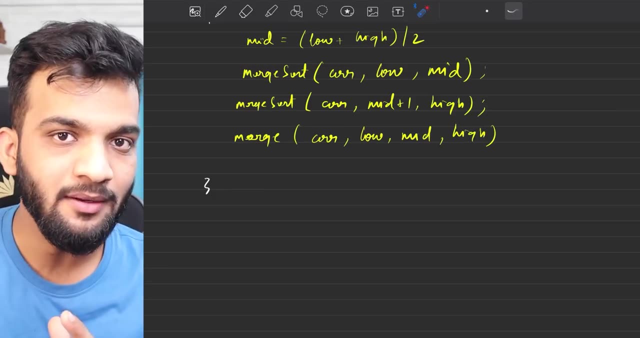 it goes from low to mid and the second half will be from mid plus one to high. so take these things and can you please merge this particular array? that's what i'm saying. that's what i'm saying, very simple. now, when do we stop? when do we stop is my question. 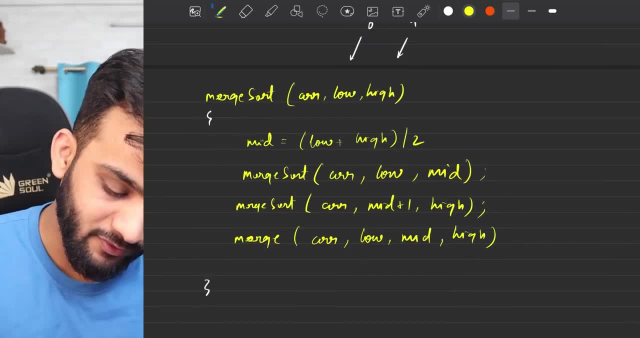 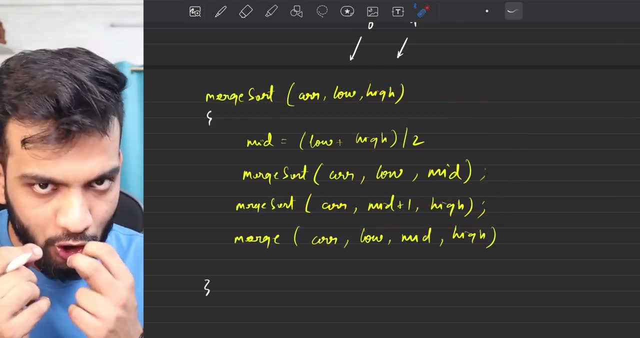 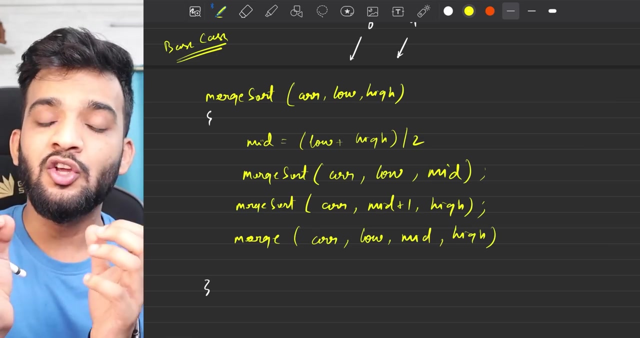 we have to write that over here, because if you know if this is nothing but a recursion- more short calling itself, more short calling itself- it's a recursion. in order to stop recursion, you write something as base case. i hope you know that in order to stop recursion, you write something as base case. so i have to write that beast case. let's analyze. 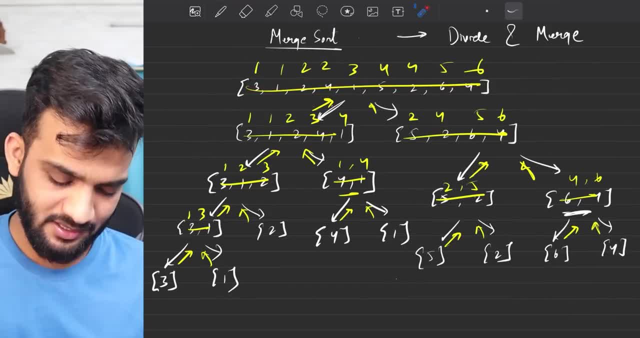 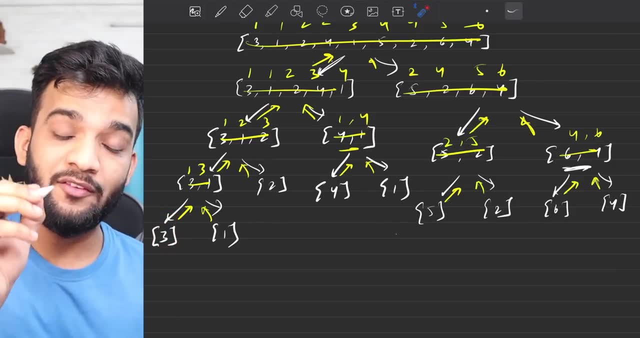 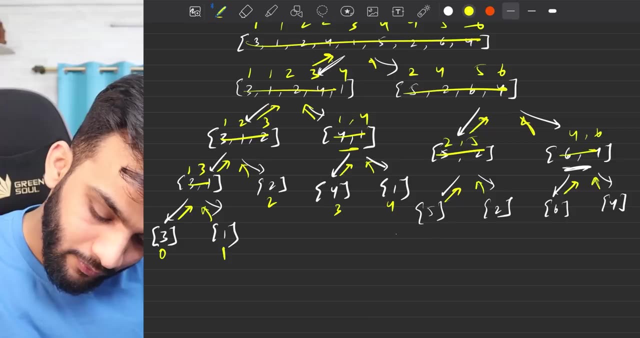 what is the beast case? let's go back to this example. what is the beast case, can i say, when your array has one element? when your array has one element, so if i have to index it, can i say: this is zero, this is index one, this is index three, two, three, four, five, six, seven, eight. can i say these? 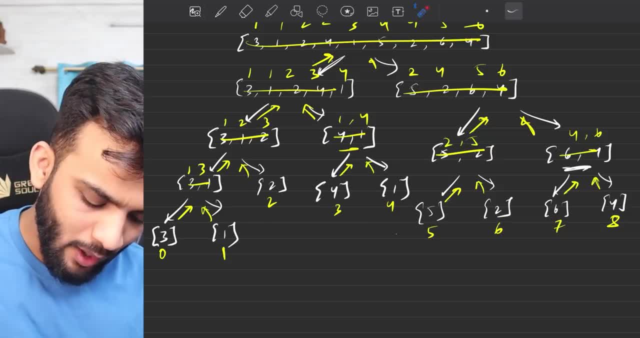 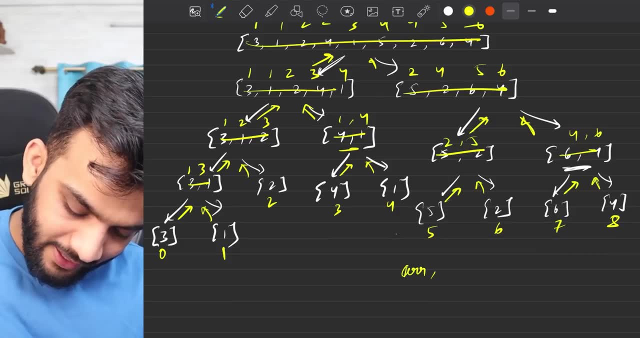 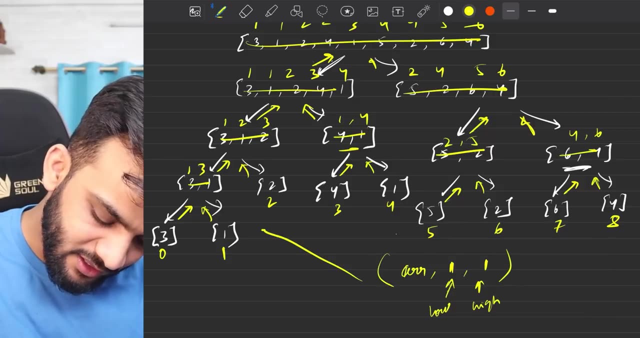 are the last indexes. and if i have to ask what array is this, you'll be like. this array is something like from index one to index one, where index one is the low, index one is the high. can i say this is the array that represents this? yes, because we are not creating a new array. i am 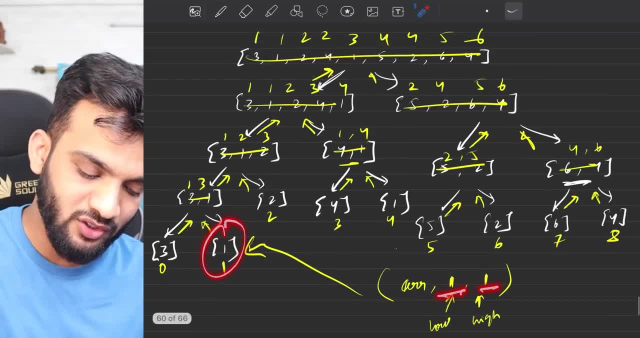 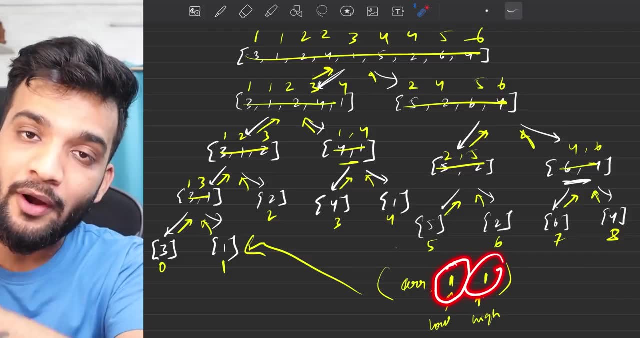 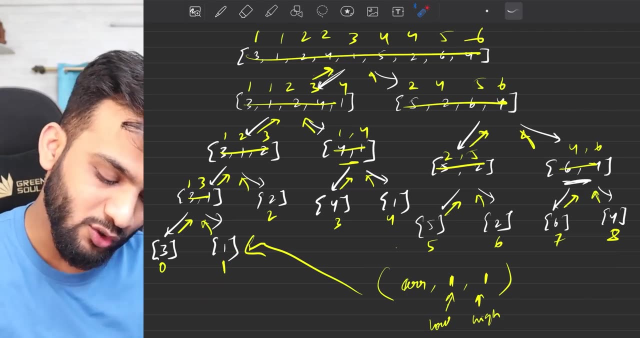 saying this array is from index one to index one. which is this right? so can i say: the moment we have the low, the left point, we have the high, the right point, to be same, that's when we do not go and divide. we do not divide, we just go back. so that's what the base case will be. we write: 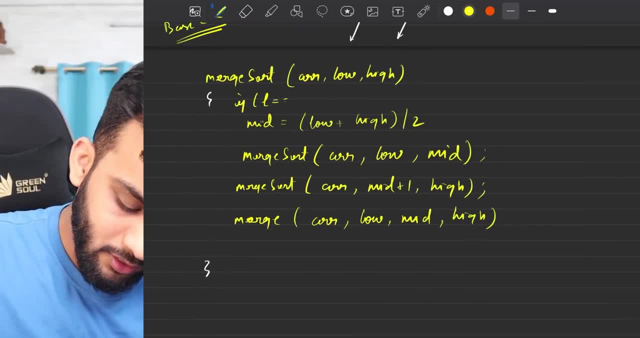 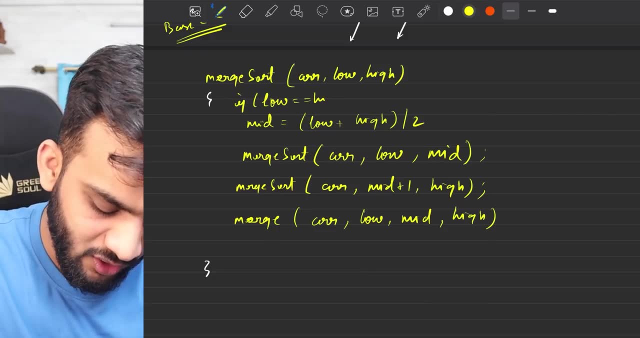 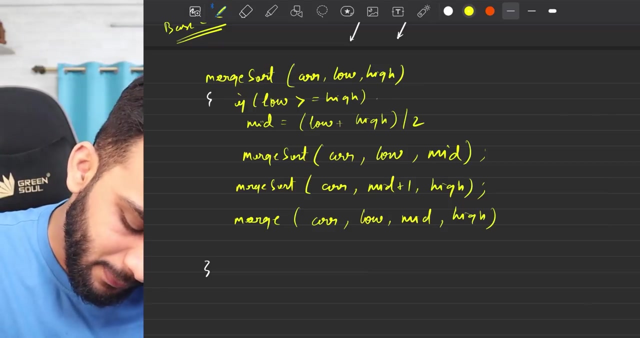 hey, if at any moment the low tends to be equal to equal to high or exceeds high for that reason- or maybe it's some how like it will never, but still there's no safety reasons. if it exceeds high, please do not, because there's no need to do any of the further algorithms. it's. 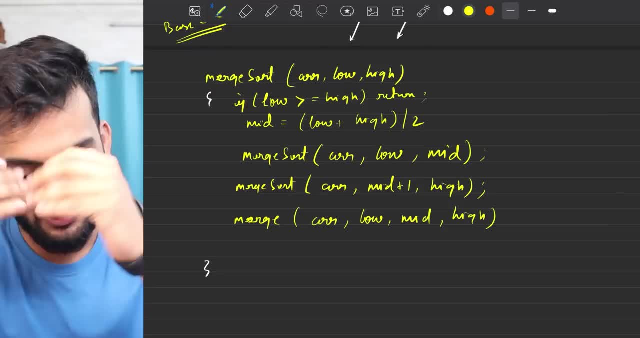 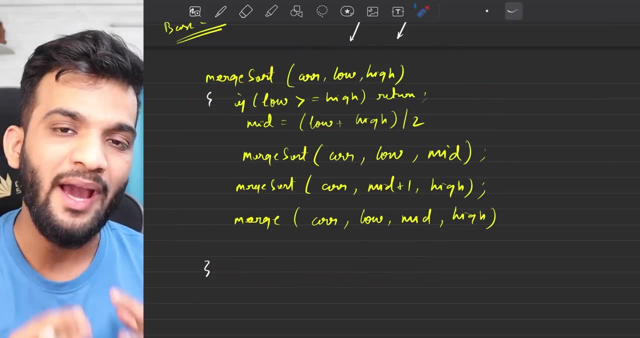 a single element array and it will always be sorted. please go back. please go back. so this is how the pseudo code will look like. might seem a bit confusing, but now when i'll write, and by taking an example it'll straight away get to your head. okay, so we can say that the pseudo code has been. 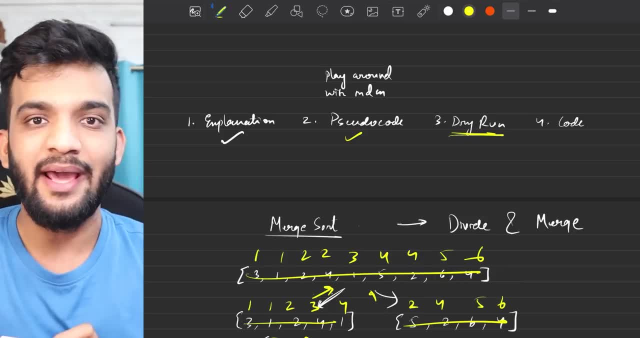 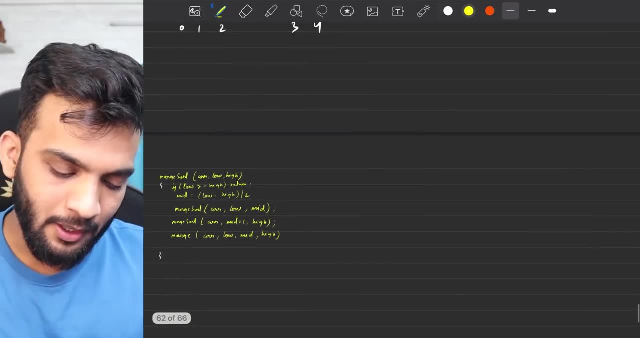 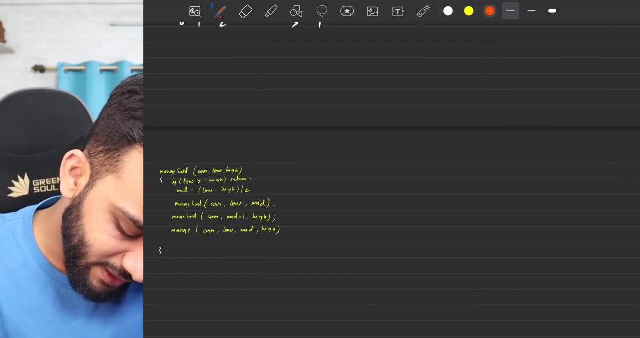 sorted. so let's try to understand this algorithm with clarity. we have to do a dry run of this recursive algorithm, then only it will get clarified. so let's try to do a dry run by taking this particular example. so remember one thing: whenever this algorithm is called, it is called with the. 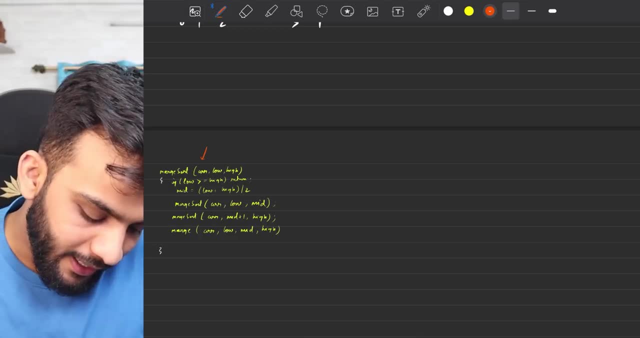 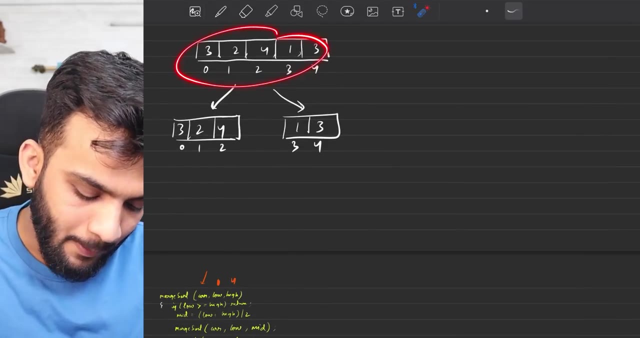 complete array. so the entire array has always been passed with this algorithm and the initial low and high will be 0 and 4, because that's what for this particular example it will be, because initially i had the property of mid and i set it to mid. so i go back to my algorithm, so i will take the value of 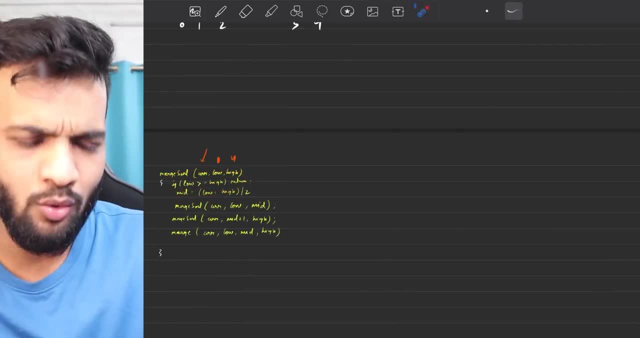 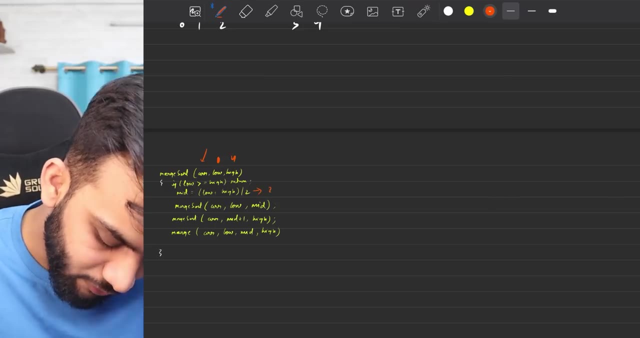 the value that i have, and i'm gonna require a value of short and i'll use the value of mid. so if i'm going to call it mid, this will be the value. that will be the value of mid, which is 4, so i'll execute the apples, all right. so now, if i'm doing the same thing, i'm going to go to my 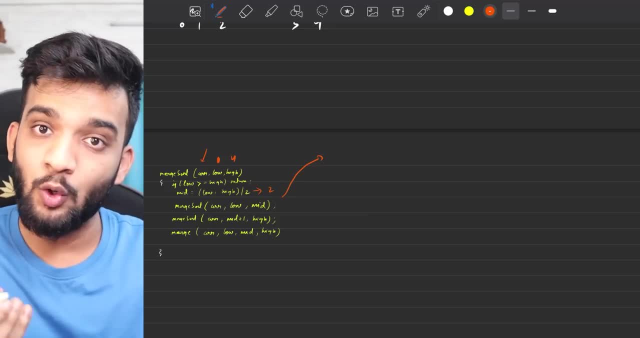 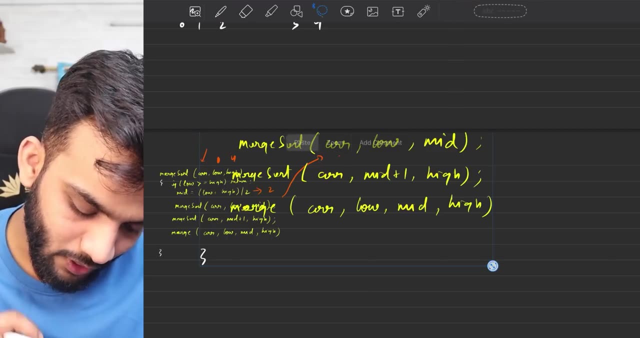 array. i'm just going to select the first base case and this is the first base case that i'm going to operate this time. so i'm going to place on this entire array and ask my shot to sort it. so what will happen? will this first base case operate? because no low is still smaller than high, so it doesn't. 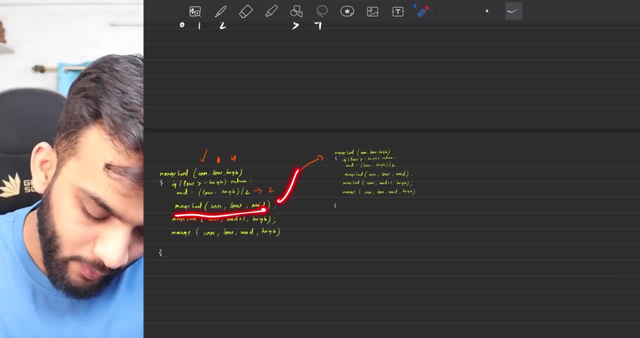 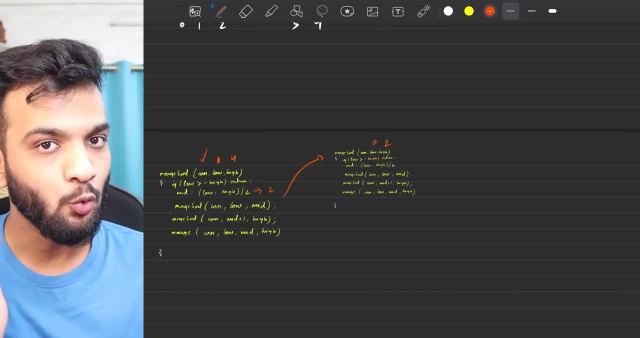 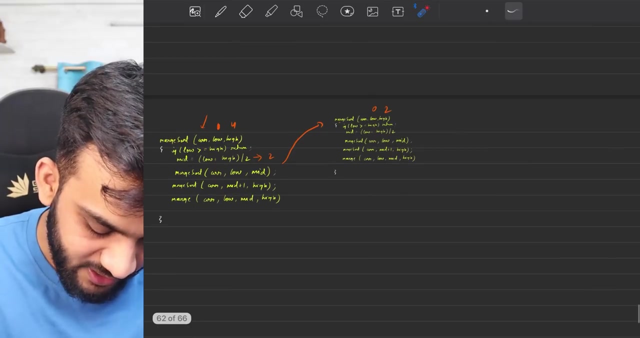 so what we can say is: this particular recursion call will call this particular function again, but this time it will pass the low as 0 and pass the high as 2. so apparently what happens is it calls for this guy. remember how recursion works is: first, this will get operated, comes back then. 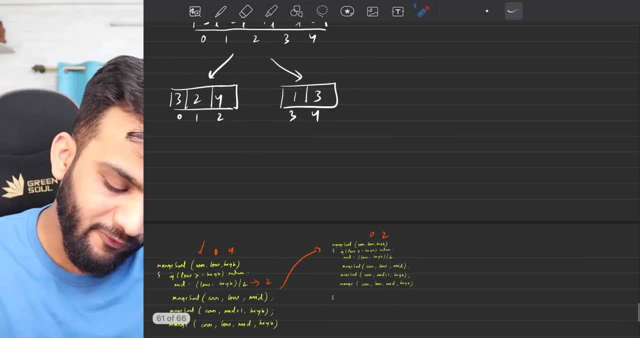 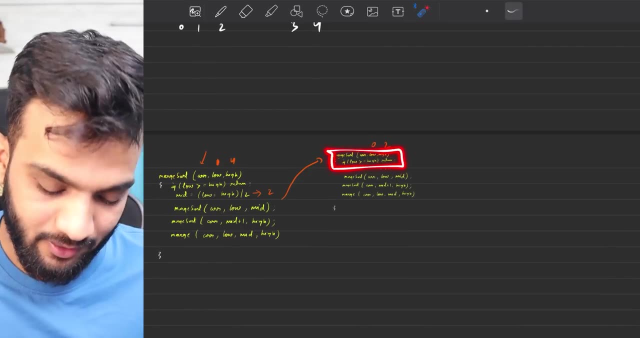 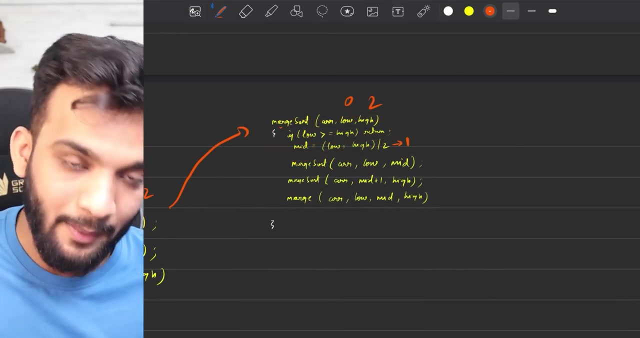 this line gets operated. that's how recursion works. so that's why first the left portion will get operated. so the recursion call for 0 to goes. now what happens? does this line operate? no, this line doesn't operates. what happens tries to find the mid, and this time the mid comes out to be 1. 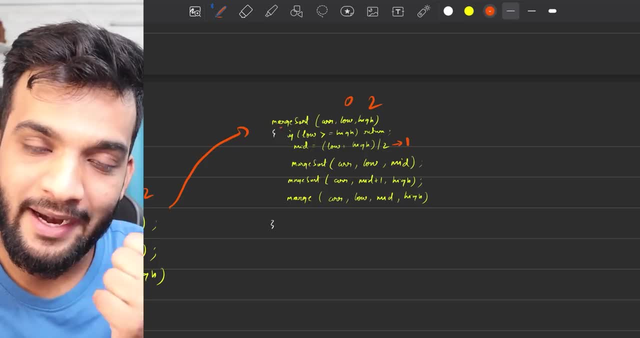 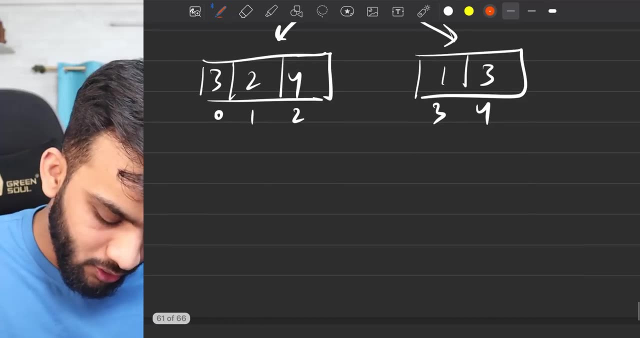 because 0 plus 2 is 2, and 2 by 2 is 1, so 1 comes out. so this time again, this merge shot gets called. but if, if the merge shot gets called, what will happen? it gets called for what? from 0 to 1, so 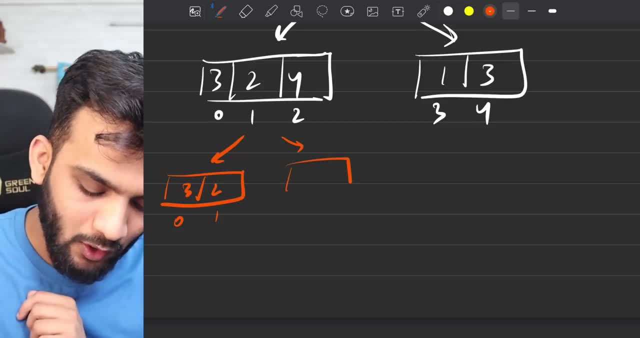 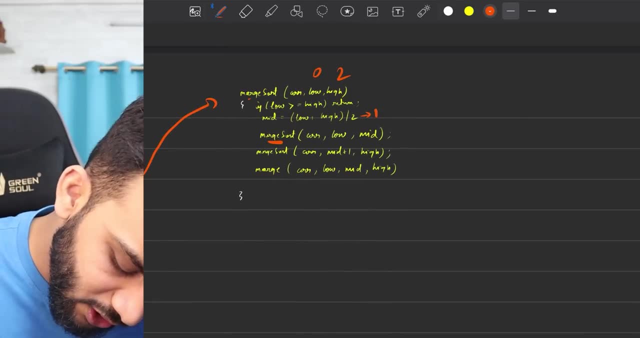 it's like 3 to 2 is what it is getting called, and then it will be called for the only number, 4, which is just 2, so we will go ahead and maybe again call this recursion. it's go ahead and call the recursion again, so the recursion is again. 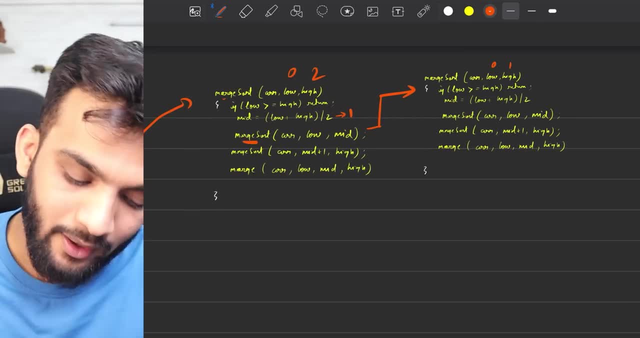 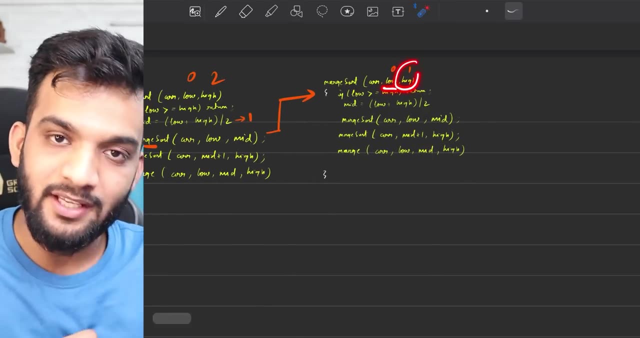 called. what happens this time? the merge shot is called with 0, 1, which means this particular example, right? so this time the low is 0, the highest one. so what happens? the mid is 0 plus 1 by 2, which is nothing about 0. so again, 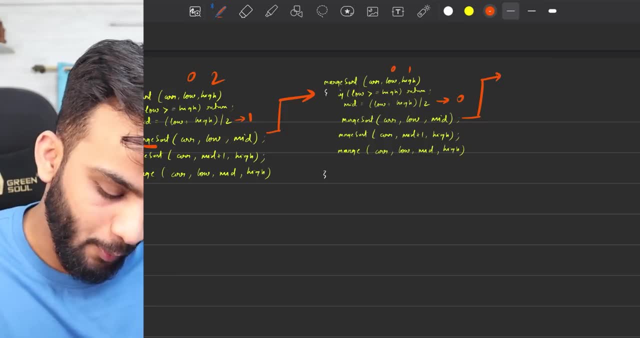 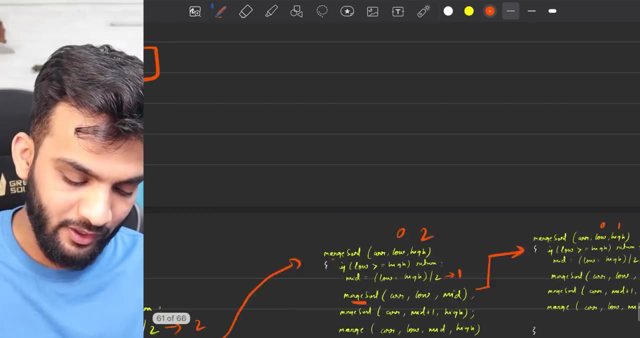 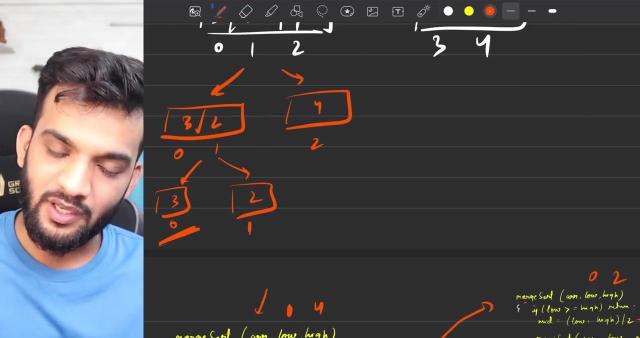 the merge shot is called, so let's again copy paste this same algorithm. the merge shot. this time is called for zero, zero. if i go into the diagram, it's something like for three and something like for just one, so this time it's called for three. so what happens is it's called for zero and zero. 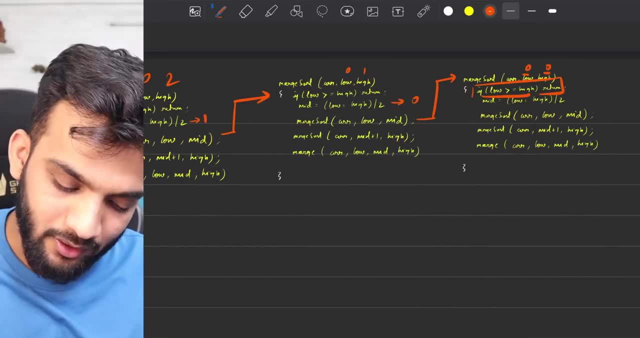 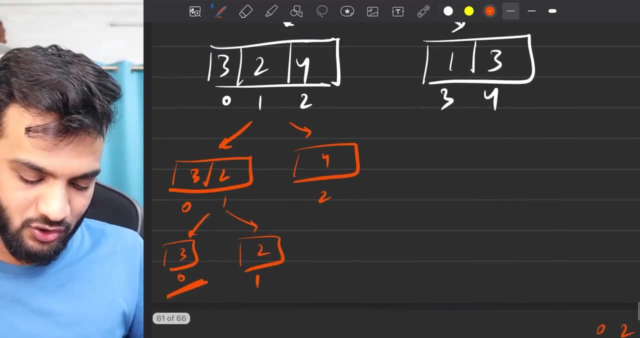 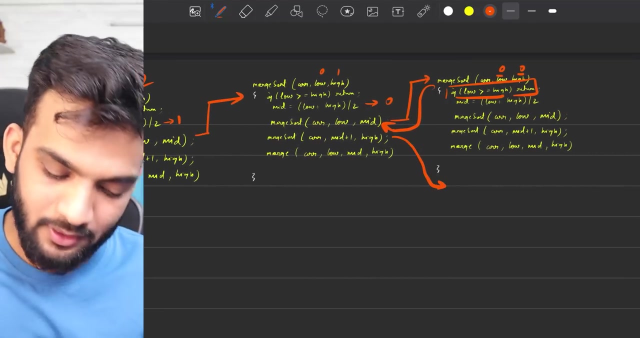 so apparently this particular base case gets executed and it returns, so i can say them: it's done, it's done. so if i have to go back into the chart, this goes back. similarly, another merge shot will be called- let's try to write this as well- and this time it will be called for. 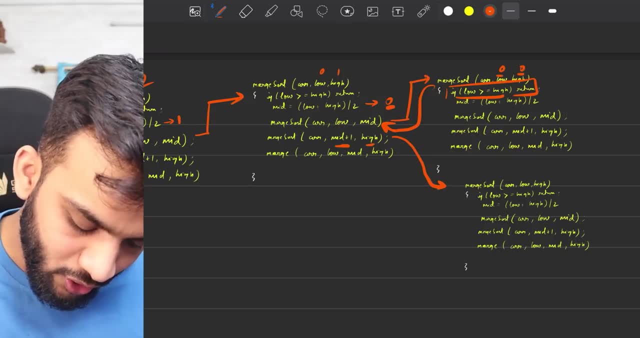 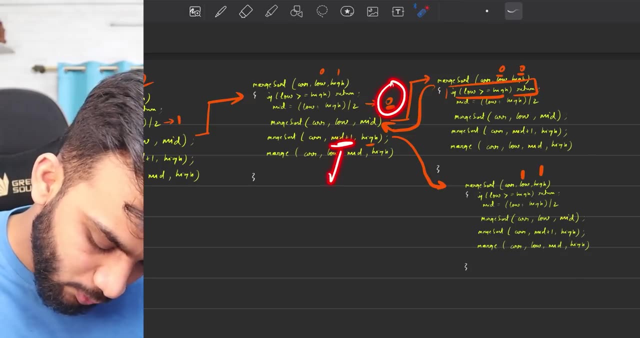 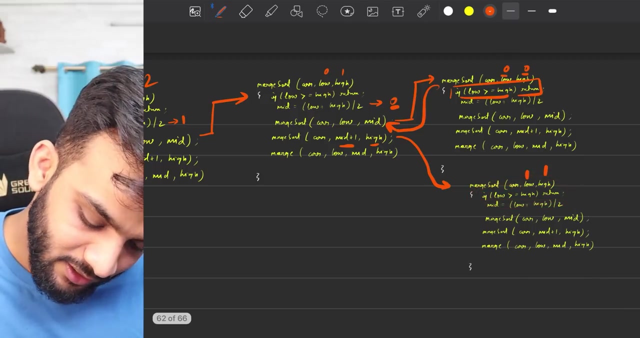 from mid plus one to high. so mid was zero. so it'll be like one comma one because high was one, mid was zero, so mid plus one is one, high is one, so high is one. it's called for one comma one. again the low, the base case operates and it calls back apparently both of these recursive functions. 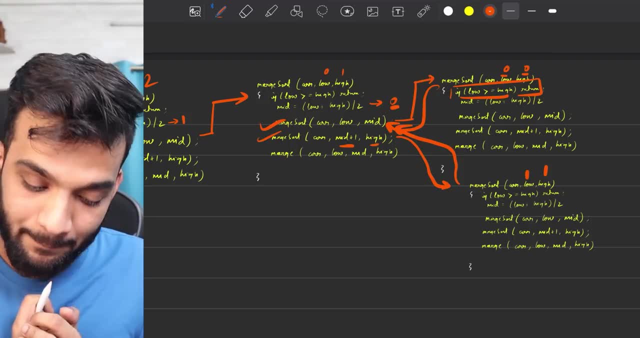 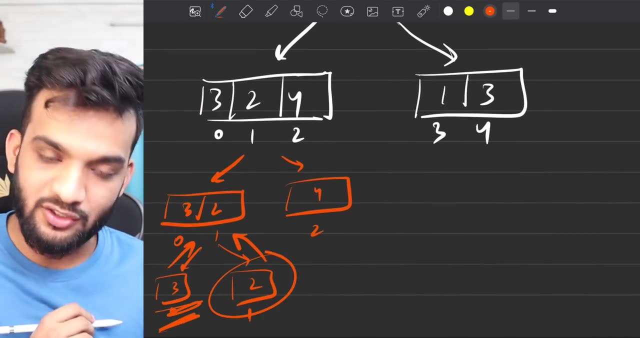 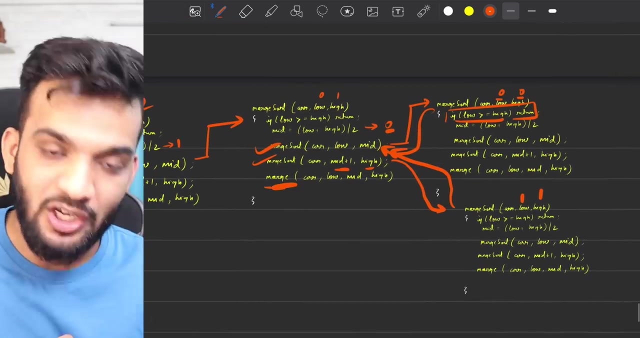 are completed. once both of these recursion functions are completed, can i say this that i'm going back from here and now. we have this as sorted. we have this as sorted. it's two sorted arrays. it's two sorted arrays. what will happen? let's go back here. this merge happens, so it takes. 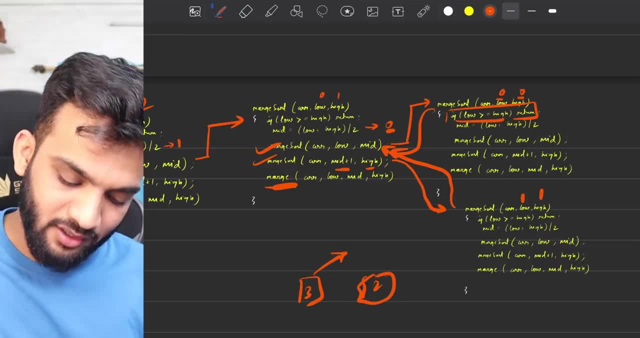 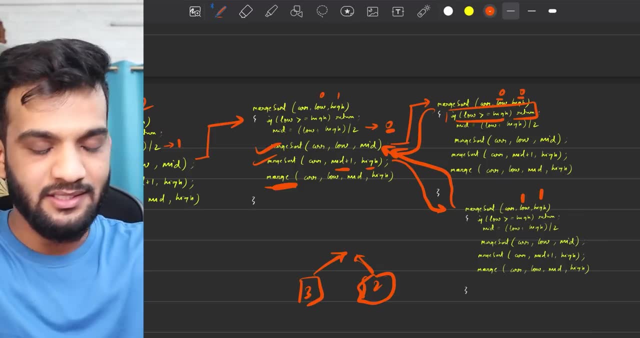 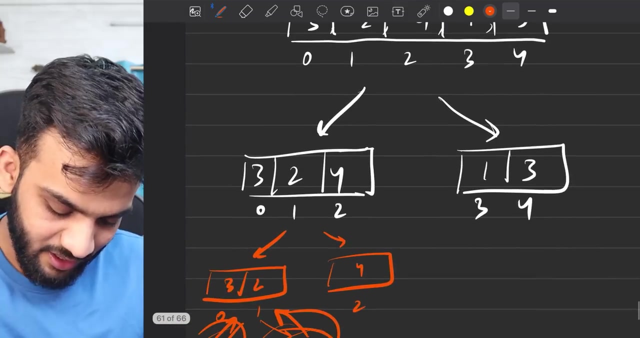 a 3, it takes a 2 and it tries to merge it. now we will write the merge algorithm afterwards, but let's understand. just imagine merges merging two arrays. that's it. that's a very simple algorithm. just understand this. so 2 comma 3 happens. so what would have happened? 2 comma 3, right? so this would. 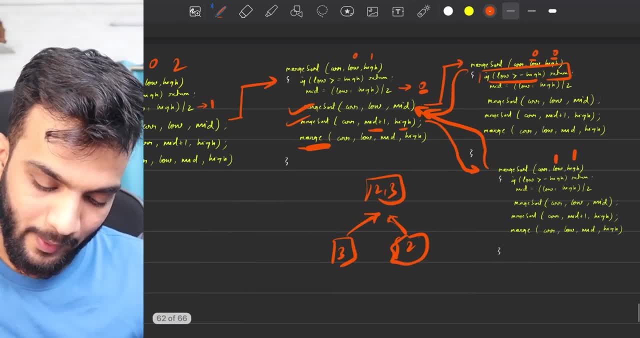 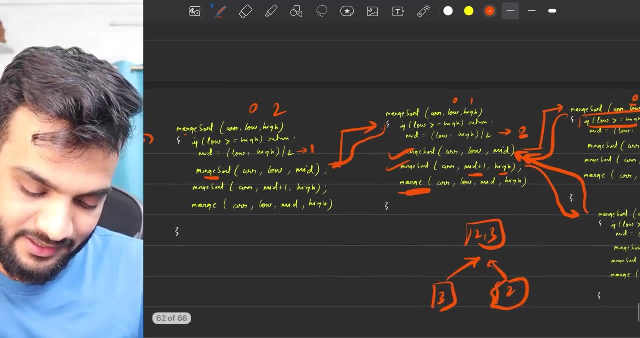 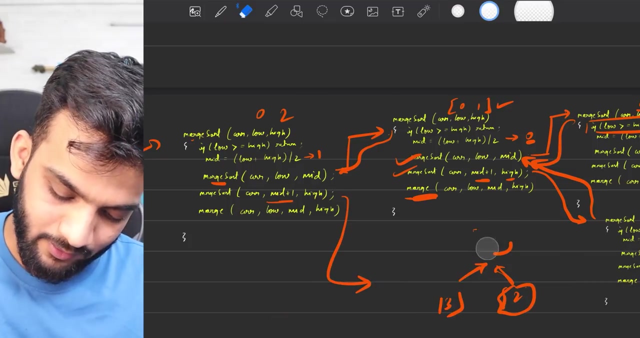 have become 2 comma 3. perfect, let's go back to the recursion. so can i say: now we can go back from here to here and we can say the 0, 1, 1 is sorted. so this time this recursion will again be called. let's try to write it. so what will be? 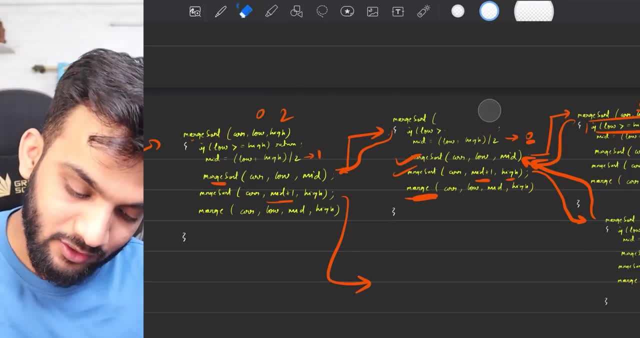 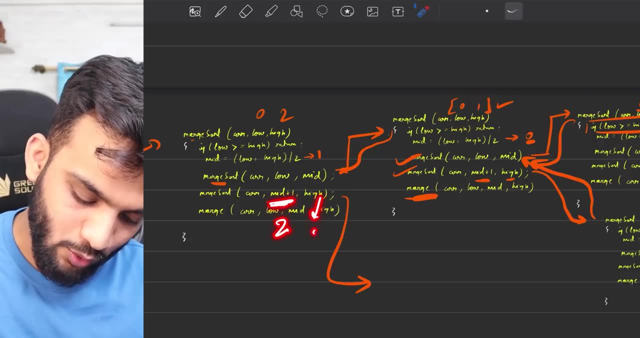 this recursion: if 0- 1 is done- sorry, my bad- if 0, 1 is done, what's the next mid plus 1, that's 2, i is 2, so we'll call it for 2 comma 2. and if we call it for 2 comma 2, what will happen? yes, they. 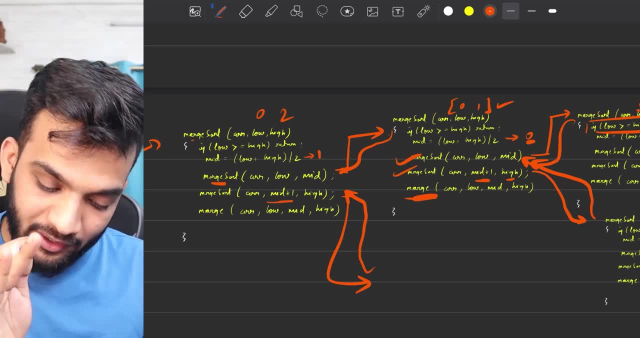 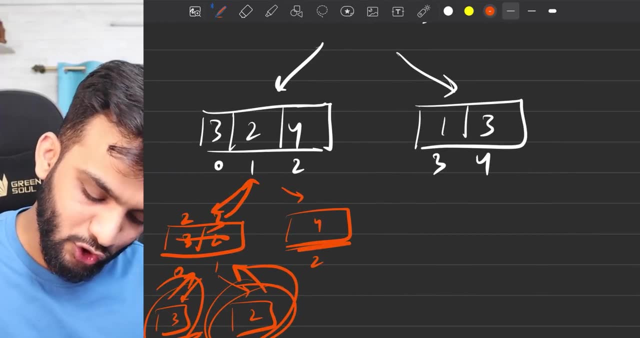 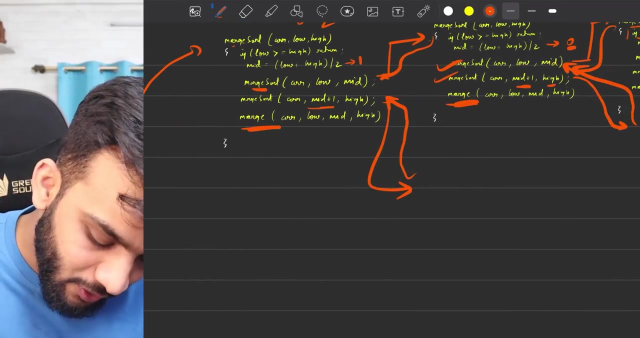 are the same numbers. so it will return. and if it returns this time, what will happen? it called for 2 comma 2. this guy has done the recursion and this guy has done the recursion. so apparently, again the merge happens. this time the merge happens from 0 to 1. 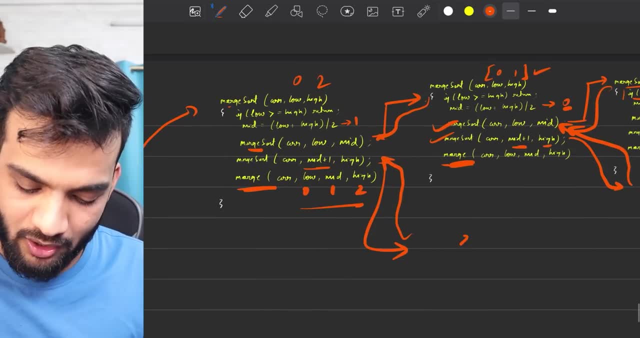 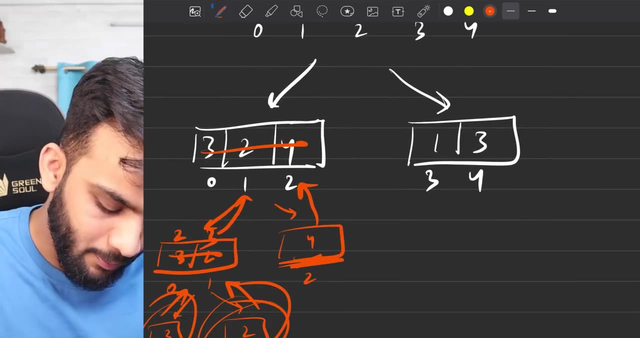 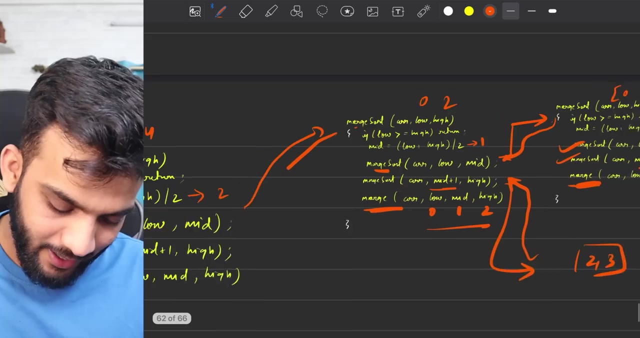 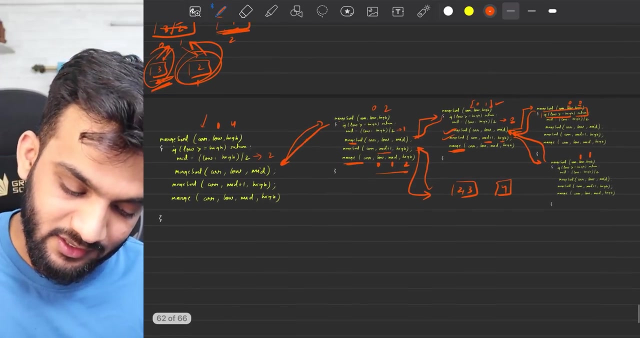 till the 2. the merge this time happens for 2 comma 3 and maybe 4 or whatever it is. yes, and this will become 2 comma 3 comma 4. i hope you are getting the gist. so can i say, after this i'll again go back, and when i go back now i'll try to just come back. yes, when i go back, can i see? 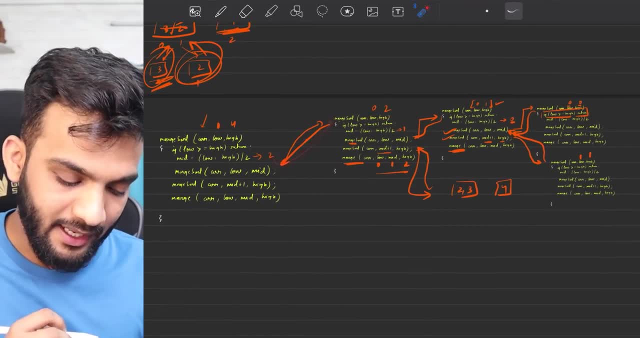 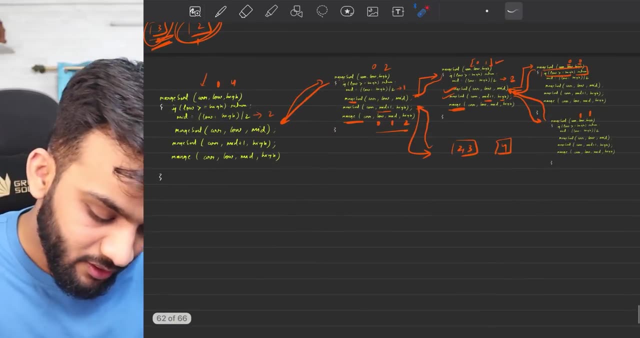 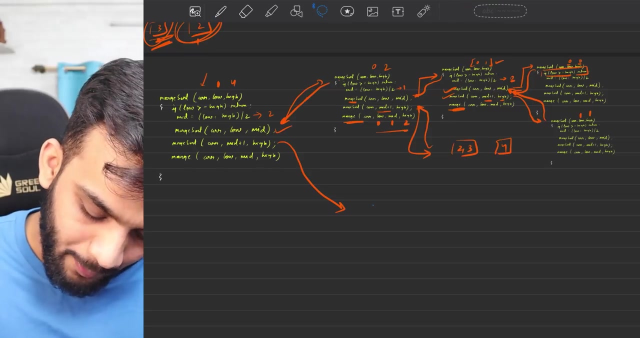 this, that 0 comma 2 would have been sorted. and if 0 comma 2 is sorted, i'm done with this and i'll go to the right part, which is having this and similarly. this is done, so this will call it right. and how will it call it? let's copy paste and show it if 0 comma 2 has been done, so. 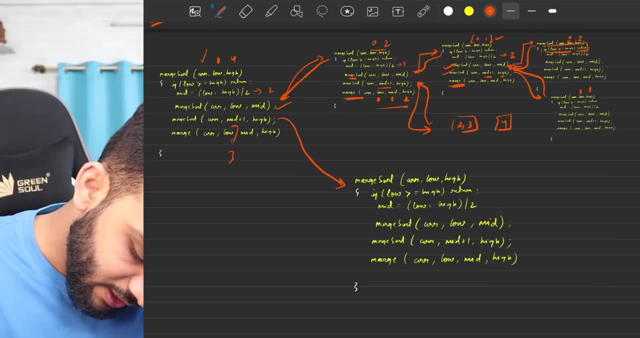 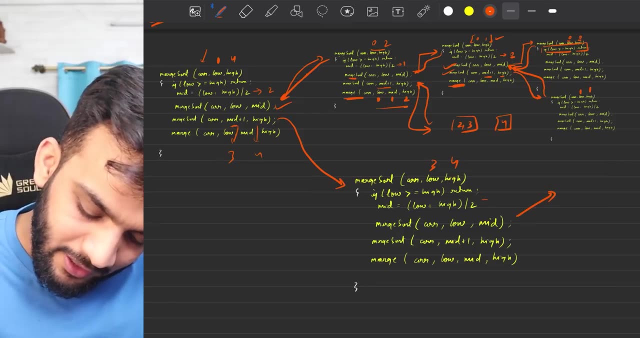 can i say? next is mid plus 1. so this is nothing but 3, highest 4. this time it goes and calls for 3 comma 4. again, the same thing will happen. the mid will be like 3 plus 4, 7 by 2, 3. so it'll be. 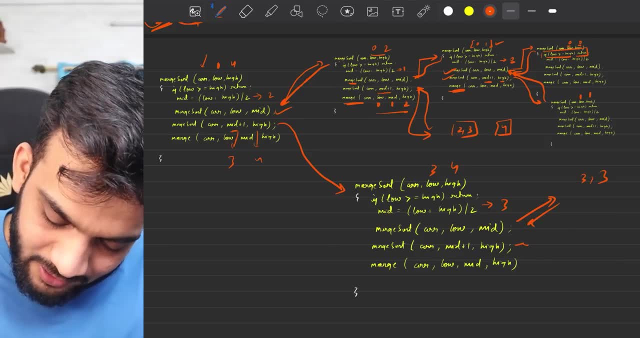 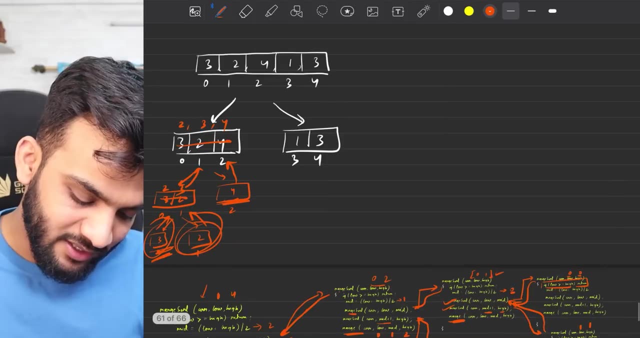 called for 3 comma 3, and then it'll come back. this will be called for 4 comma 4. it'll be come back and then this will merge both of these two elements. it's like it'll be called for 1, it'll be called for 3, then they will be merged as 1. 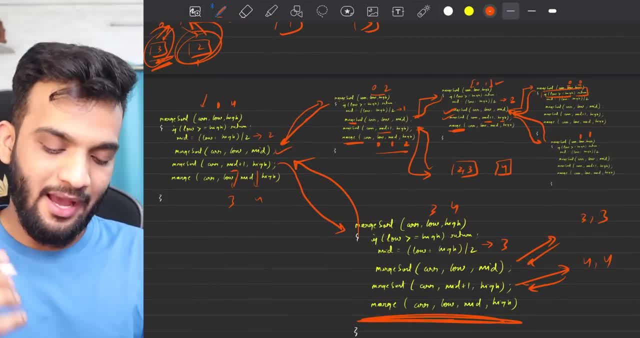 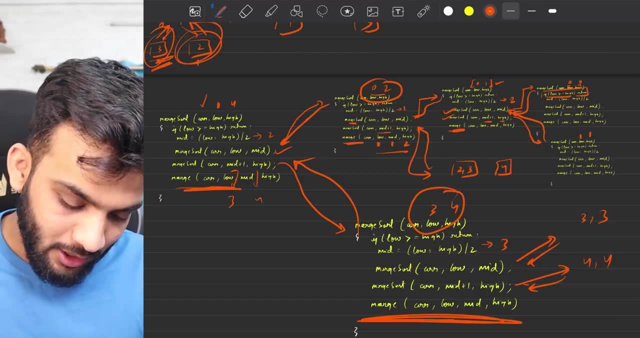 3. and once this is done, what do we have? we have 0 comma 2 sorted. we have 3 comma 4 sorted. so the last merge takes place between this 0 comma 2, that is, 2 comma 3 comma 4 and 1 comma 3. 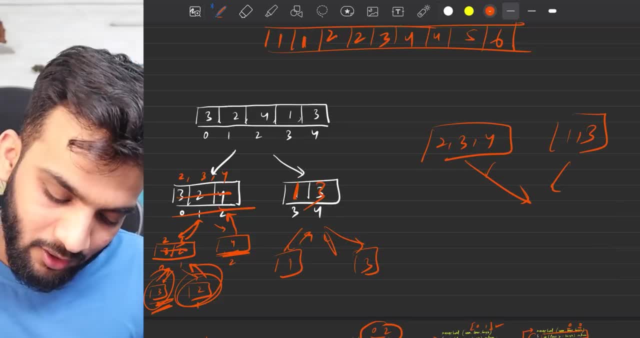 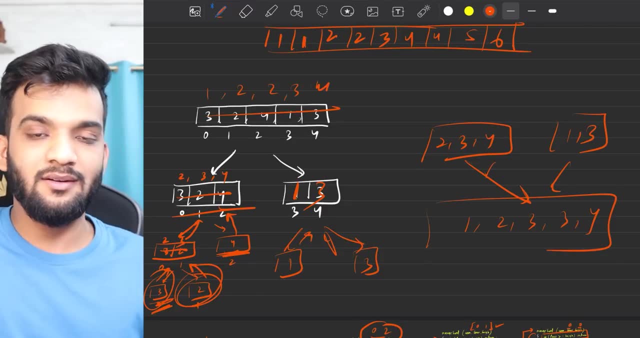 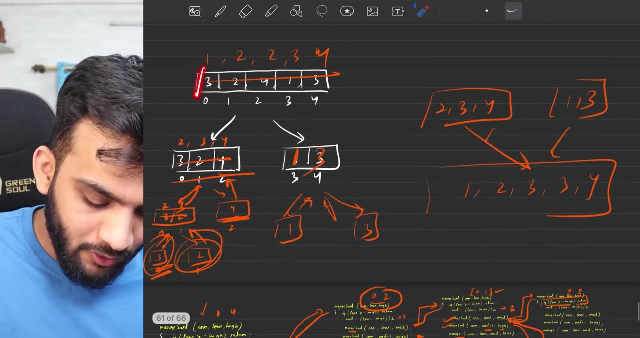 so apparently they are merged together. when merged you will get 1, 2, 3, 3, 4. that is what happens at the last step. i hope that does make sense. so so i hope that viran is clear. in terms of the pseudo code, it was very simple. first, the entire array goes to the left. 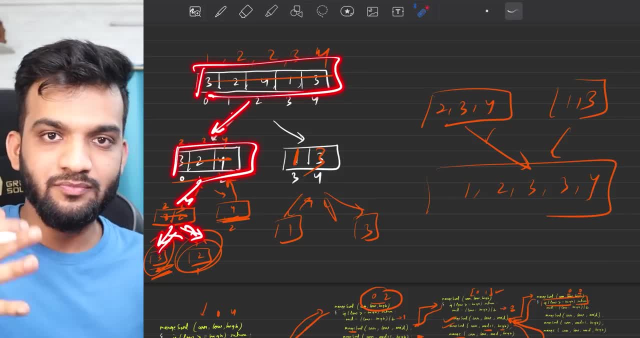 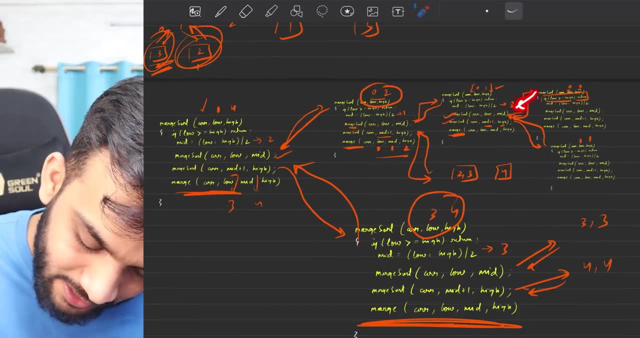 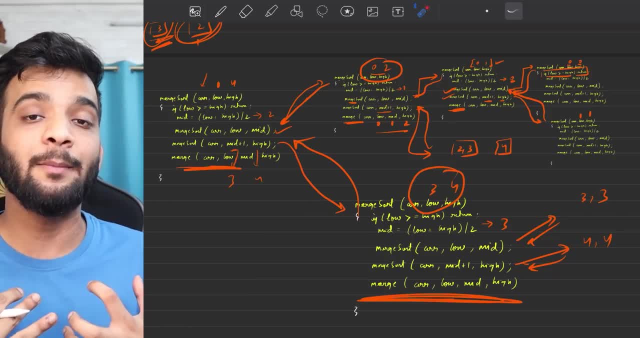 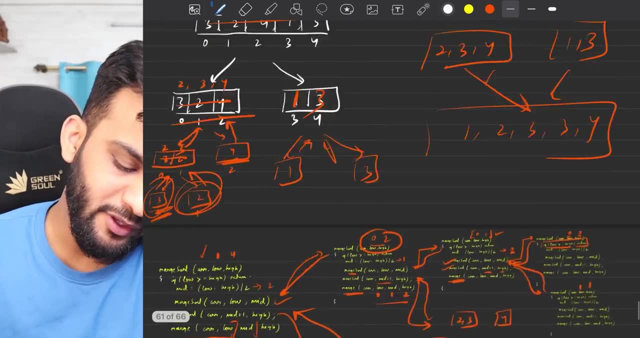 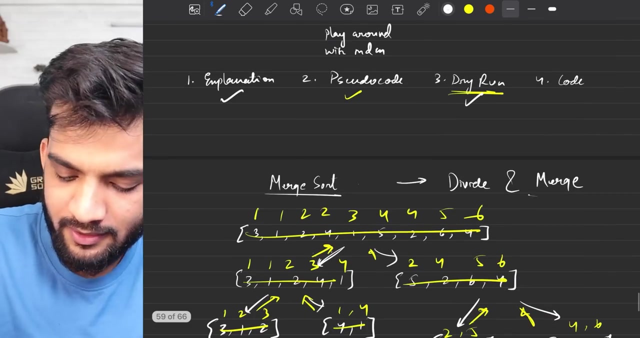 in order to understand this in much more depth, what i'll recommend you is: take a pen and paper, write this code. try doing it all over again. got it? so what have we completed? we have completed the dry run, the pseudo code as well, but before going into the code, we still are left with the merge. 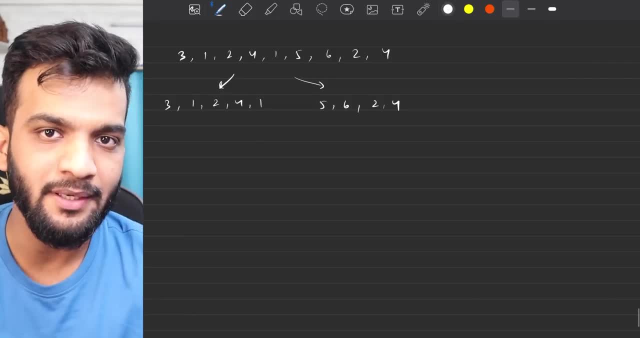 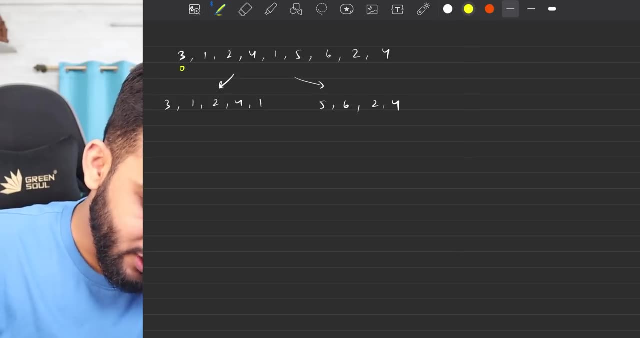 pseudocode. if we are able to write the merge pseudocode, i think we will be done. so let's take a bigger example in order to understand the merge pseudocode. can i say the indexing is like 0 to 3, four, five, six, seven, eight, and this is like zero. one, two, three, four and this is like 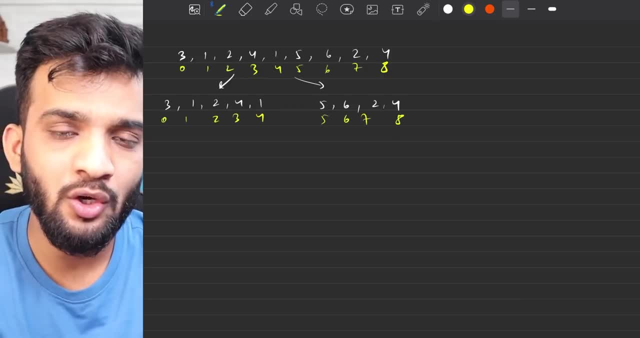 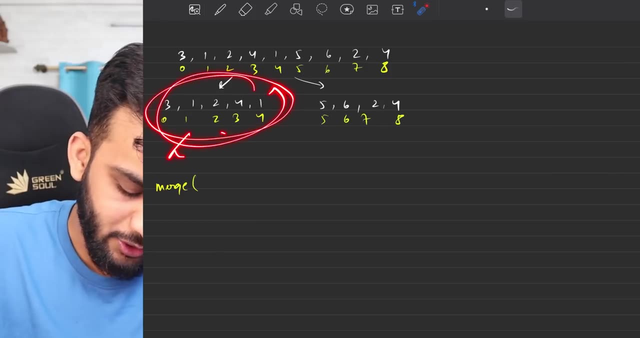 like 5,, 6,, 7, and 8.. And if the merge will happen, I will call it like: merge these two arrays, because if you know this array, when goes into depth, goes into depth, it will be sorted. 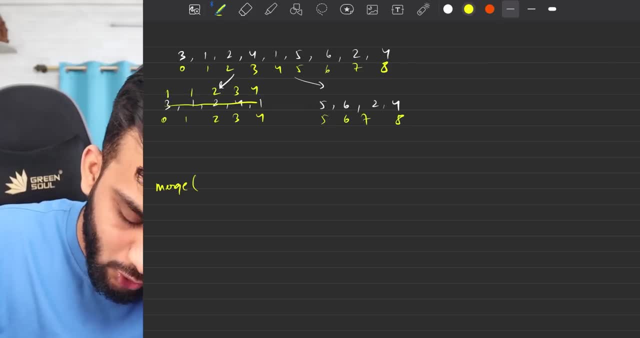 It will be sorted like 1, 1,, 2,, 3,, 4.. And this also will go into the depth, and it will be sorted like 2,, 4,, 5, 6.. This is something which all of us know for sure. 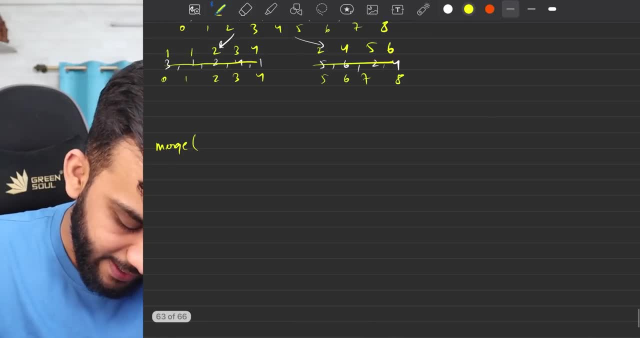 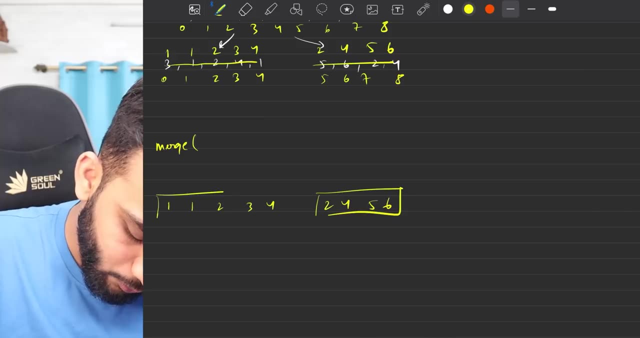 that both of them will be sorted And both of the array will be something like 1, 1,, 2,, 3,, 4.. And this will be like 2, 4,, 5, 6.. This is something we know. 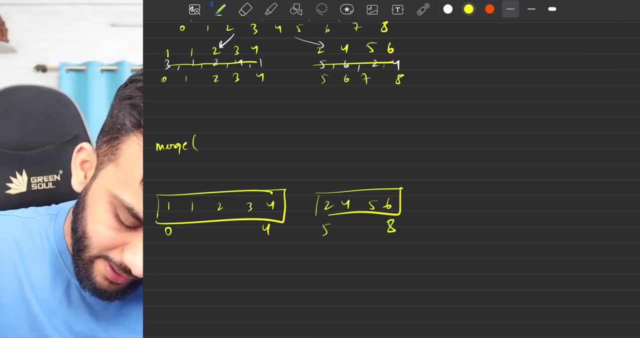 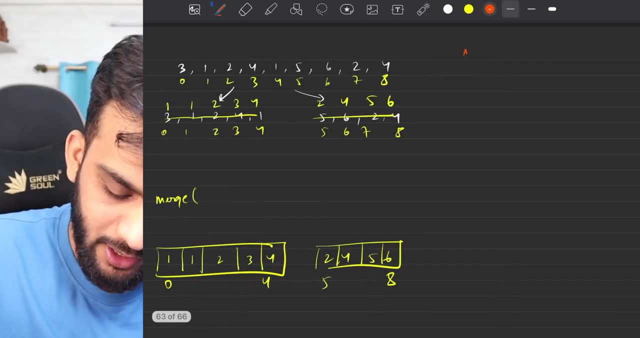 And this will be indexed from 0 to 4.. This will be from 5 to 8.. That's something we know. We just have to write an algorithm to do it. So we are writing the algorithm, So we are saying merge. 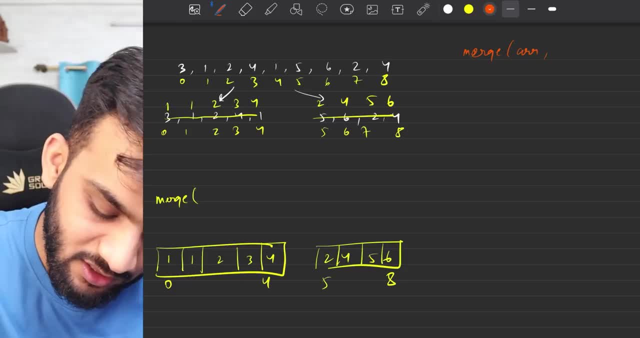 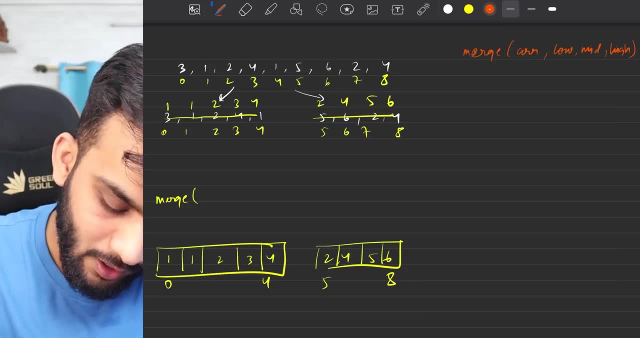 I will give you the array and I am stating you that the first half is from low to mid, and then you can go from mid plus 1 to high. So I am giving you all the three parameters required. What I will do is maybe I will just keep an empty data structure. 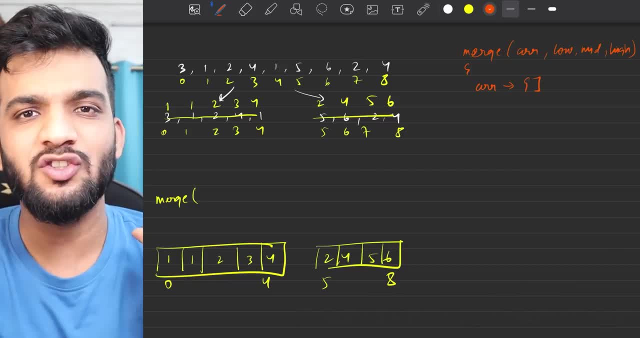 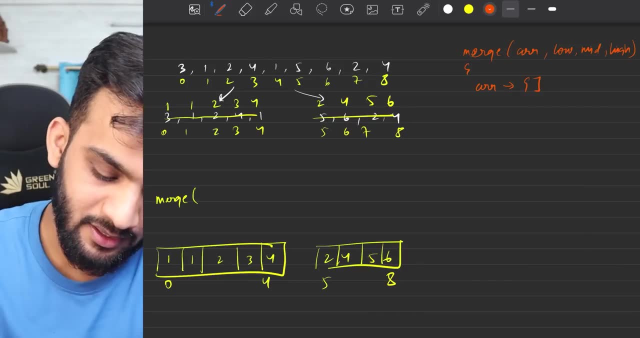 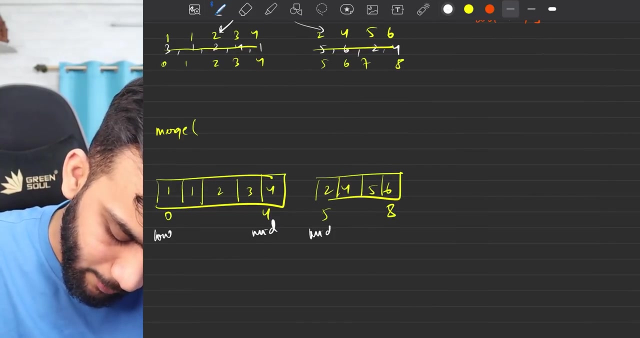 It can be a vector, It can be a list, As of now. just imagine this is an empty data structure where we can add elements. Now can I say that the left array will be from low to mid, And can I say the right array will be from mid plus 1 to high? 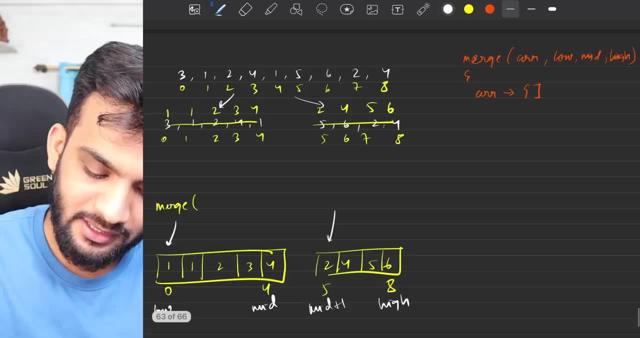 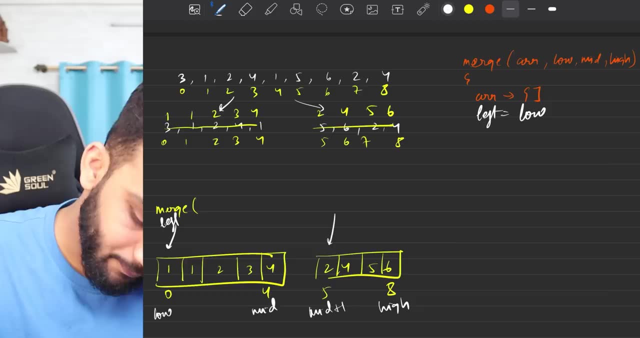 I can. So I will keep a couple of points. So I will say, okay, left pointer is at the low, So that means left comes over here. And I will say, right, pointer is nothing but at mid plus 1.. 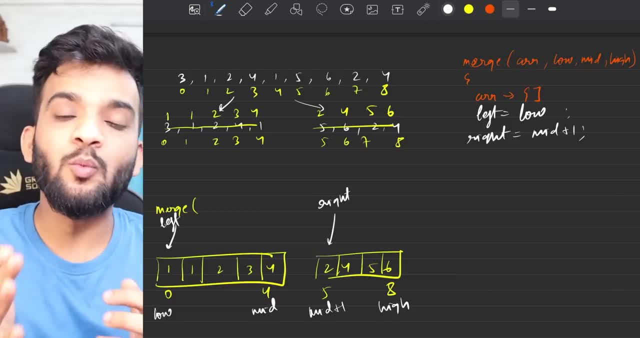 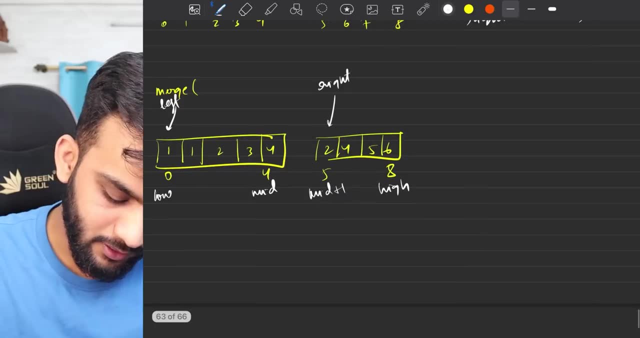 So what happens? I will say: right is here. Now what will I do? I will try to compare these two and try to fill in this bigger array, The bigger array. I will try to compare these two and try to fill in the bigger array. 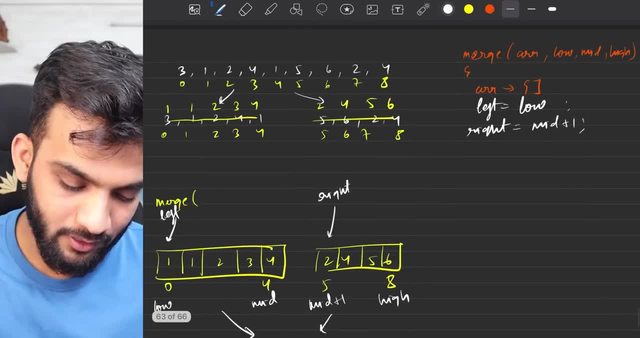 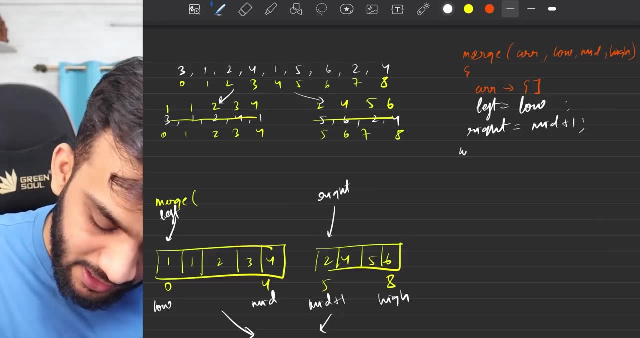 So what I will do is I will now. I will now try to iterate Till what? Till we have elements on the left or till we have elements on the right, Can I say? That means I will say: while left is smaller than equal to mid. 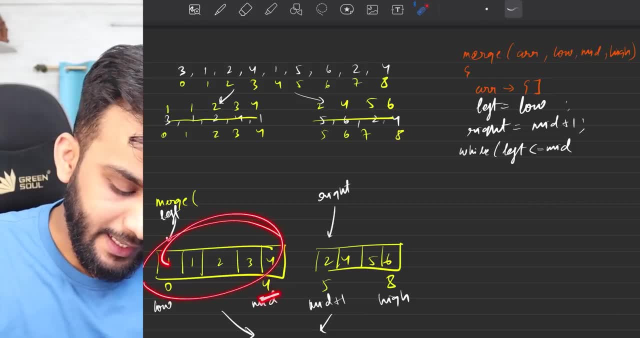 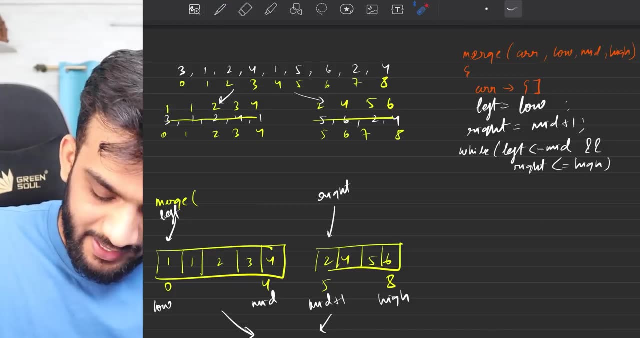 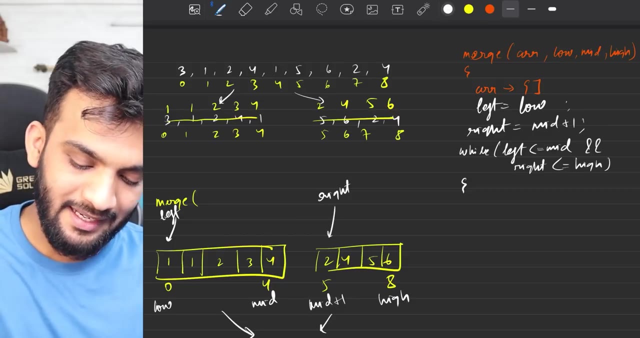 which means I still have element, and I will say and, and right is lesser than equal to high, which means I still have elements on the right. Very simple, Now. what I will do is: okay, this is what I will do Till I have elements on the left. 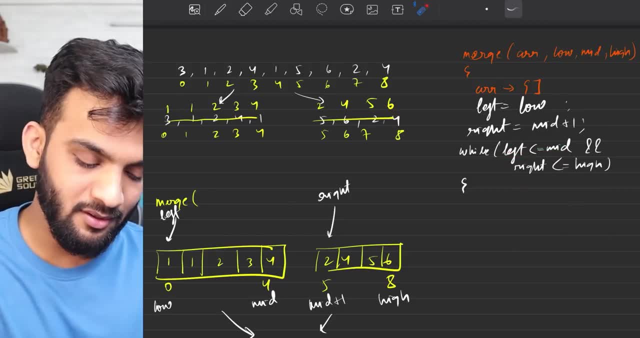 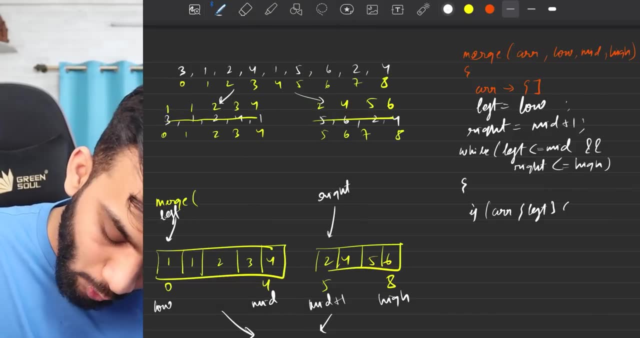 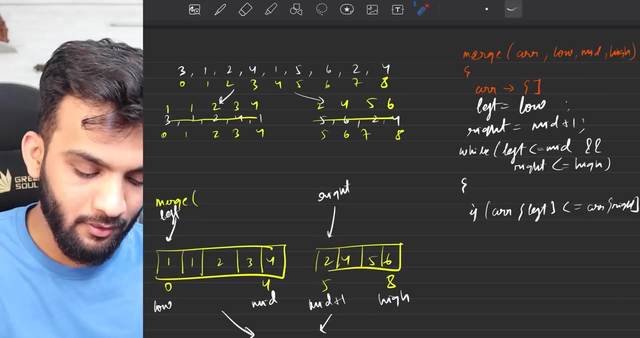 elements on the left. they'll have elements on the left, on the right. so i'll now try to compare. i will say: hey, listen, if array of left is smaller than equal to array of right, so what happens? this and this gets compared, and if one is smaller than two, i'll take one and i'll 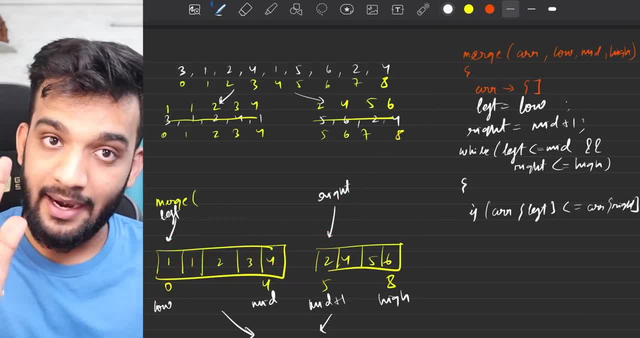 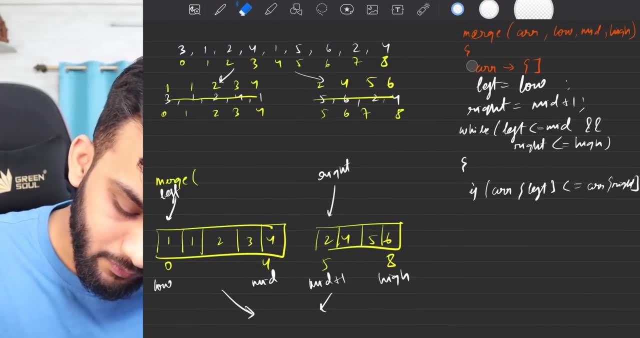 add it to our resultant guy. i'll add it to our resultant guy, so i'll say: okay, maybe we can name this as something else. let's go and name this as. maybe let's say temporary, that's a better name. as a temporary, can you please add yourself the smaller guy array of left, and once you have done, 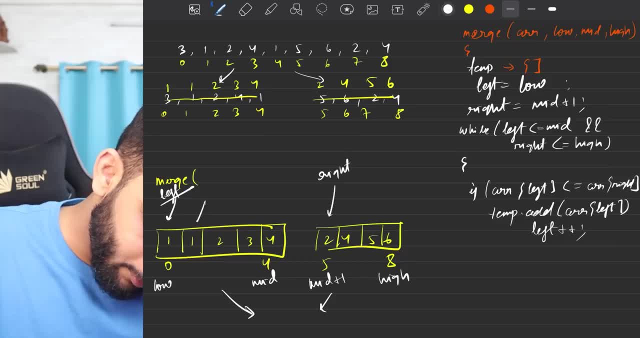 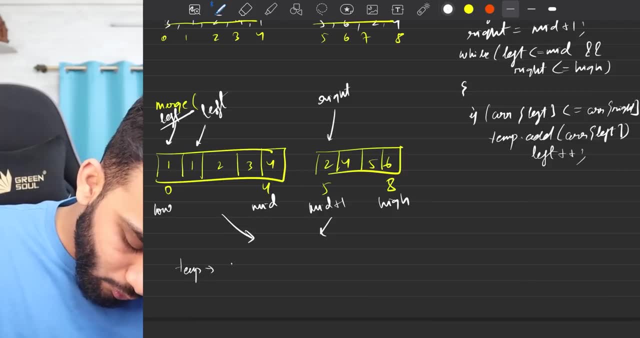 this can you move ahead. the pointer, which means the left pointer, goes to the next again. so basically what will happen is now temporary will have one with itself, again the comparison between one and two will happen, and this one will come here. so temporary again takes it and now the left moves here again the comparison between two and two will happen. 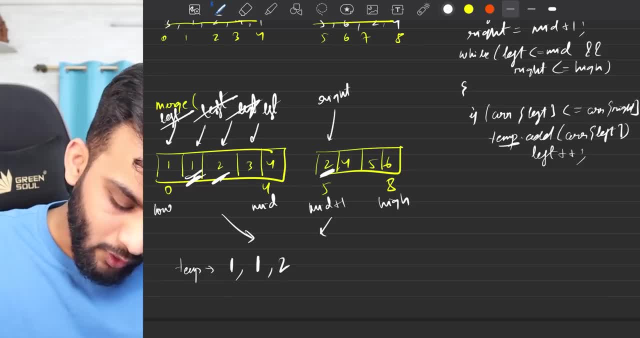 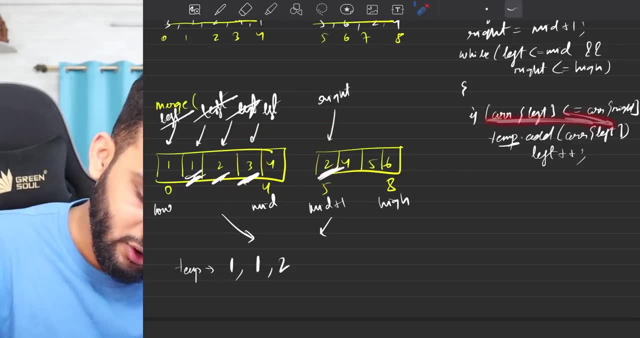 and it comes here and the left moves here. this time, when you compare three and two, when you compare three and two, the two will come, but the if only compares for lesser. so there will be a else. else will state: can you please add the right guy? can you please add the right guy? that is. 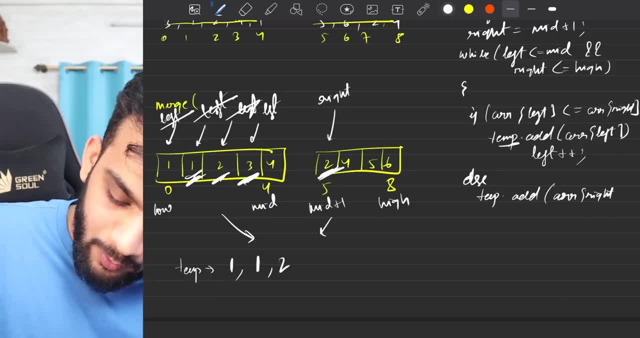 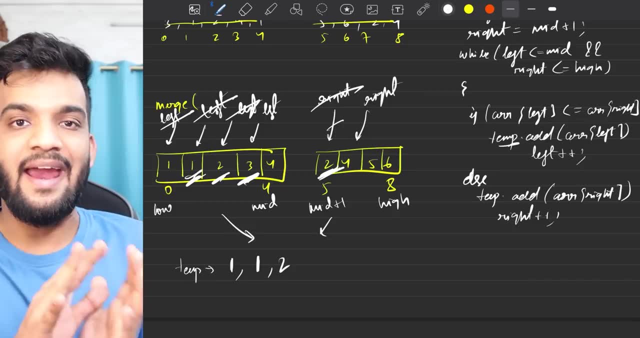 take from the array and add the right guy, and once you have added, can you move the right plus plus. so what i'll do is i'll move the right to ahead. now, that's how this will work, and you'll keep on comparing and you'll keep on adding. 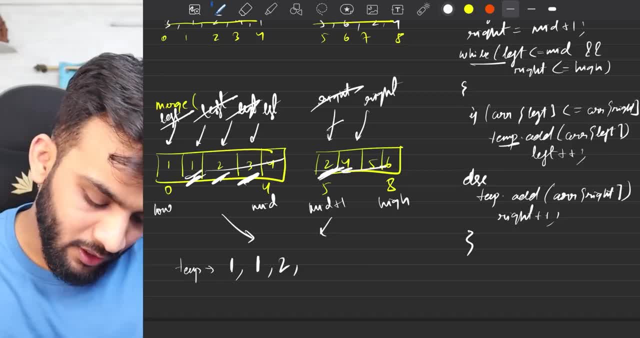 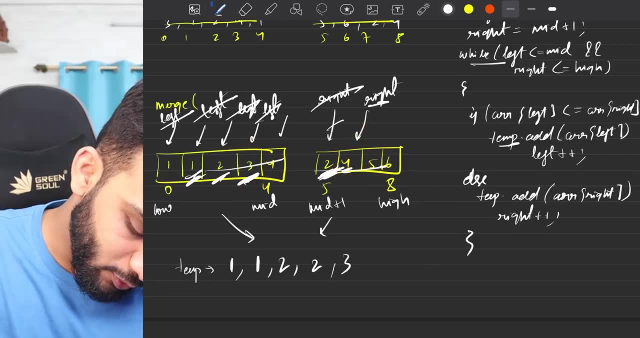 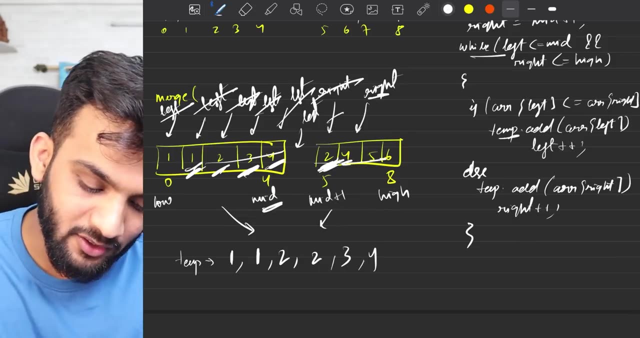 till this is not completed. so what will happen this? two will come and the right will move. here now the comparison between four and three happens. so three comes and the left moves here. now four comes and the left is exhausted. left exceeds mid, left exceeds mid. so we see that the left has to be. 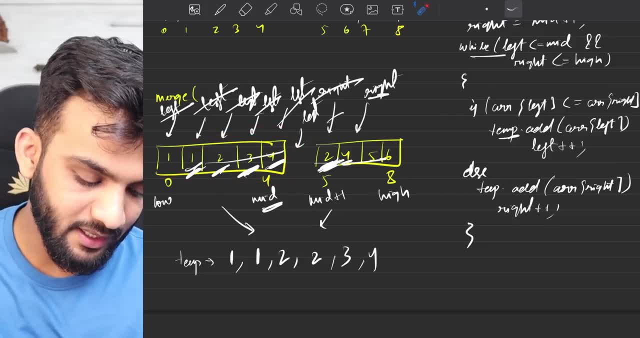 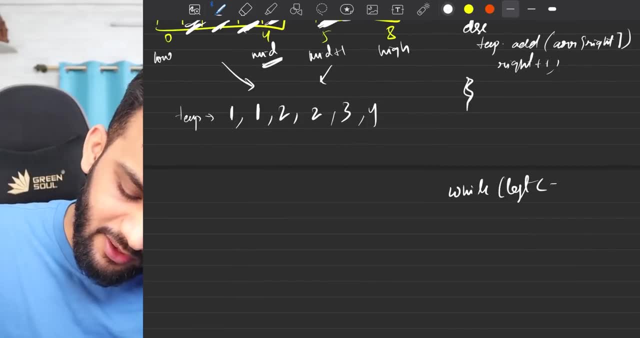 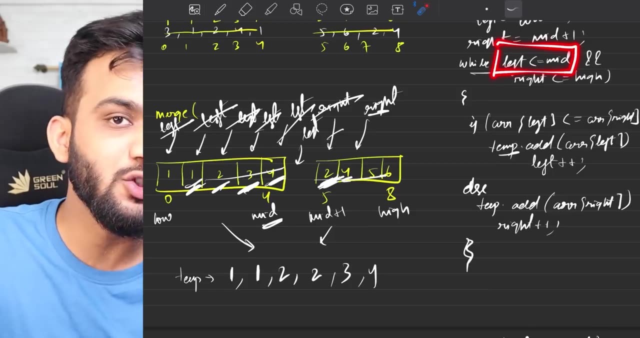 exceeded mid. there is no one on the left. so what i will say is after the end: if there is anyone on the left, which means if there is anyone on the left, because if this while, if this while loop is false, either it will be false because this is true or this is true. so if there are on 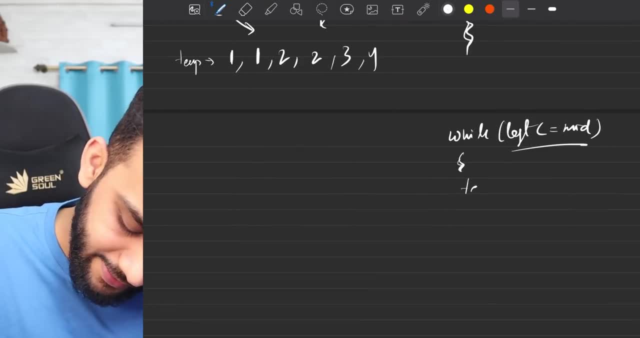 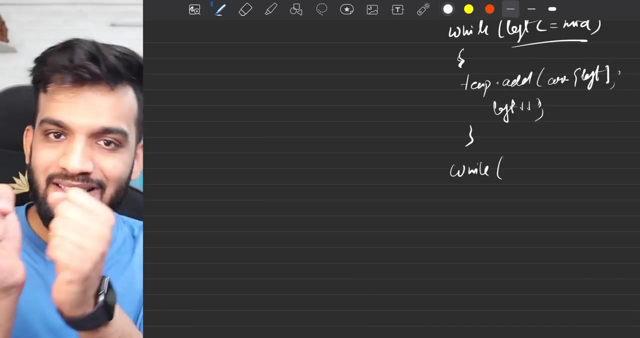 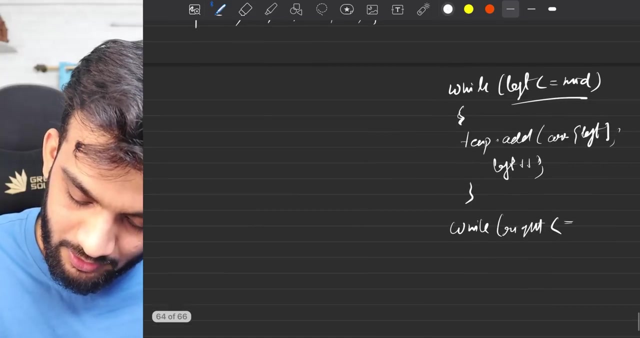 the left. if there are on the left, i will still add it. i'll just take everyone from the left and add it to my stuff. and if there are people on the right- because anyone will be true- either there will be on the left, either there will be on the right. if there are people on the right, which will be right high. 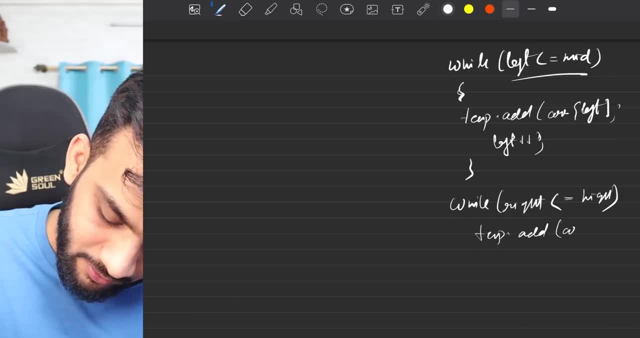 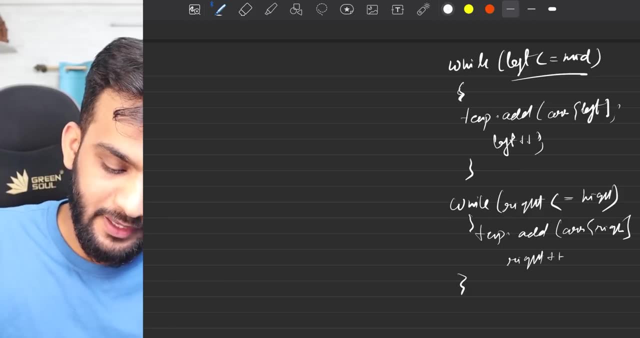 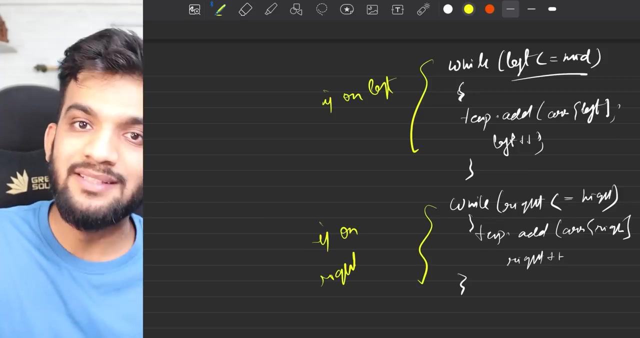 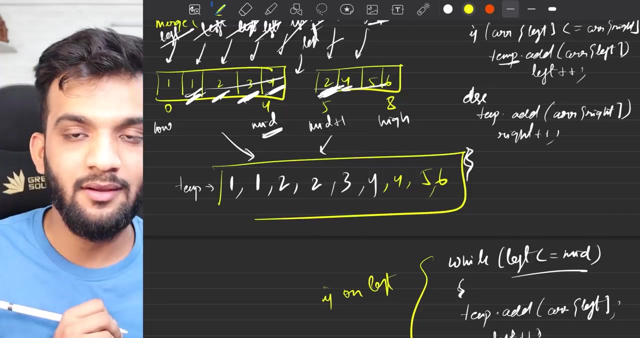 and then i'll say temporary dot, add array of right and i'll do right plus plus. quite simple, if that means: if on left, copy them. if on right, copy them. as simple as that. so can i say: at the end of the day i would have four, four, five, six, all of them in the temporary array. now we need to place them. 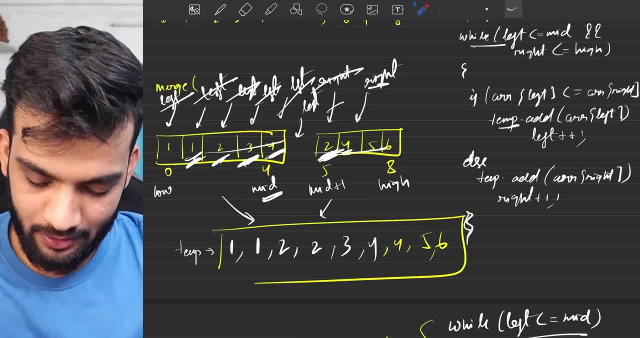 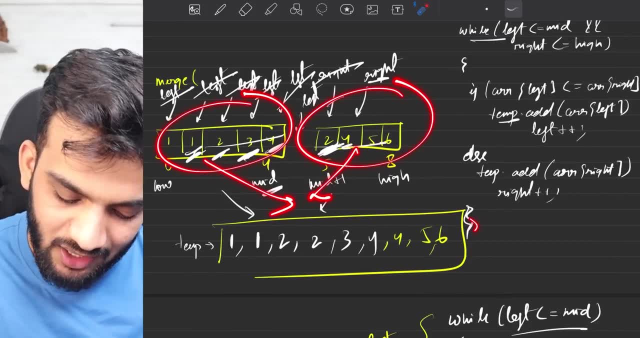 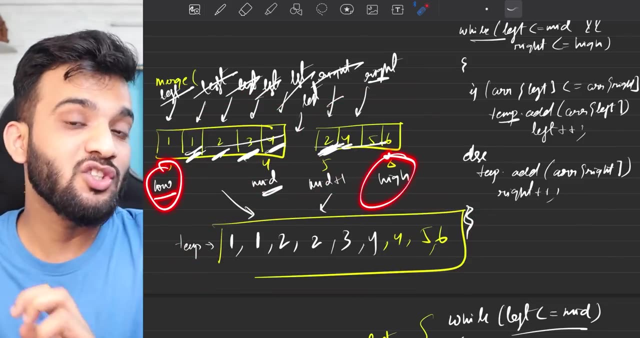 into the original array. so what have we completed till this step? we can say the left sorted array and the right sorted array have been put into a third array- temporary. but we actually need to put it from low to high, because that's the original array, because the original array is from 0 to 8. 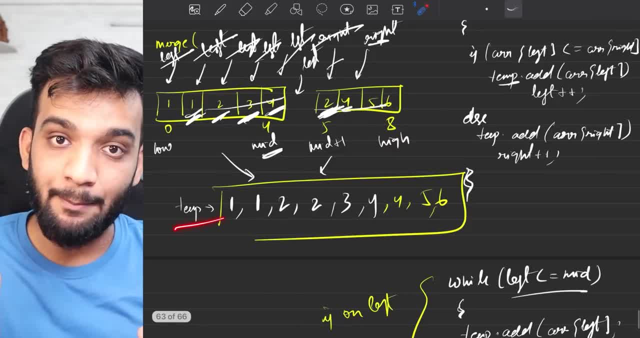 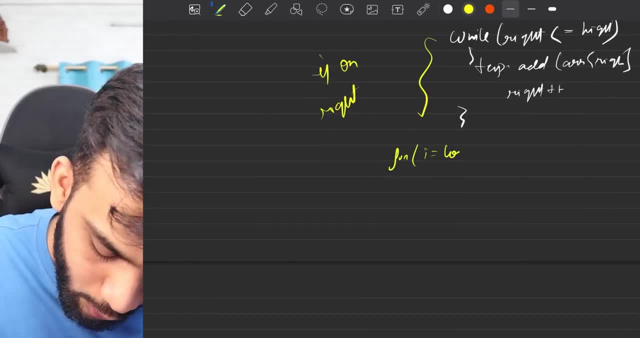 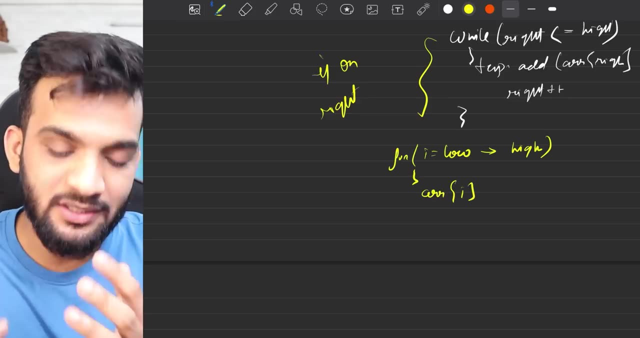 and we'll take these elements and put it there because it is in temporary. so what i'll do is i will probably loop. yes, let's loop. i'll say for i from low to high is where i'll loop. please loop from there. and i'll say: array of i. that means who is the first element? temporary. 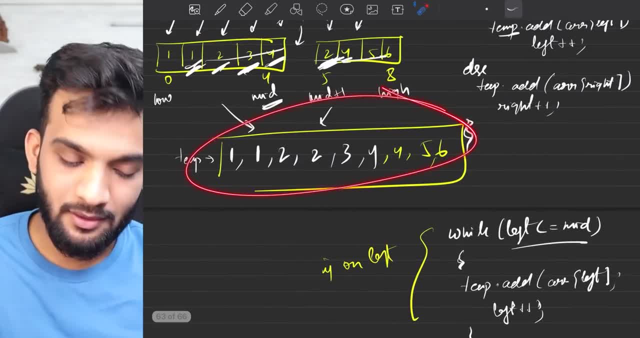 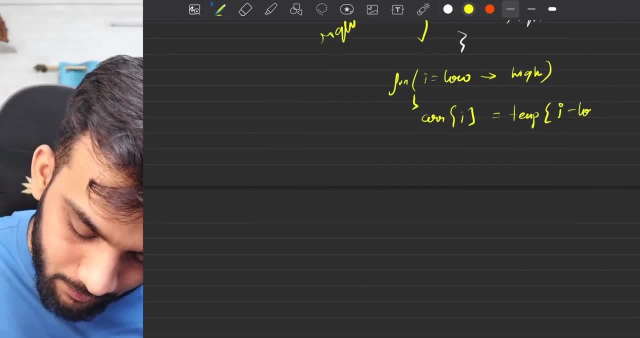 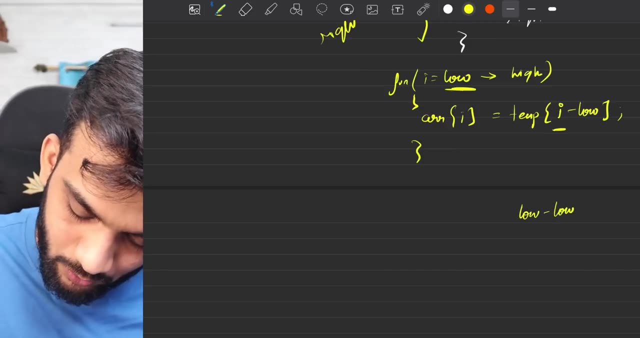 temporary must be keeping because it's a temporary array. it will always keep in the zeroth index. so i'll always say temporary, i minus low, that's it. first time i will be low. so what will this happen? low minus low, that will be zero. next time i will be. 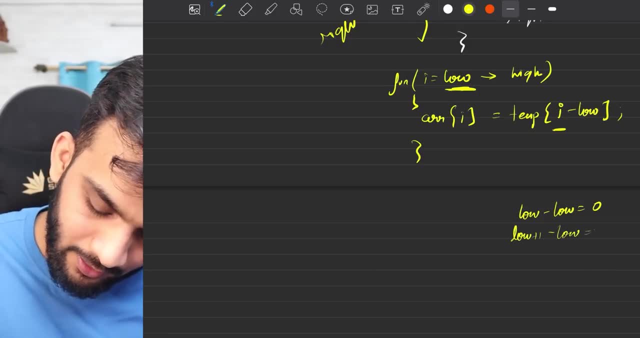 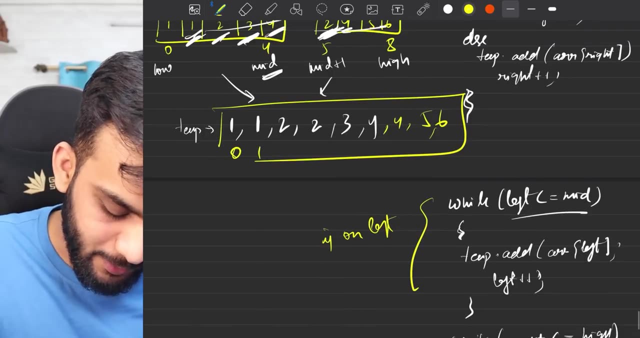 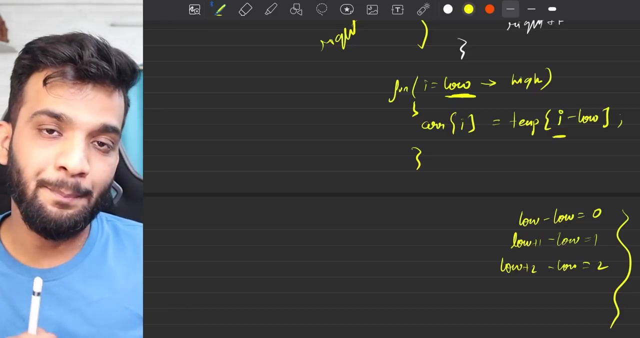 low plus one. so low plus one minus two, that'll be one. next time i will be low plus two. low plus two minus two, it'll be two. so it will get all these indexes because it will be stored in a temporary array. it will pick up all these indexes and store in the correct order. so we'll pick up all these. 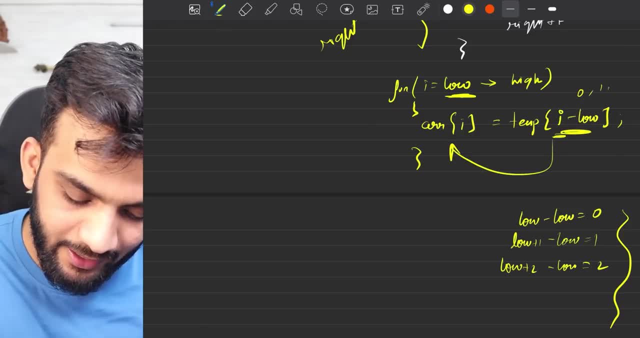 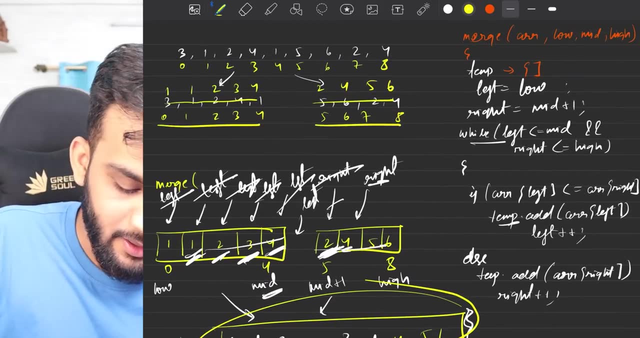 indexes at zero, one, two, and it'll store it in the correct order from low to high, because, because this was low to mid, this was mid plus one to high and they got together from low to high. that was the original array got it. this is how the merge. 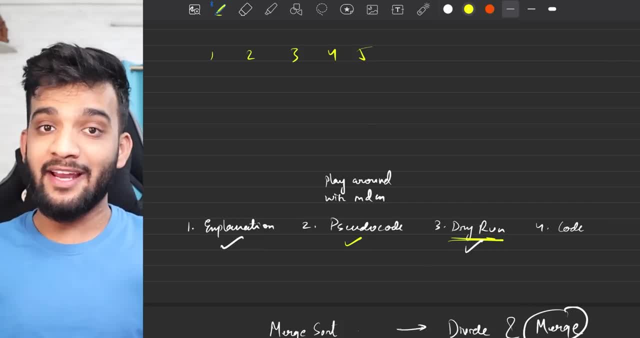 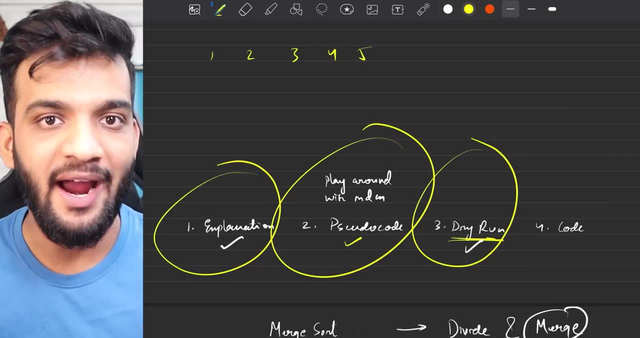 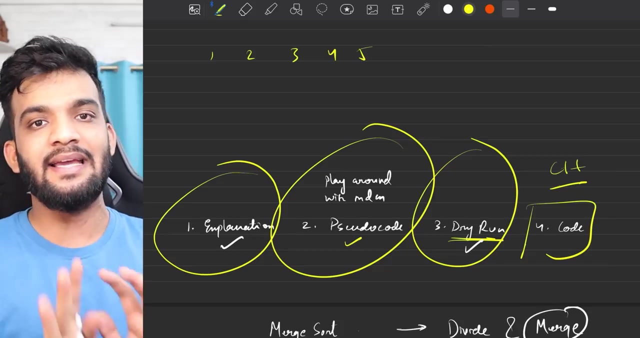 will look like. i hope that does make sense. so now i can confidently say that you have understood the, the pseudo code and the dry run. So you can code it in C++, Java and Python. So I'll just go across and code it in C++, but the Java and Python codes you can find them in the links in the description. 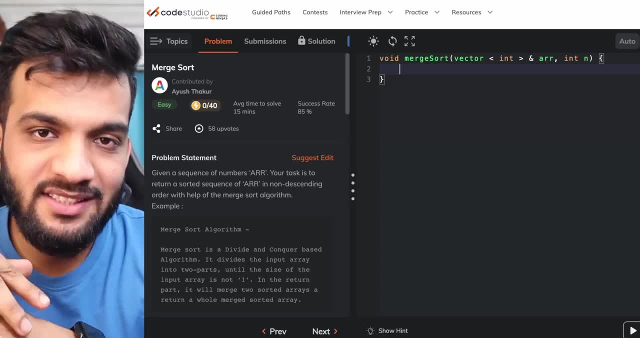 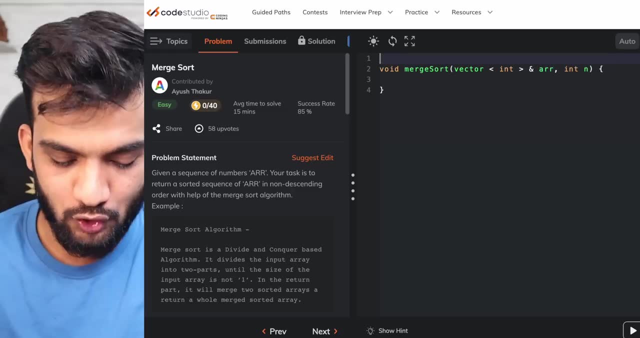 It will be updated very, very soon. just in case it is not there as of now, Let's come to the compiler and try to code it. So we are given a function, we are given the array and we are given this. So assume we are going to write this function and we say void mouse short and I'll say let's. 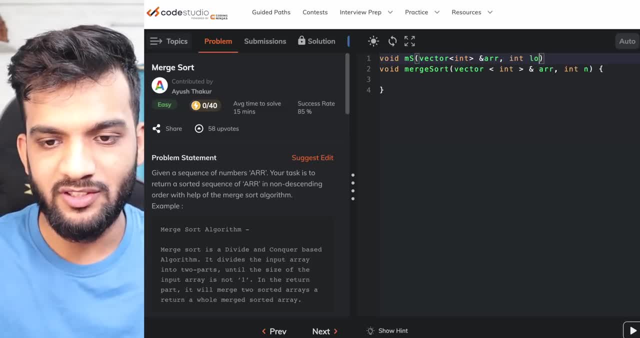 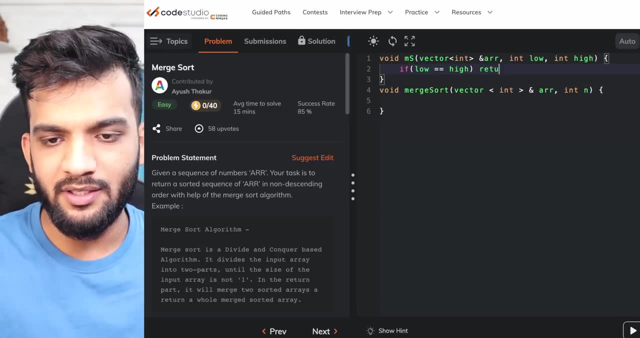 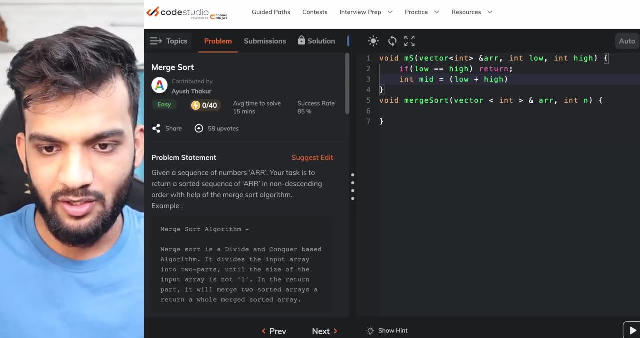 take the array, which is this: please make sure you pass it by reference. low and high. That's what we require, And we know one thing: if low is equal to equal to high, we are going to return. that's it. Otherwise, we are going to find a middle which is low plus high by two, And then we will. 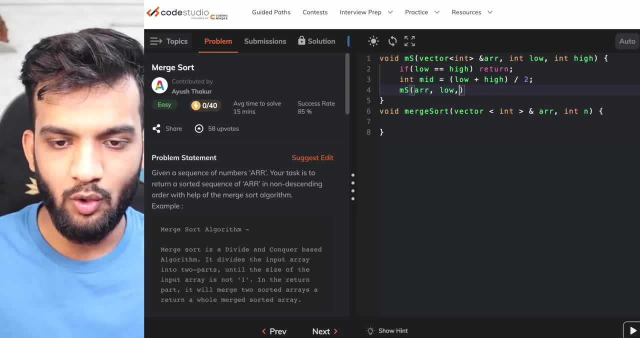 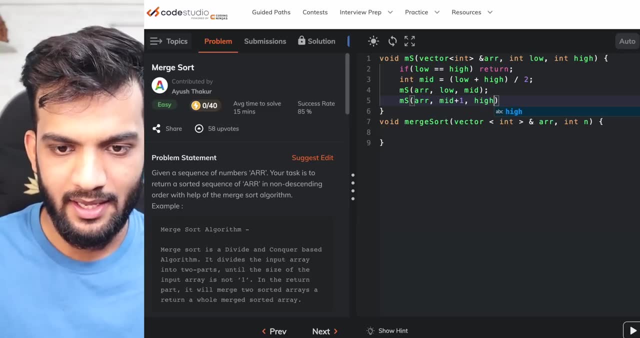 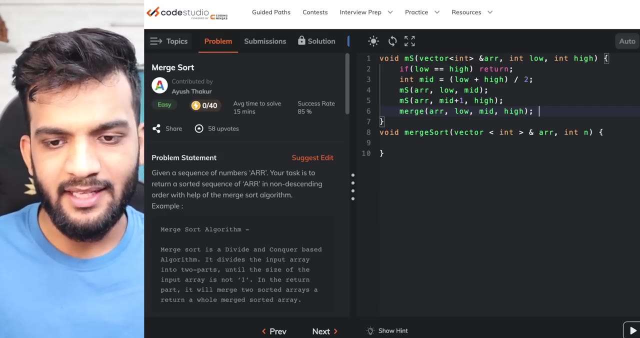 be calling the MS with array comma low, comma mid and MS array comma mid plus one comma high, and then we will be calling something like merge where we'll be passing array low, mid and high. That's what the algorithm will be, And we can call MS with the array and zero comma n minus one. 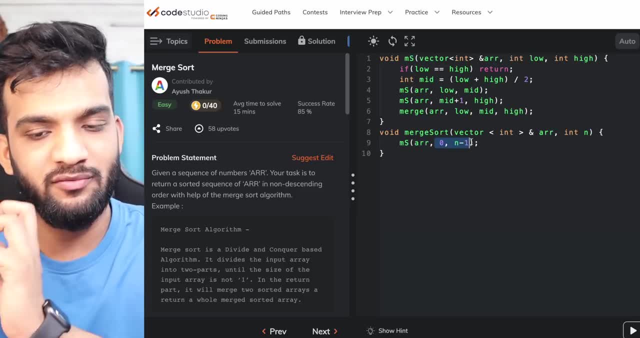 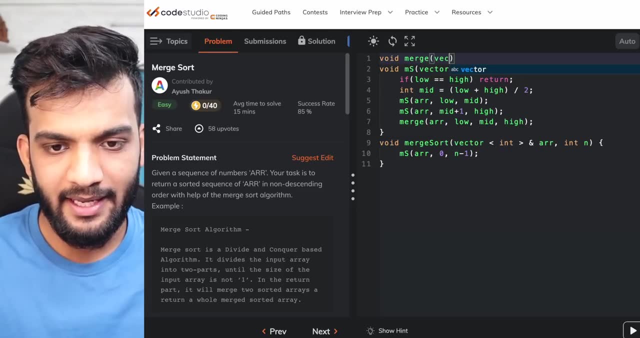 because that's the initial starting and the end position of the entire array. Just have to write the merge function and I think we will be done. So let's write the void merge And again, make sure you take everything by reference array and then low, and then you can say merge and then 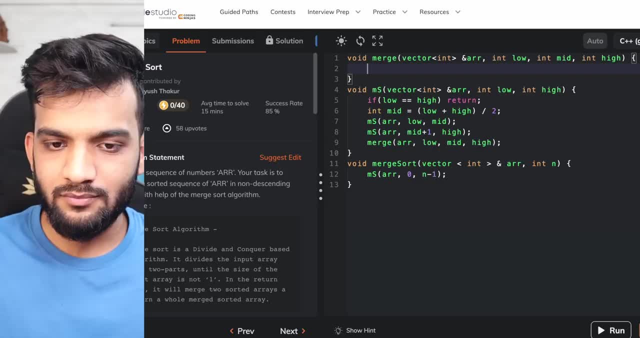 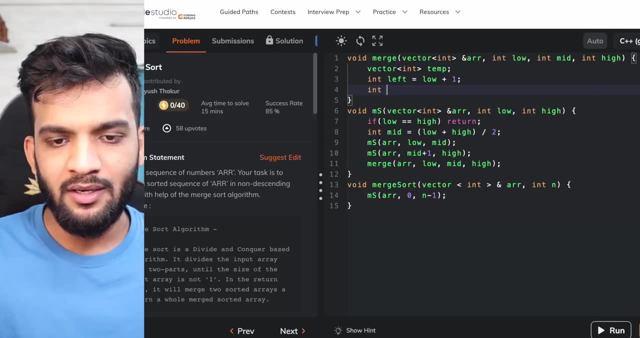 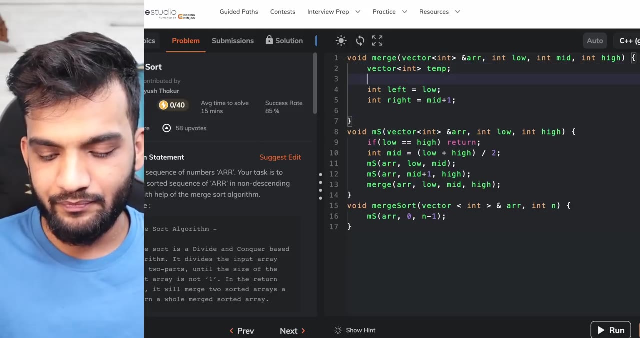 mid, and then you can take high. So can I just take a temporary array? We can, And we can take the left pointer to be low plus one- sorry, low rather- And we can take the right pointer to be mid plus one, because we know the first array will be like. if I have to comment it, it will be from: 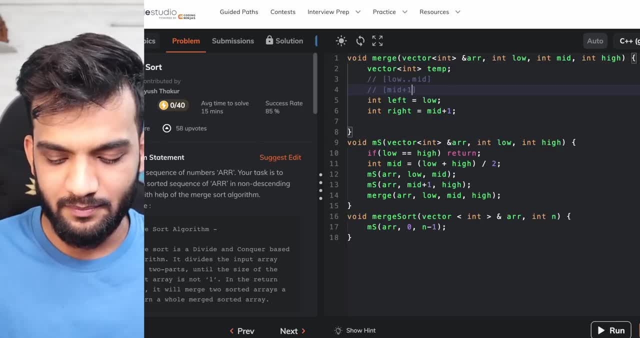 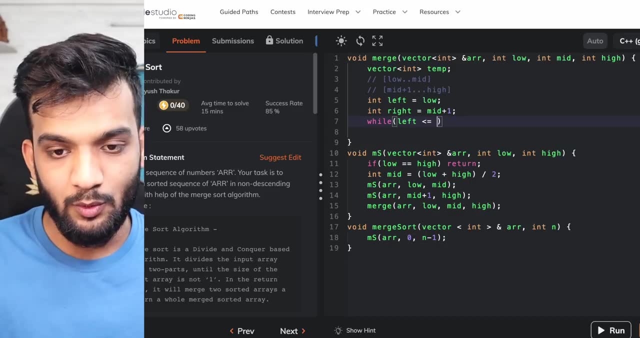 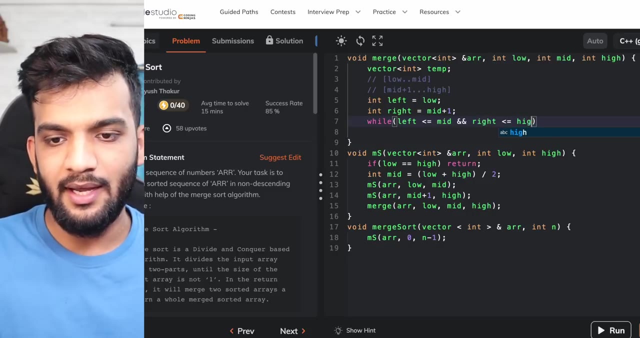 low to mid And the second array, if you remember it, will be mid plus one till high. So let's see, let's write this, So we say left is less than equal to mid and and mid, and then right is less than equal to high. Very simple. 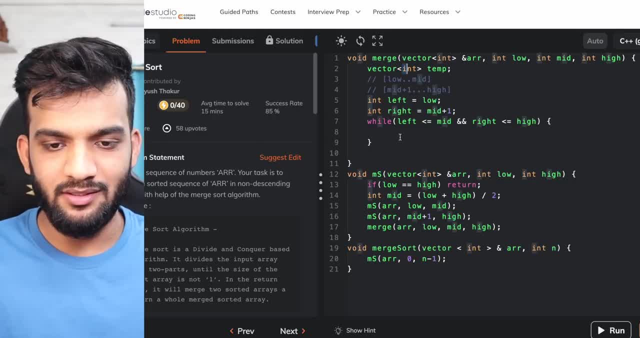 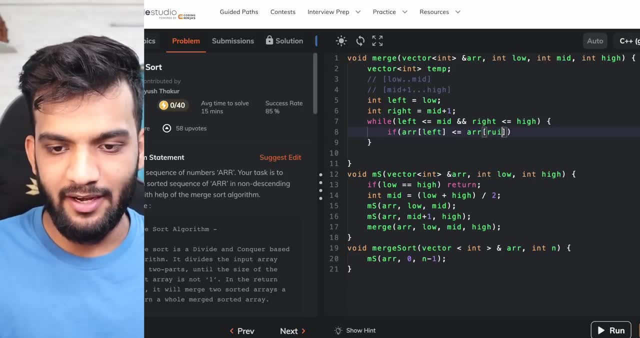 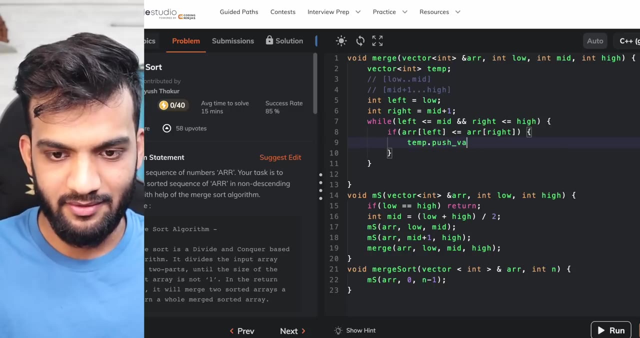 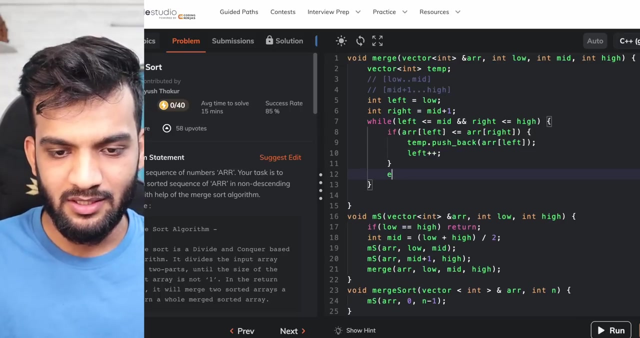 But we need a temporary array that is defined over here. We say, hey, array of left, are you smaller than array of right? If you are, can you please go ahead and get attached, push back to array of left? Very simple. At the same time, you can do a left plus plus and you can write an else and you can. 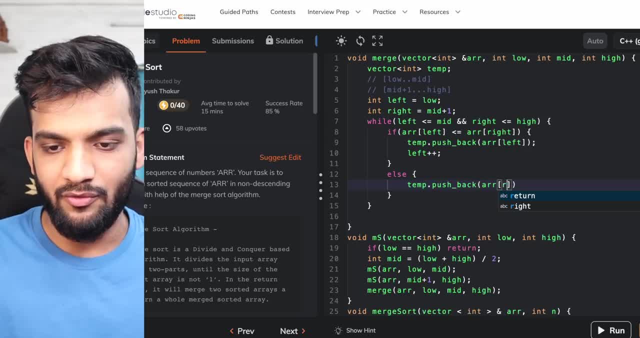 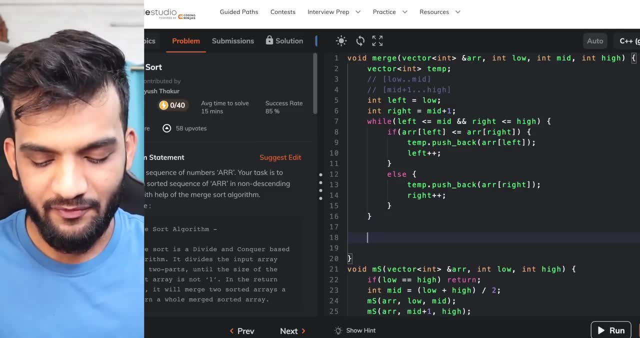 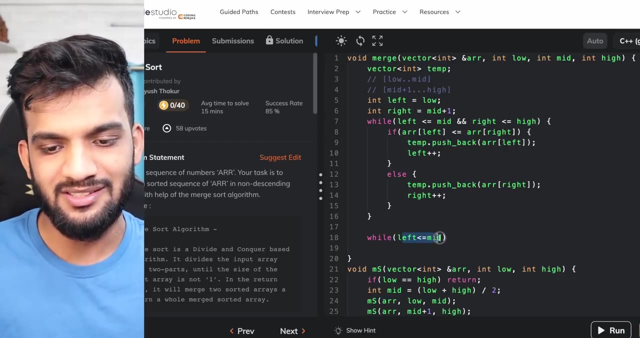 say temporary dot, push back array of right and you can say right plus plus. This is what you will do for comparing and putting it After that, if there are still elements left on the left, please take it, because if this is false, then this must be having some elements on the left, So go ahead. 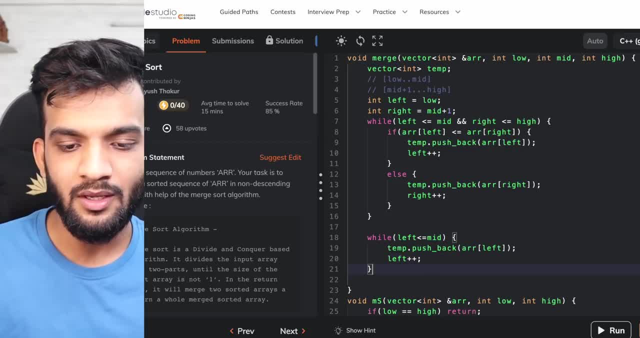 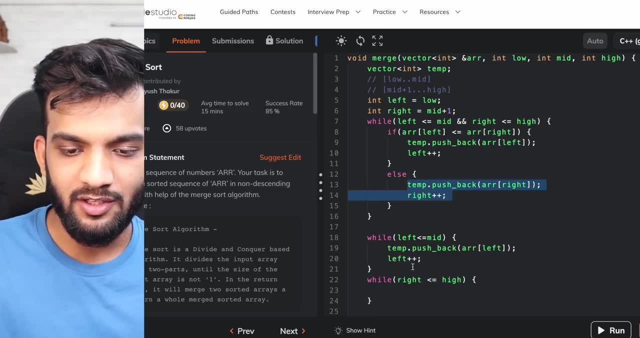 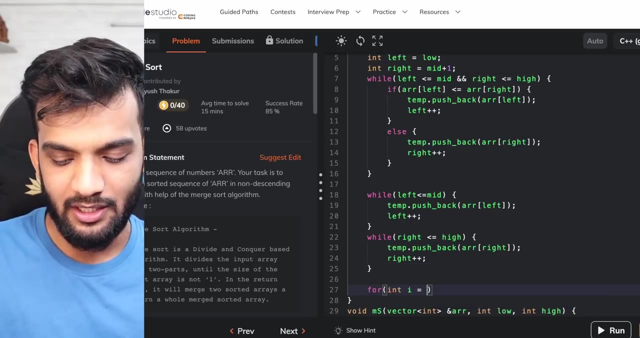 and just copy paste this, Perfect. And if there are still elements on the right, then go ahead and copy paste everything from the right. quite simple. Once you have done this, make sure you put them into the array, which is for int: i equal to low. i less than equal to. 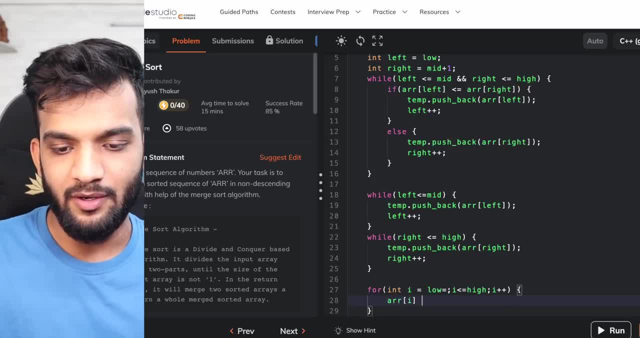 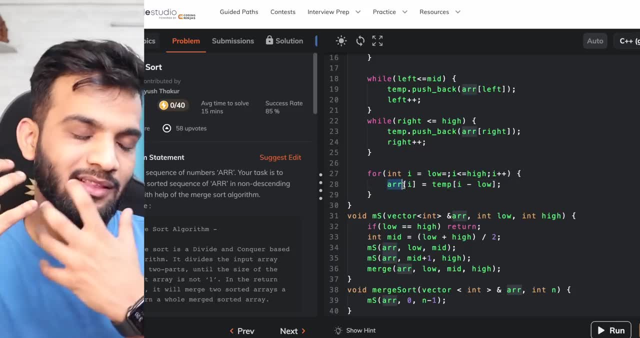 high and i plus plus, and you can say: array of i will be temporary, of i minus low. So once you've done this, since everything is by reference, the numbers will rearrange themselves in the array itself. now i can go ahead and go ahead and run this and see if it is running. 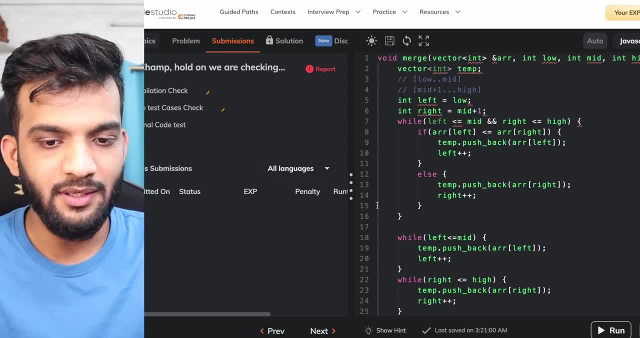 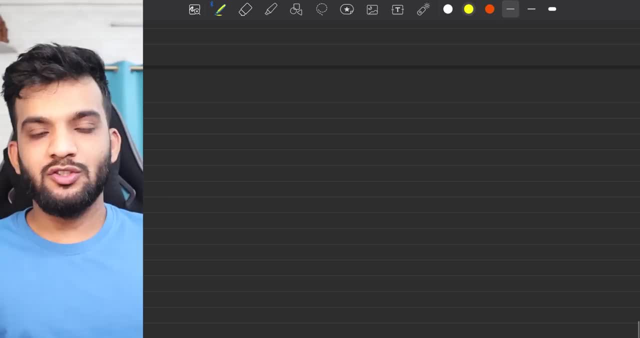 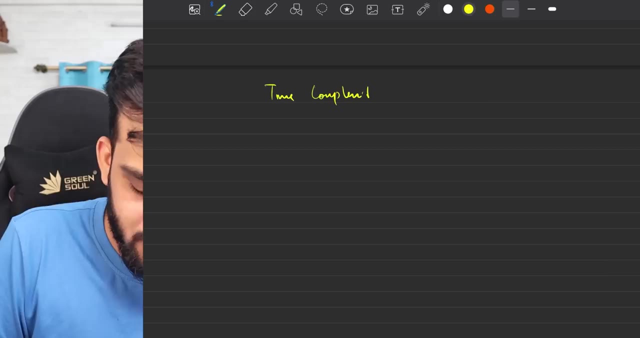 fine, i hope it does. it does, and now i'll quickly submit this. i write codes in one go, wow nice, no syntax errors. so we have understood everything, but there's only one thing that is left, which is the time complexity of this merge shot algorithm. remember one thing: what's happening? there's an. 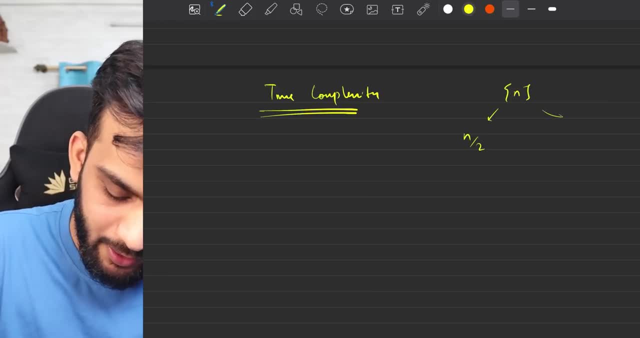 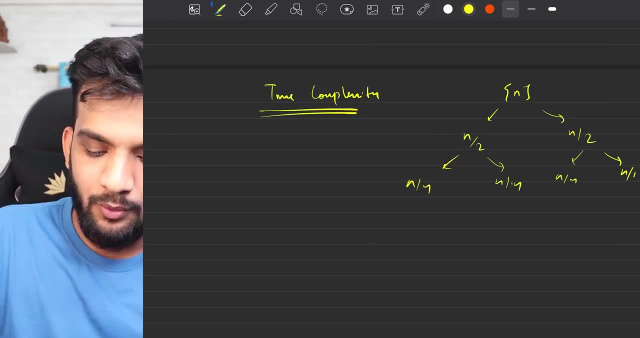 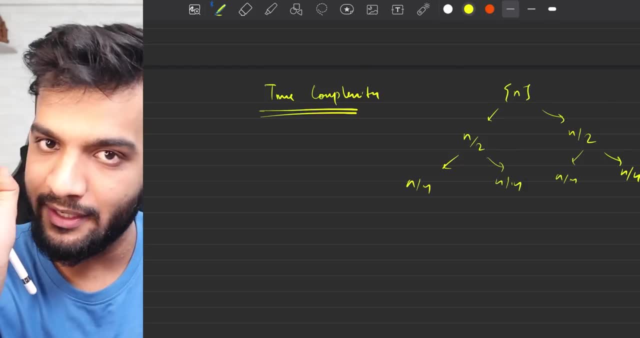 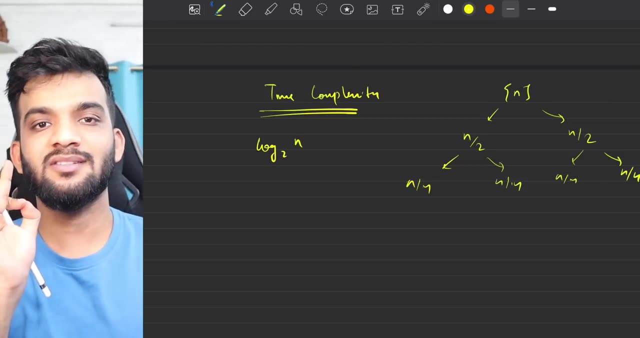 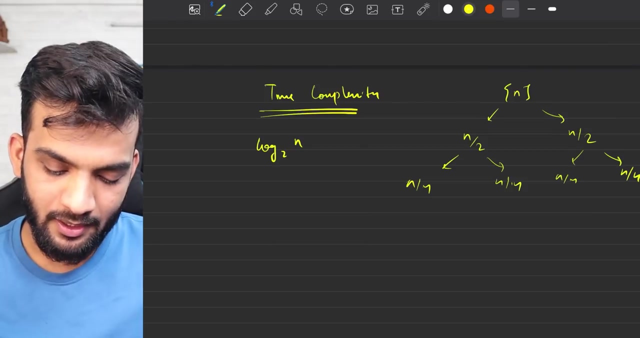 and if you remember the time complexity lecture i have already told, whenever it gets divided by by 2, the time complexity is log b to n. remember this. now you might ask me, but trevor, why you're dividing by 2, it by by two, by two, but why it has log base 20. it's very simple: if i have to write 16 and i have 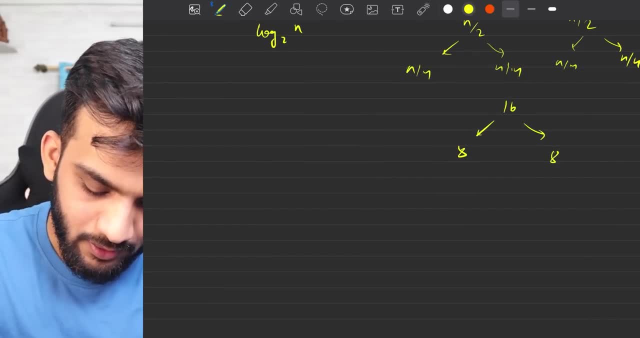 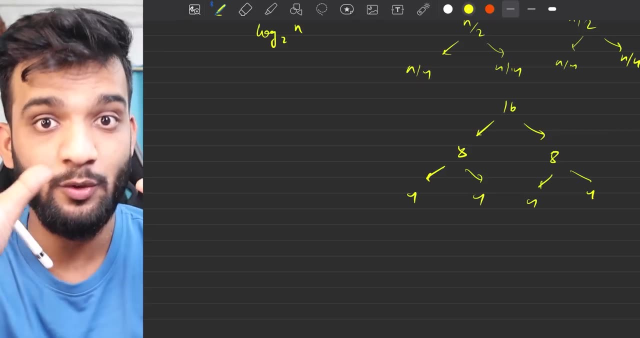 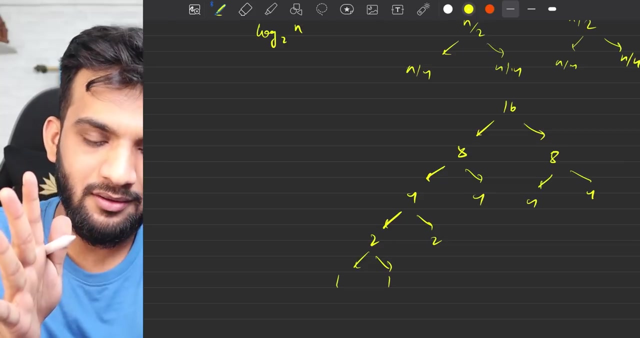 to divide it by two, it'll be like eight and eight. it'll be like four and four. right, like if there are four, like if there are 16. array elements gets divided into eight and eight. it gets divided into four and four, four gets into two and two, and then two gets into one and one. so apparently this is. 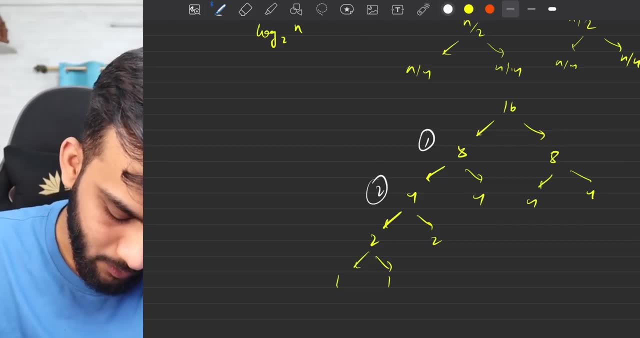 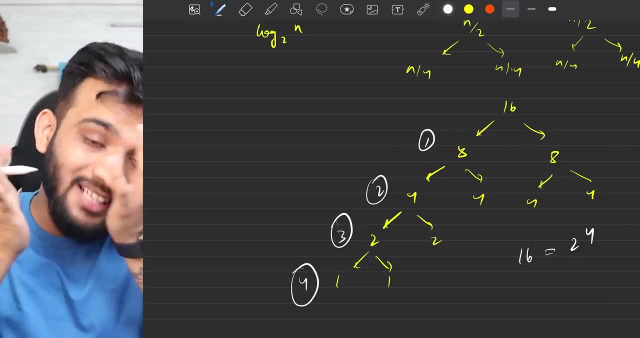 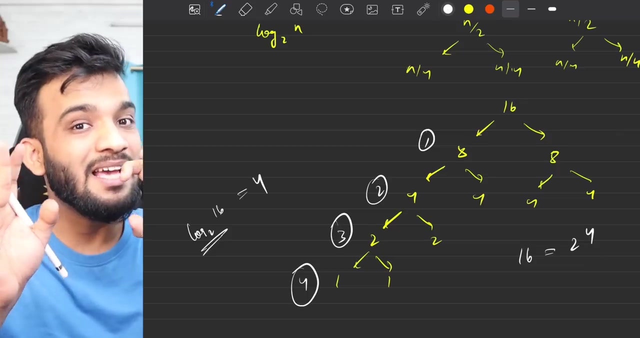 nothing but one step, two step, three step, four step, and 16 is nothing but two to the power of four, and that's nothing but four steps. right, four steps. log base to 16 is nothing but four steps. so it's approximately logarithmic number of times the division happens. it's approximately. 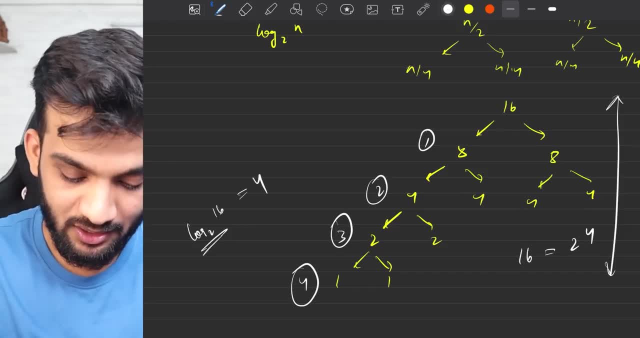 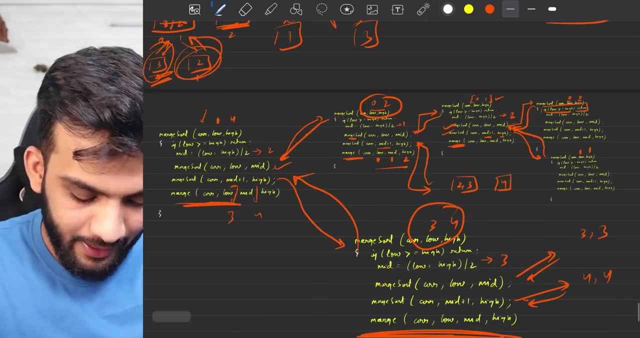 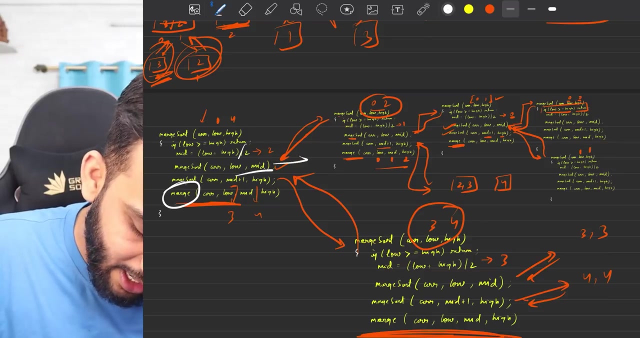 logarithmic number of times that the division happens. that means it gets broken down into logarithmic of n time, and you're also performing something like a merge every time. so every time division by like this is: this is half and this is half, so this half will go on till. 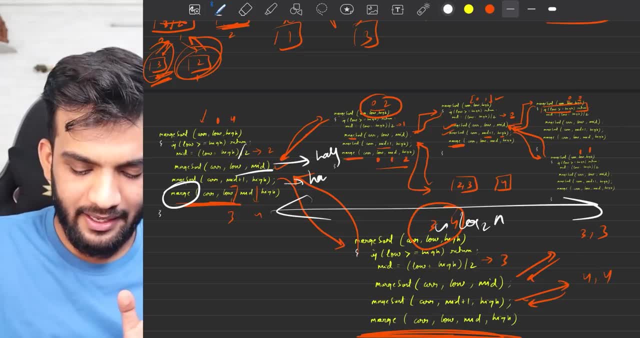 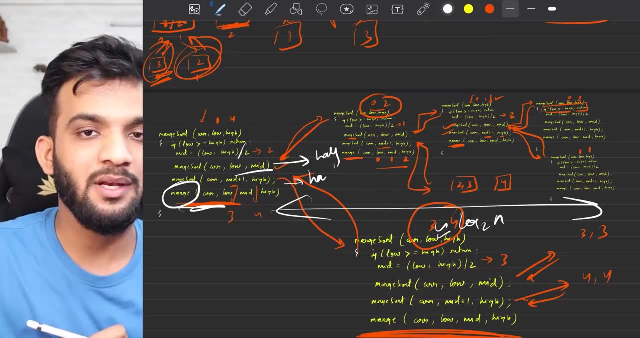 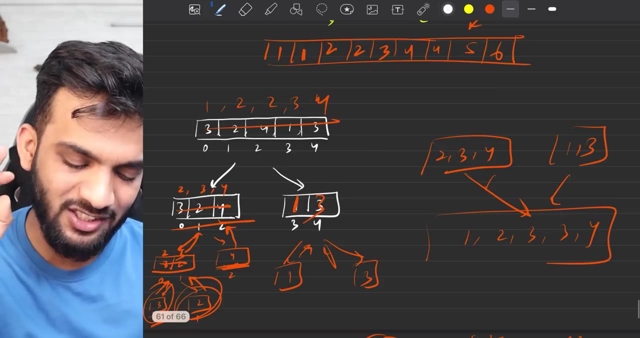 log base to n. near about. again. everything is in terms of near about. okay. time complexities goes till near about. log base to n and then there is a merge happening. how much is merge taking? if i have to think of the extremist case? if i have to think of the extremist case, 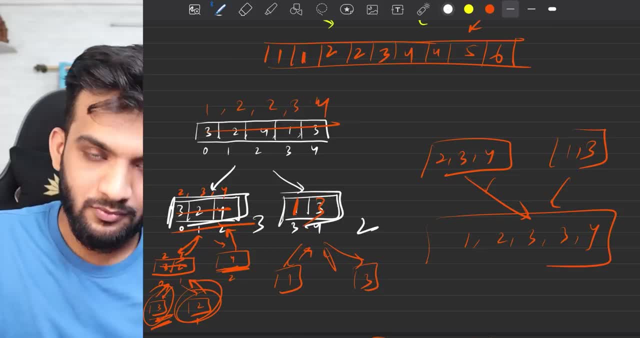 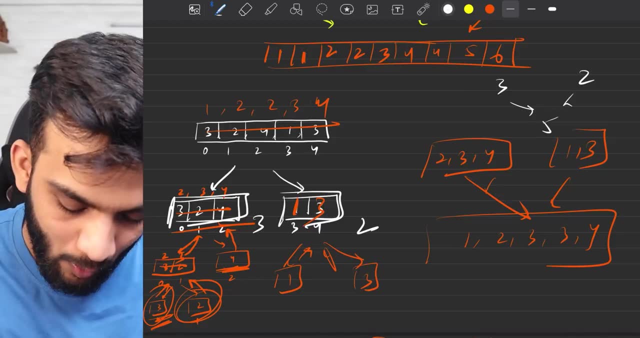 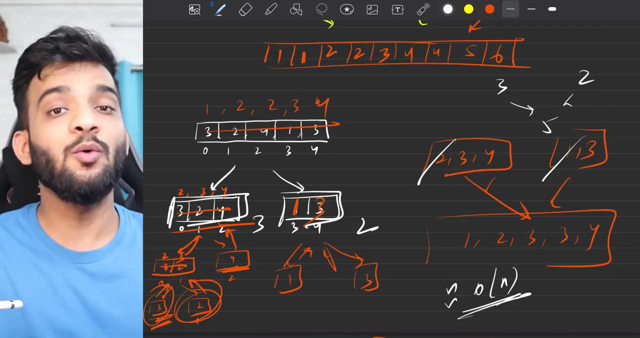 can i say: this is of size three, this is of size two. so in order to merge three and two elements, i'm gonna require five steps at minimum. one comparison. that's like everyone is comparing in itself. it's like a near about bigo of n. that's the worst case, because for this i'll end up taking 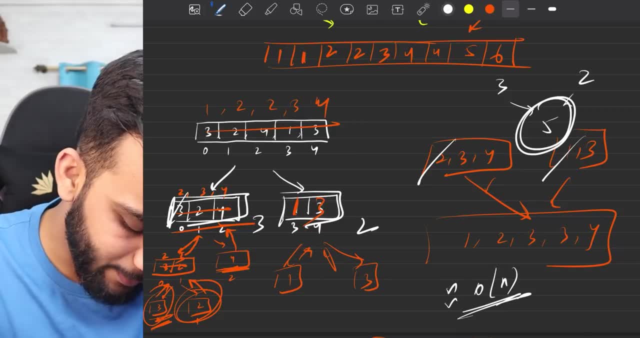 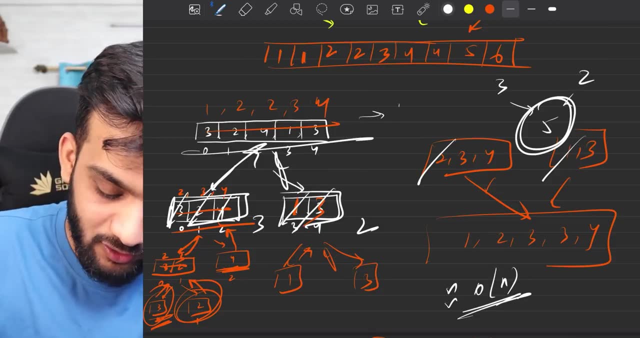 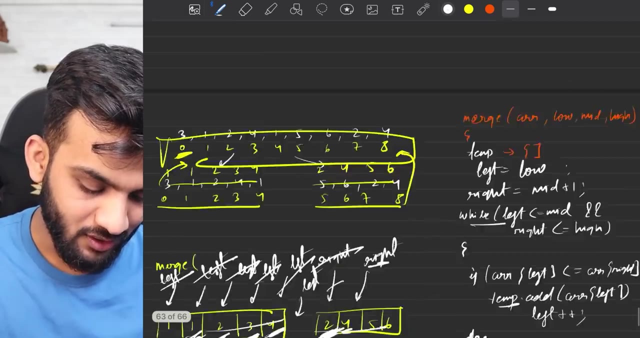 at minimum of five steps, because every element is compared one by one and then it is put over here. it takes minimum of five steps, which is nothing but the length of the array at the worst case. so can i say the merge? i have to go back to this. uh, there's so many things written, man, i have to go back this. can i say this at the 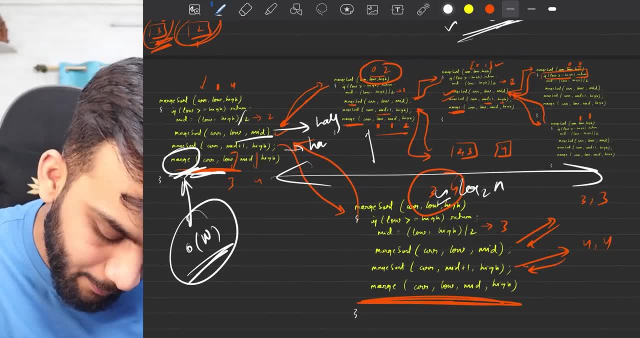 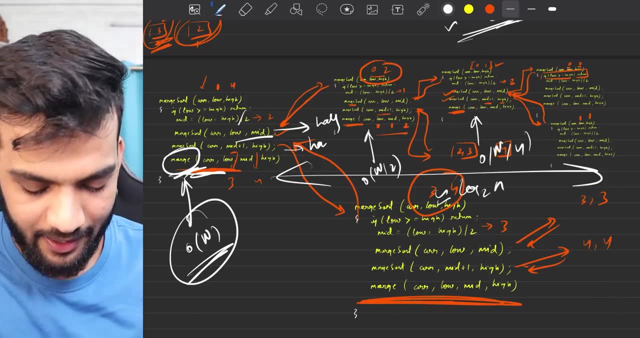 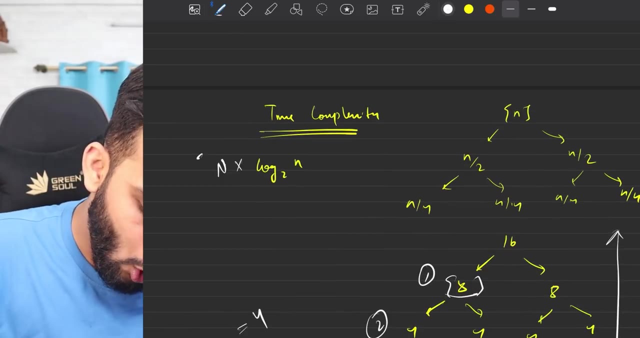 worst case takes bigo of n this time. over here it might take bigo of n by two. over here it might take n by four, something like this. but at the worst case it is taking n. so thereby i can actually say that the time complexity is nothing but n. into log base to n. now you might. 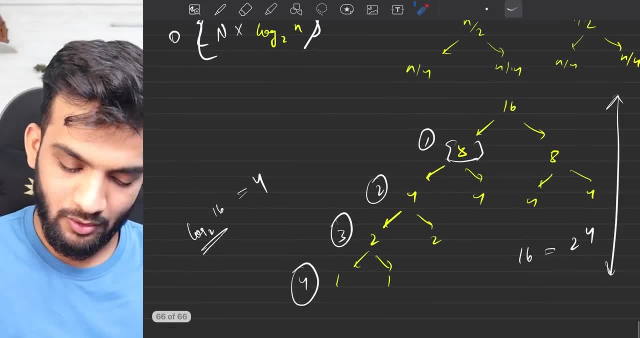 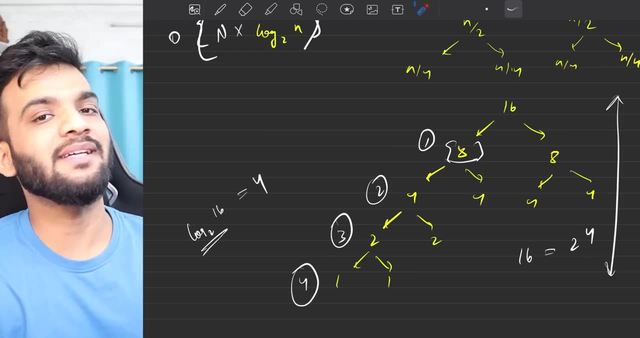 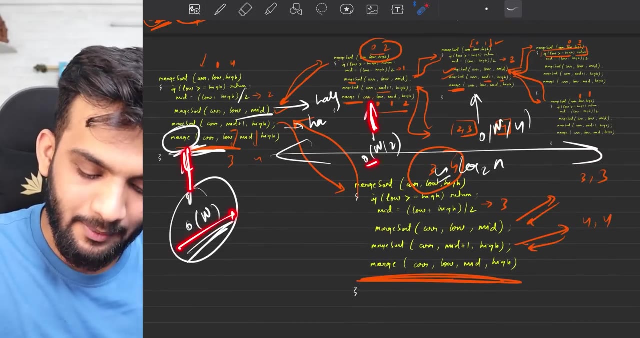 ask me a question, but striver, wait. one step, two step, three step, four step. who will be counting these steps? wait, that is actually compensated how? because the merge over here takes bigo of n. the merge over here takes n by two. the merge over here will take n by four. the merge is taking less. 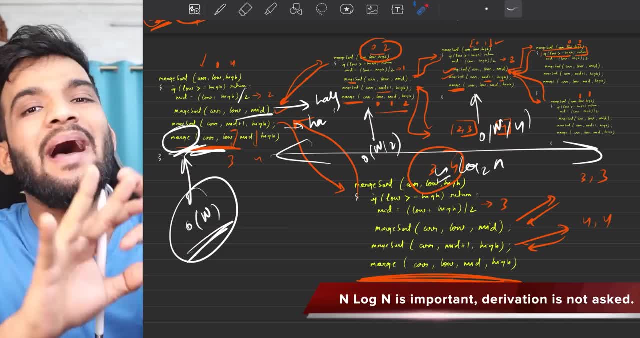 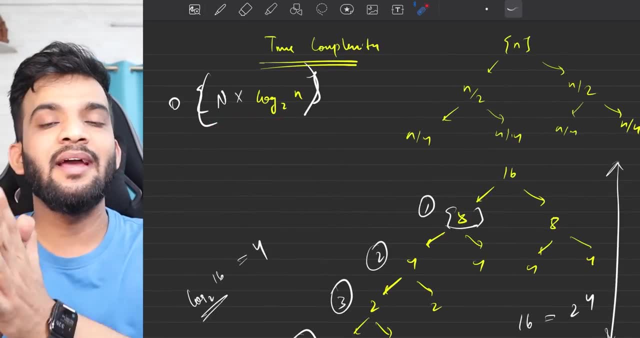 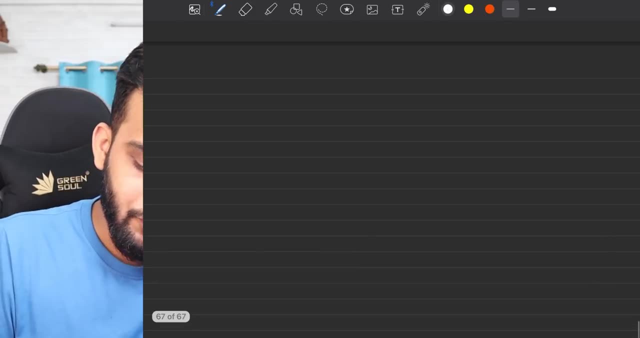 so in overall, if you try to add it up in mathematical you will actually get somewhere near about n into log base to n, as the merge starts time complex. so n log n is the best average and the worst case. but if i have to ask, hey, what is the space complexity of the algorithm? 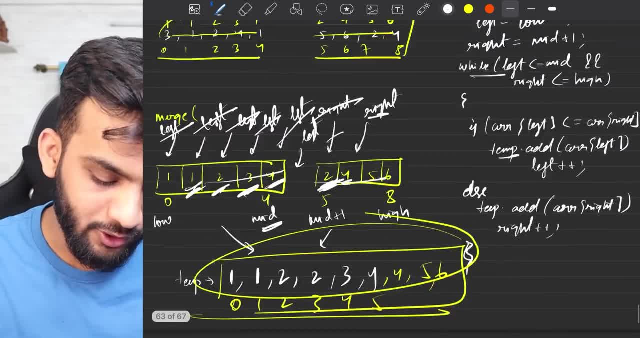 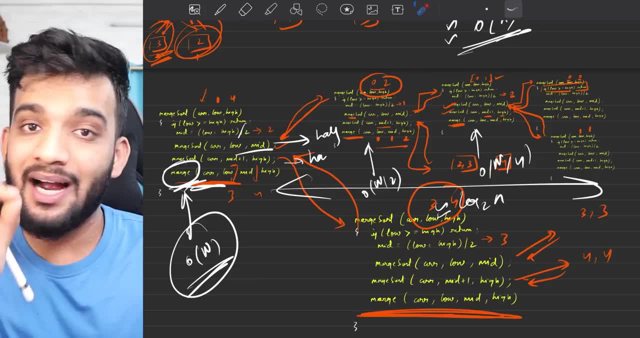 how much extra space are we using? so, if you remember the algorithm, the algorithm is actually using indexes, no separate arrays. is this the given array that they are using or is this the given array that they are using? are they using any extra additional space? they are during merge. 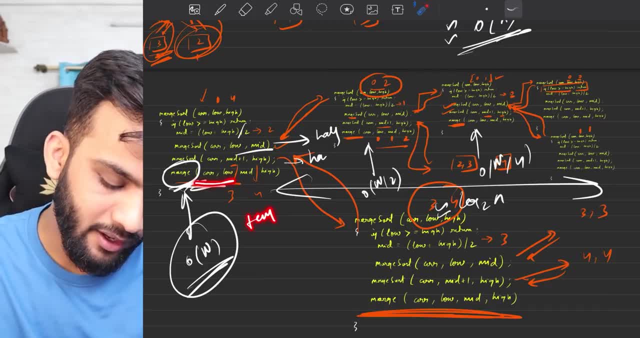 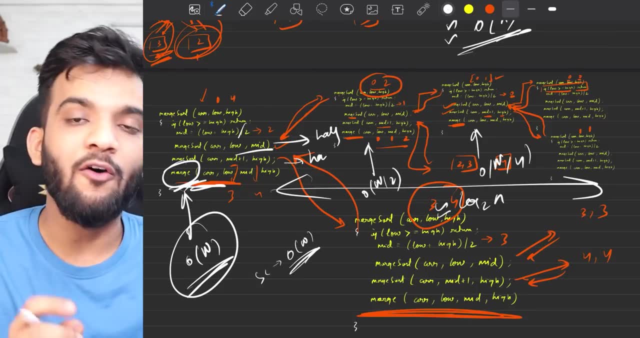 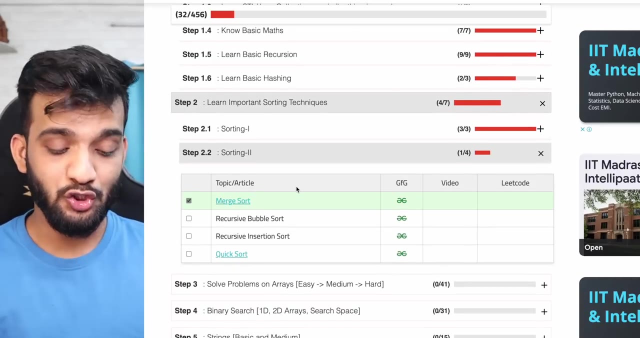 in every merge step they're creating a temporary array which at the worst case might take bigo of n. so the space complexity at the worst case is bigo of n, near about bigo of n, for this particular algorithm. so with this i will be completing merge shot and the time is 3: 28 am in the morning as 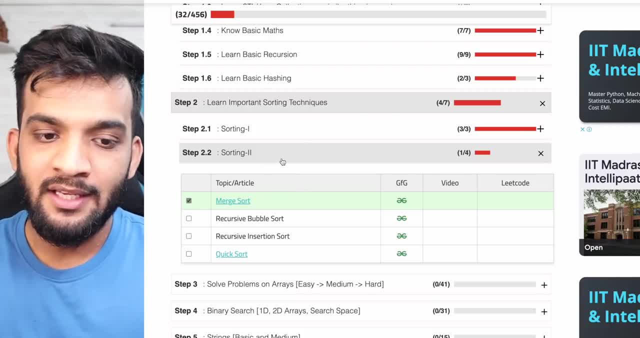 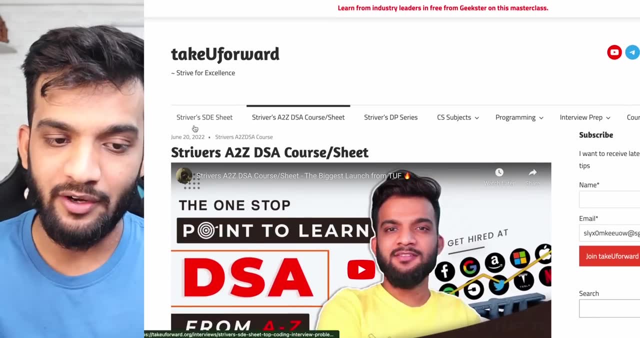 you can see, i cannot record in the day because there's a lot of background noise. so just in case you understood everything, please, please, consider hitting that like button. and if you haven't checked out strivers, it was a dsa course. the link will be in the description. 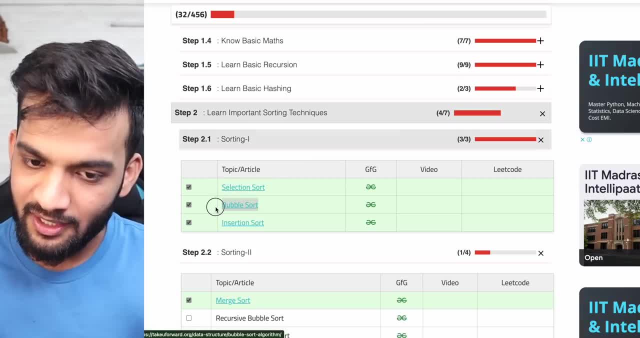 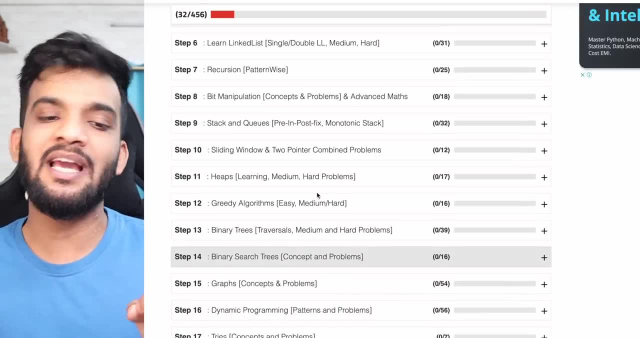 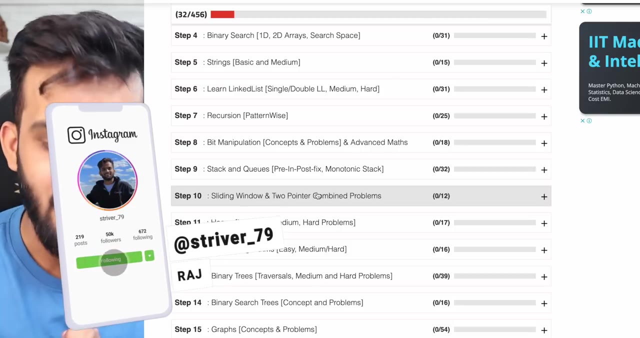 please make sure you check it out, because we have notes for everything. we will be attaching video solutions to everything. yes, most of the advanced topics have been covered previously. i am starting to cover the basic topics now, so you can definitely proceed ahead with the advanced topics in case you need for advanced as well. so, guys, if you're new to our channel, please do. 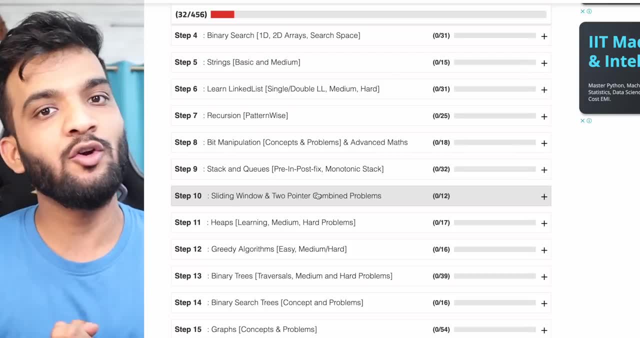 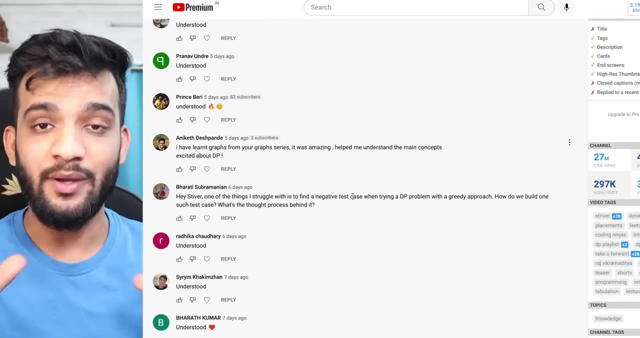 consider hitting that subscribe button and i will see you in the next video. bye, bye, subscribe button, because that is the only thing that keeps you motivated to make these kind of videos. and, yeah, to follow our tradition, please make sure your comment understood in the comments so that i get a vibe that you guys are understanding everything. so with this i'll be wrapping up this. 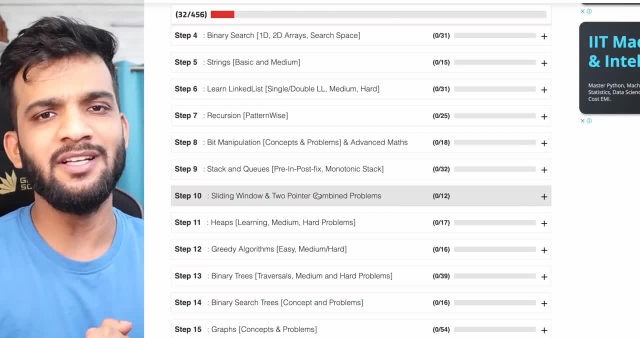 video. if you haven't followed me on instagram, twitter, linkedin, the links will be in the description. with this, let's wrap up this video and meet in some other video.